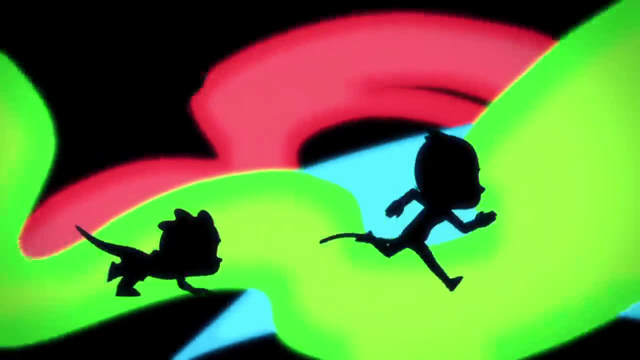 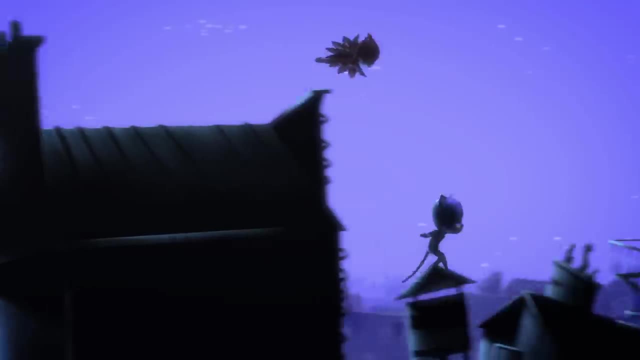 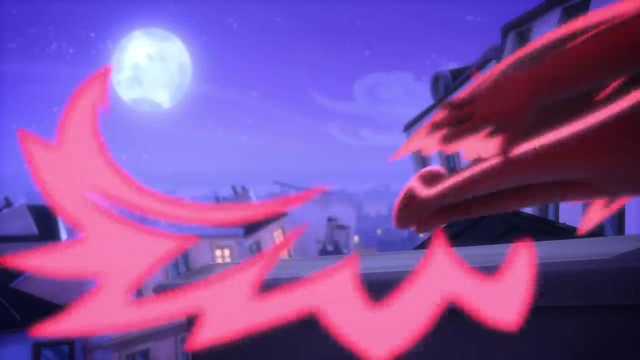 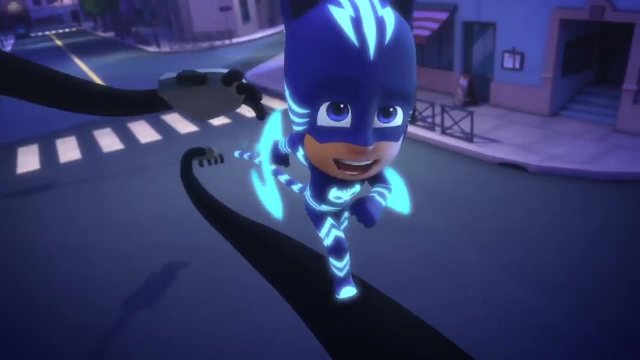 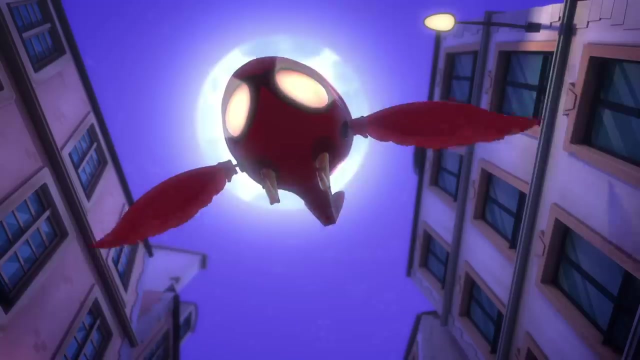 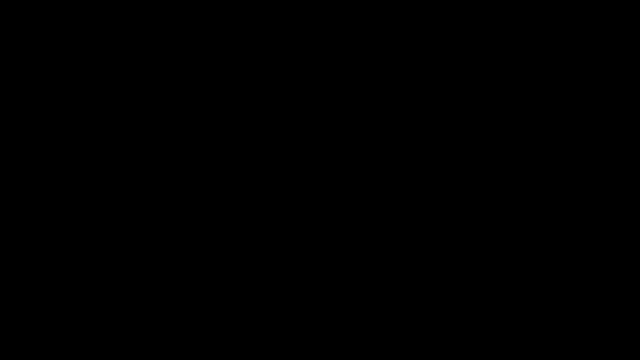 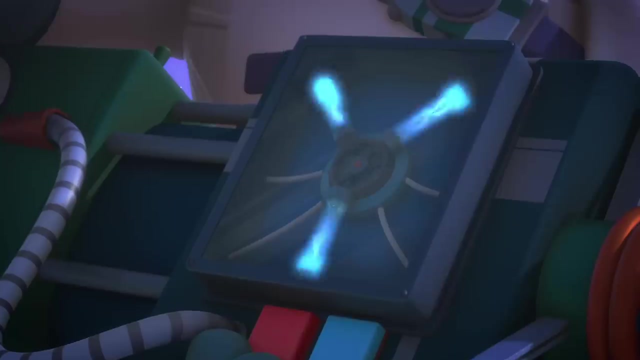 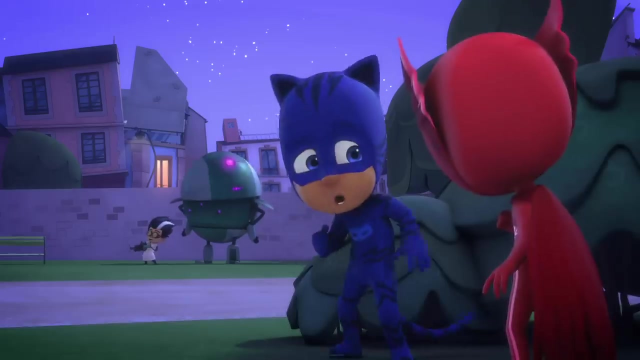 Captions are auto-generated by YouTube. PJ Masks, PJ Masks. We're the PJ Masks, PJ Masks- Catboy Squared. And now for some target practice with my multiplying machine. Romeo and a multiplying machine. 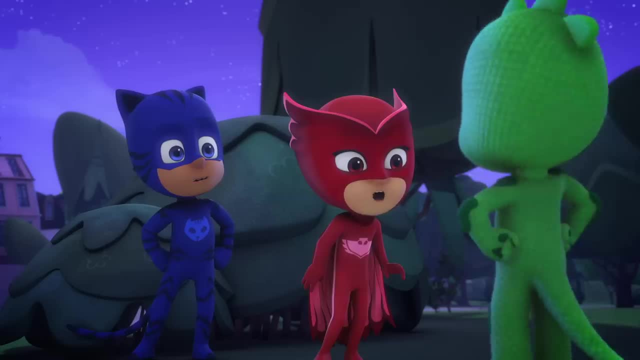 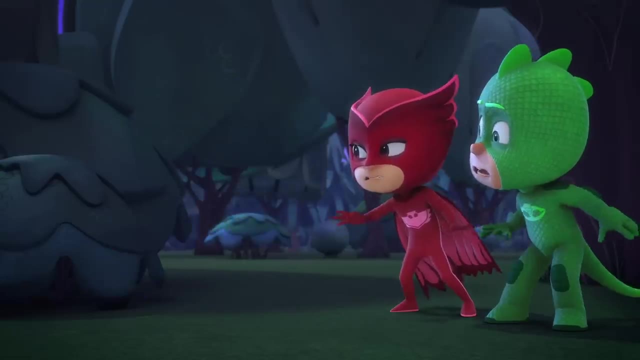 I'll use my super camouflage to sneak up and take it. Then you throw it to me and I'll pass it to Catboy. And ooh, I've got a better idea. I'll grab it right now, Super Cat, What? 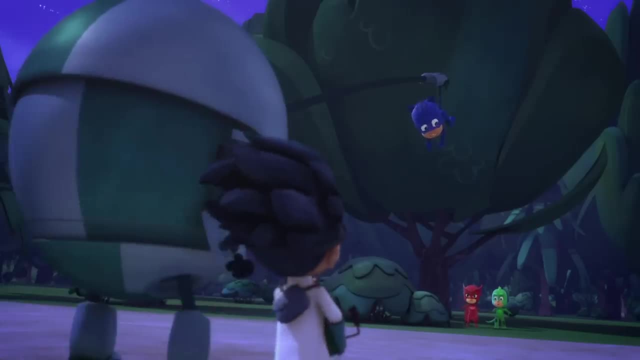 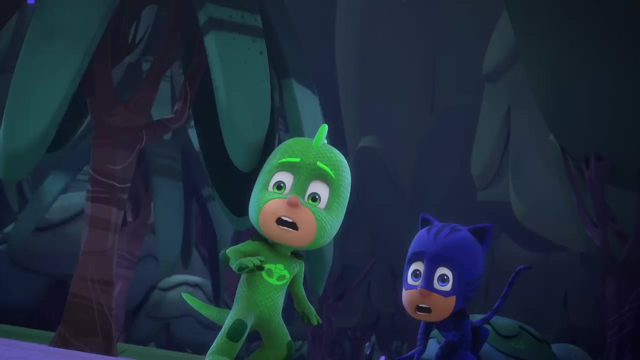 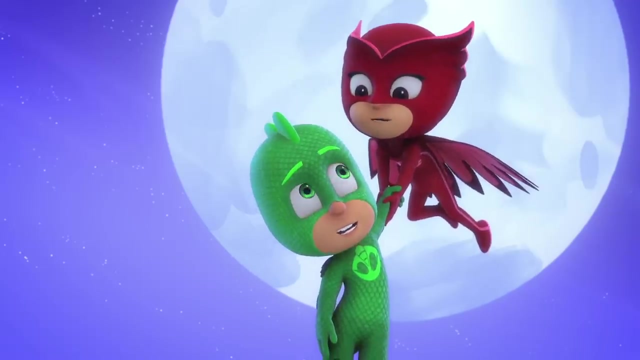 Uh-oh, Catboy having fun up there. pussycat, Put him down. robot, Super Gecko Muscle, You're barking up the wrong tree. Try these. Let's do things together. this time. I'll fight Gecko out first and then. 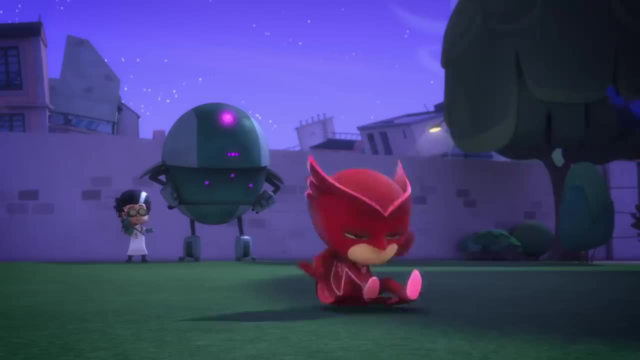 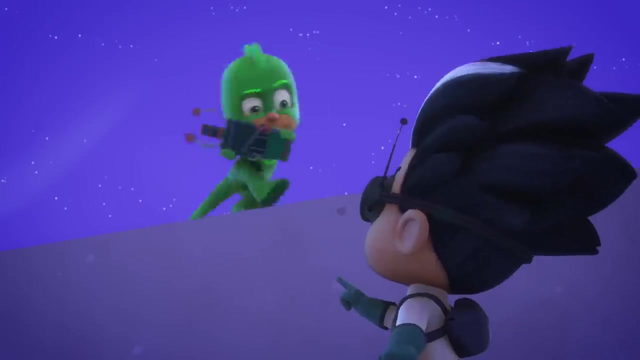 Wait, How about a super cat jump? Super Gecko Camouflage- Whoa, Give that back. Wait, What are you doing? Stop it. Super Gecko Muscle- No, You'll pay for this next time. PJ Masks. Now, let's lock this machine up in HQ. 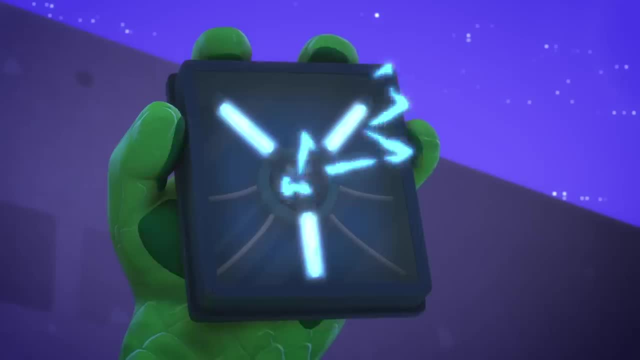 PJ Masks. I'll shout hooray, Because in the night you save the day. Get it PJ Masks. I'm so happy, I'm so happy, You're so happy, I'm so happy, You're so happy. 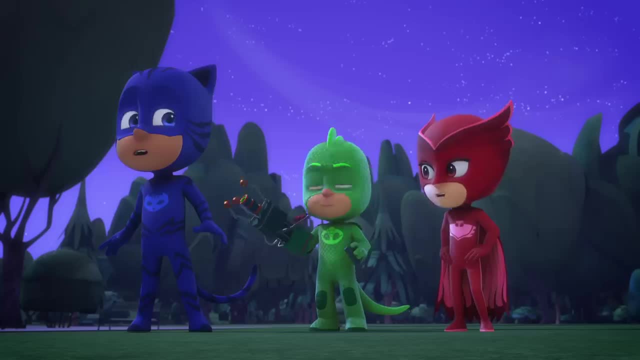 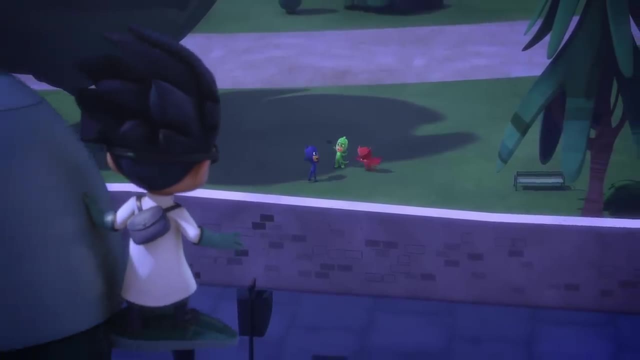 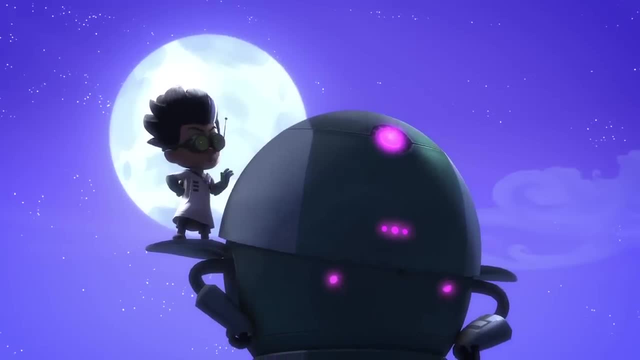 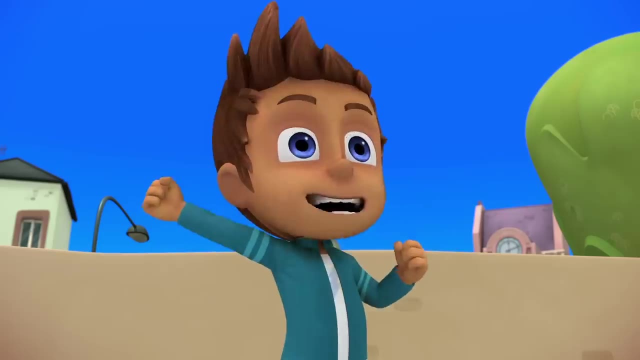 I'm so happy. I'm so happy To my robot friend. the PJ Mask saved the day. Getting rid of a multiplying machine isn't that easy, is it, my robot friend? Wahahahahaha, The PJ Mask saved the day. 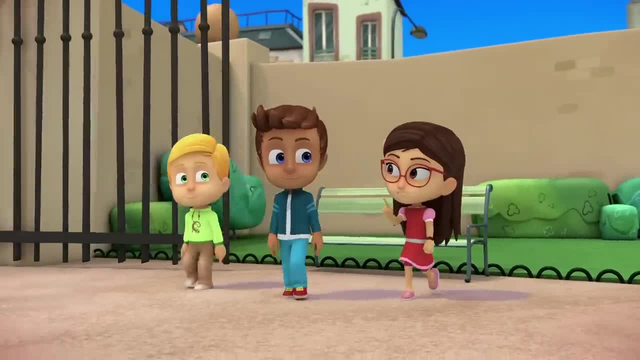 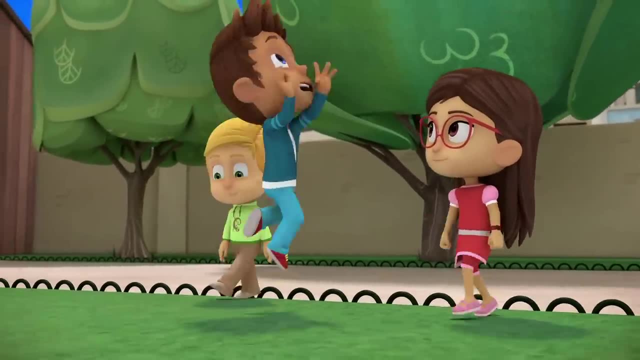 Again, It was pretty close, though One of us was always doing his own thing. I'm sorry, I just wanted us to win And we did. right Now, what are we going to play? Basketball, Volleyball? Actually, let's make it soccer. 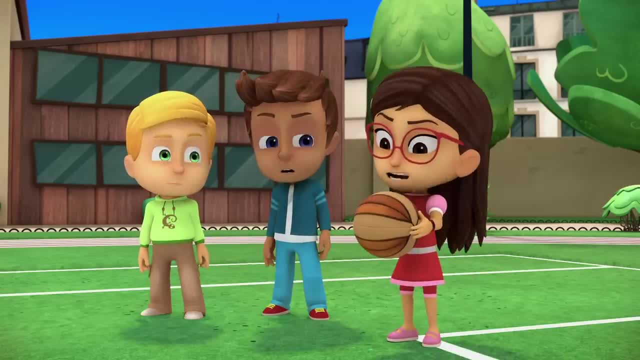 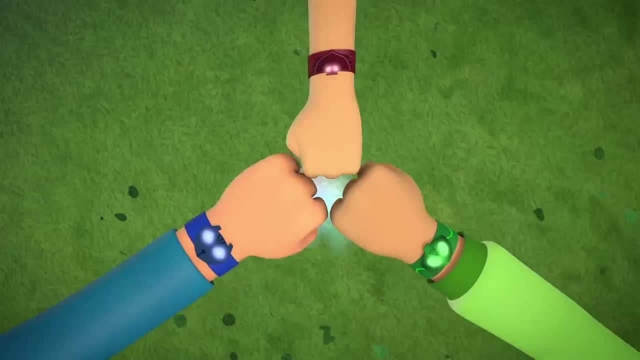 Look at all of these. Romeo must be practicing multiplying again. But how? The machine's back in HQ. Let's check it out. PJ Masks, we're on our way Into the night to save the day, Night in the city. 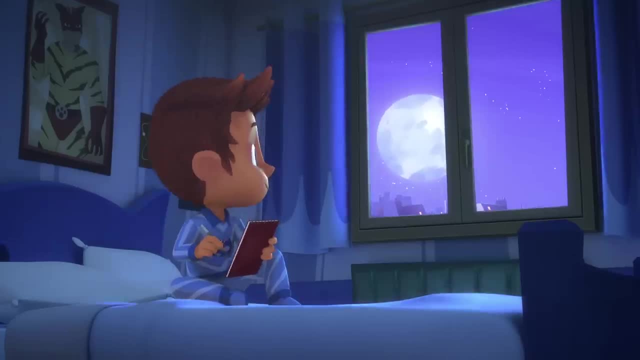 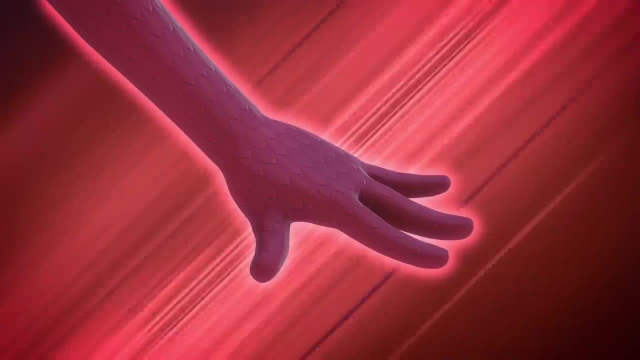 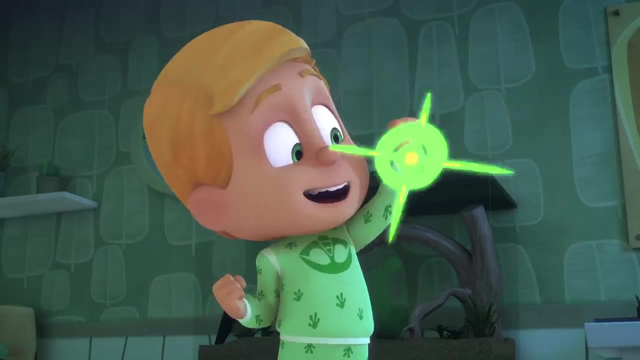 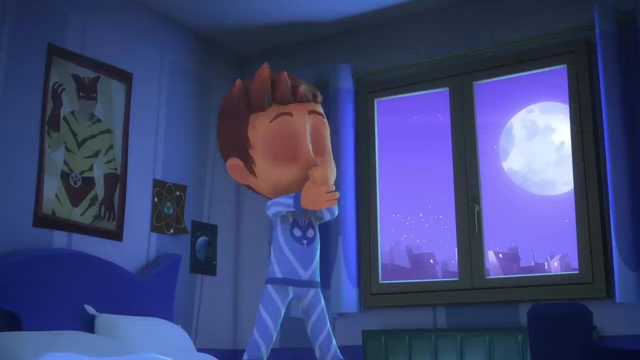 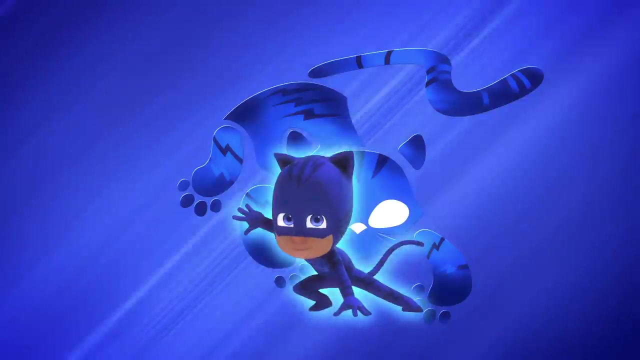 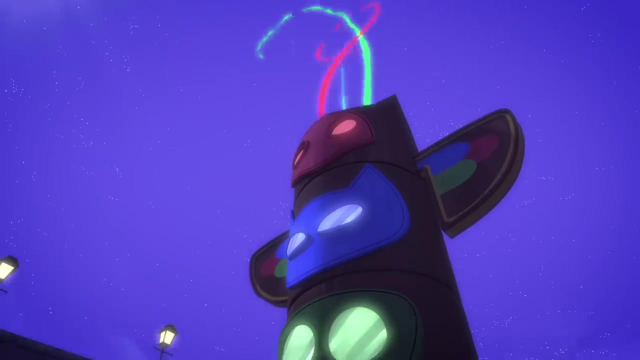 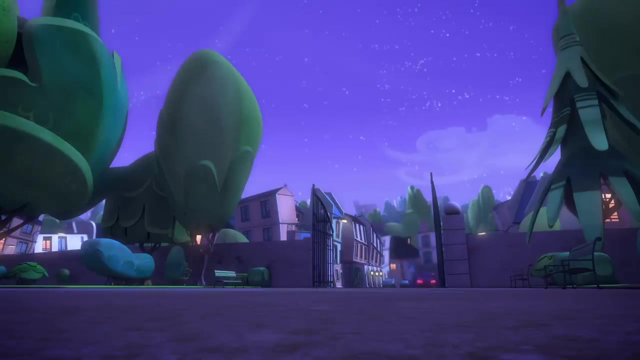 And a brave band of heroes is ready to face fiendish villains to stop them messing with your day. Amaya becomes Owlette- Yeah. Greg becomes Gekka- Yeah. Connor becomes Catboy. The PJ Masks. Students are ready to do what they have to do. 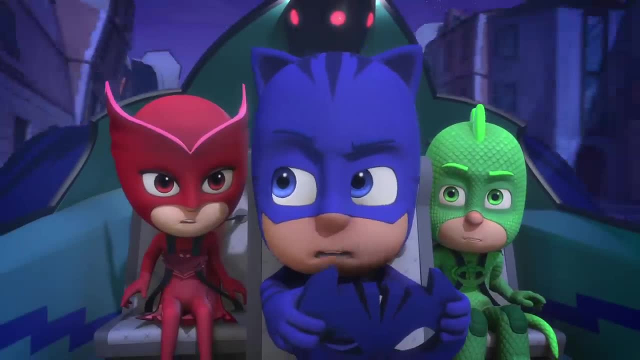 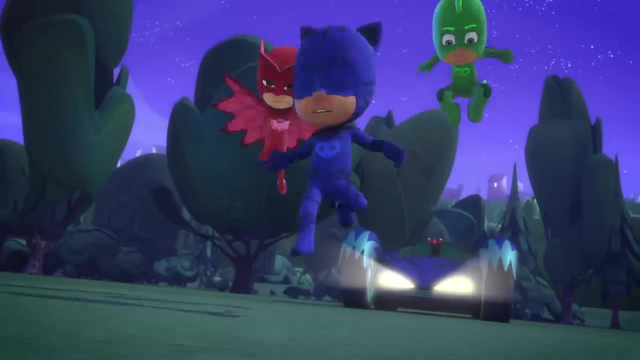 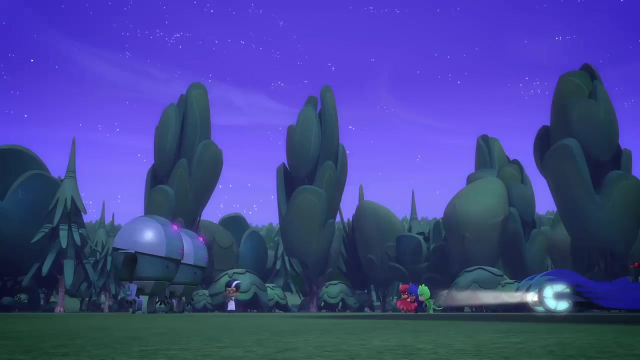 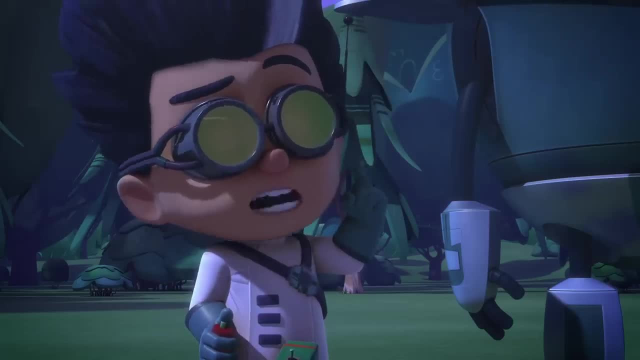 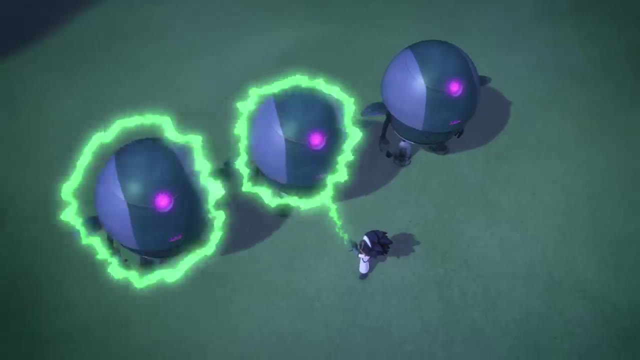 As soon as I invented the multiplying machine, I used it on itself to make a spare. Here it is Multiplying multiplying machine, Multiplying machines, Multiplying robots, Gaspin' geckos. we've got to get that machine. 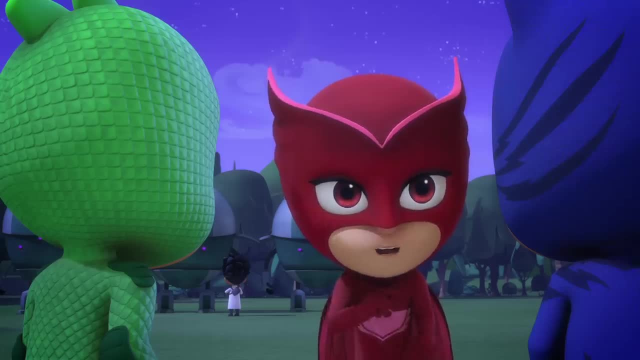 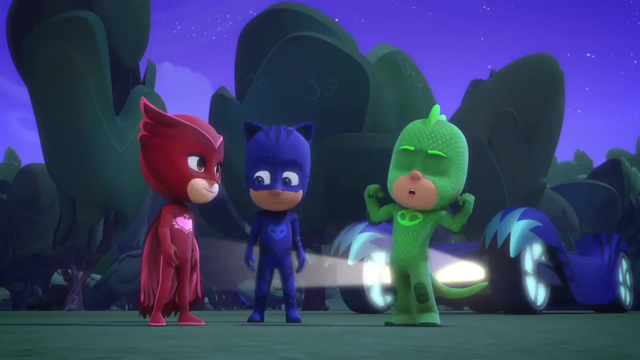 I have an idea. I'll swoop in and grab it from Romeo, then pass it to you, Catboy, and you give it to Gekko and I pull out the glowy thing and switch it off. Stand by for my super gecko muscles. 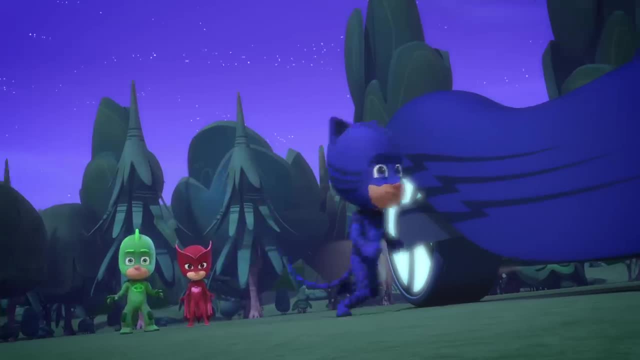 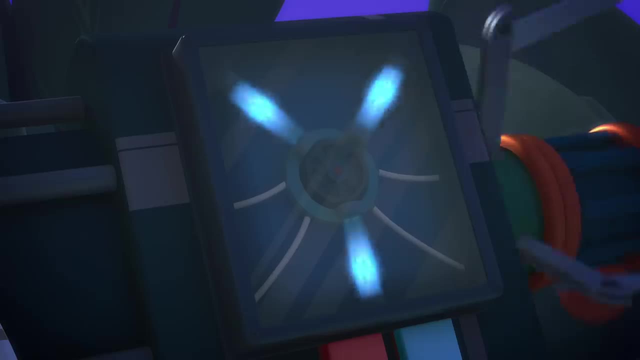 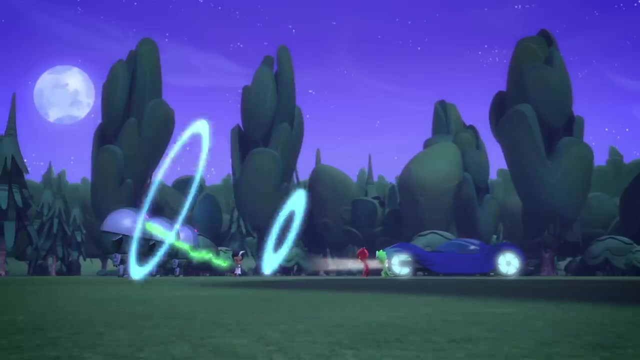 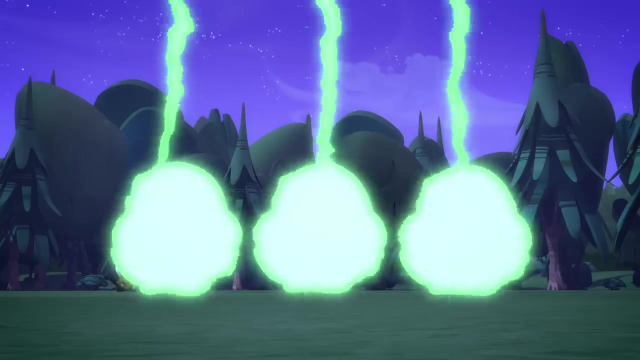 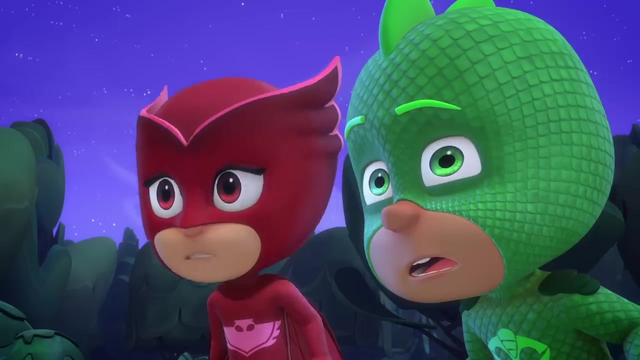 The cat roar. It's so loud it wrecks electronics. Wait Time to make more robots. And then there were four. Cat roar Whoa Oops. How nice of you to help my robot army grow Robot army, That's right. 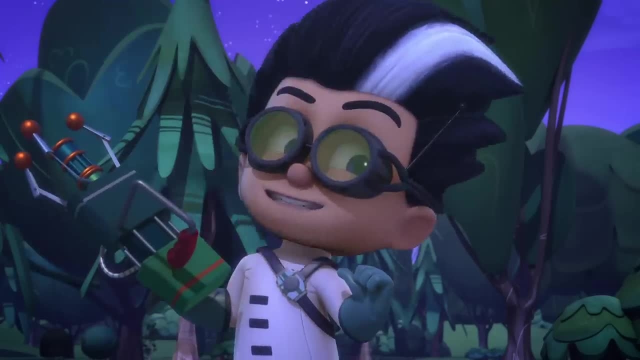 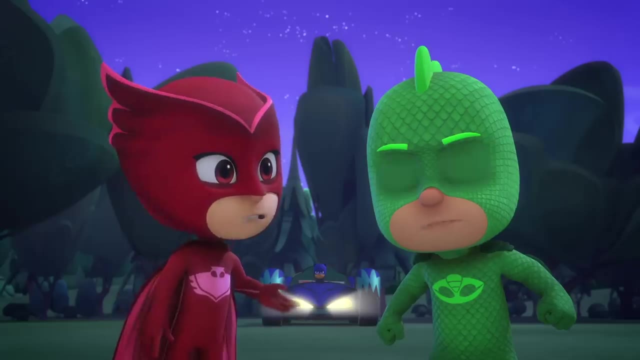 At last, everyone in the entire world will do as I say. What if we don't, Then my robot army will pick you up and hold you in the air until you do. If the robots do that, people will do whatever Romeo says. 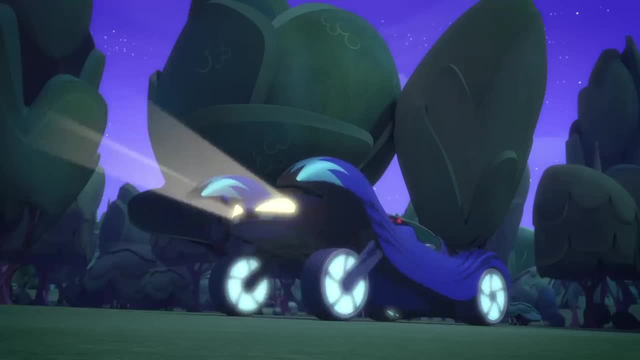 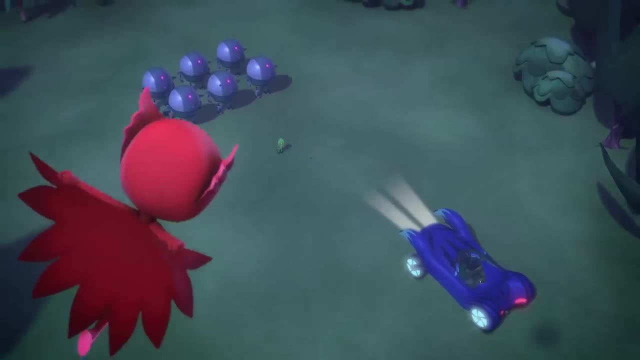 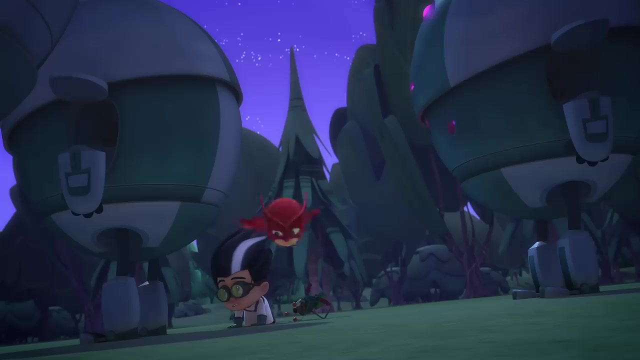 Okay, back to our plan: Fire furballs. Ah Fine, We'll do the plan with just the two of us. Now, where did the multiplying machine go? Super owl eyes There. No, Give that back, you fluttering fool. 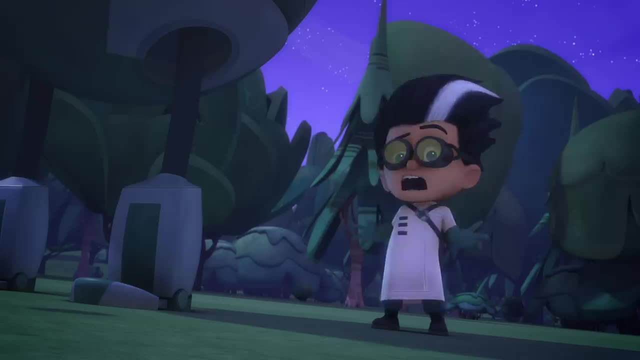 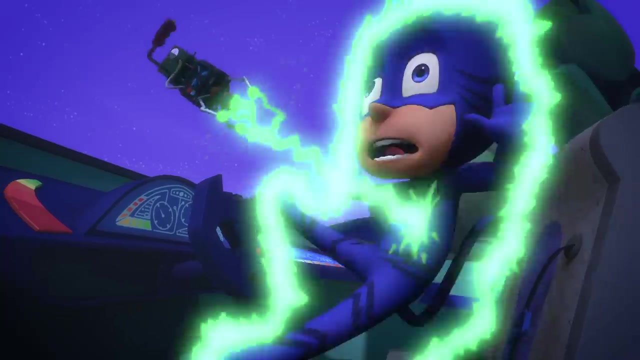 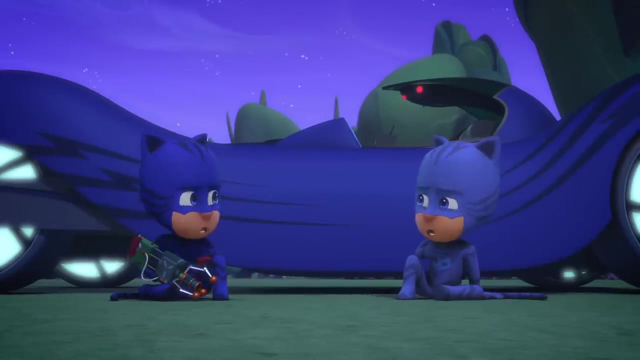 The furball button is stuck, It won't stop firing. Ah Huh, Ah, Ah, It's okay, Nothing happened. Yeah, I'm fine too. Oh, my cat's whiskers. Catboy, you've been multiplied. 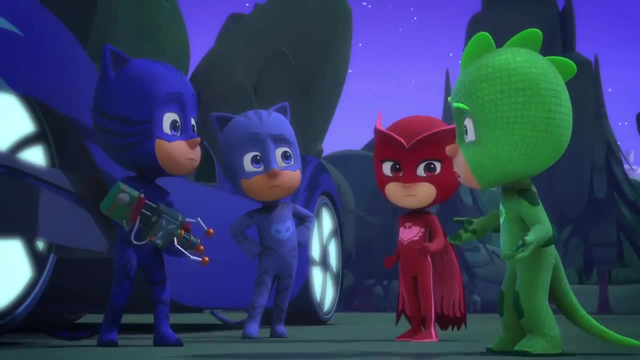 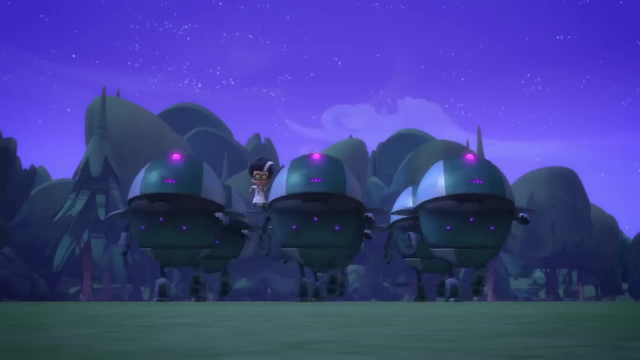 I know, I know too, But why does he look and sound different? Maybe the multiplying machine works differently on us because of our powers? The robots, Look, Get that machine now. robots, It's for multiplying you, not PJ Masks. 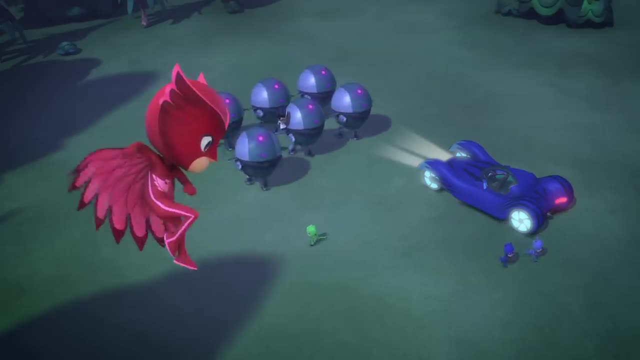 Throw me the machine, Catboy, I'll pull out the glowy thing. I can't. There's too many robots, But maybe, if there's a few extra, PJ Masks too. Yeah Yeah, Wiggling reptiles. Now there's four. 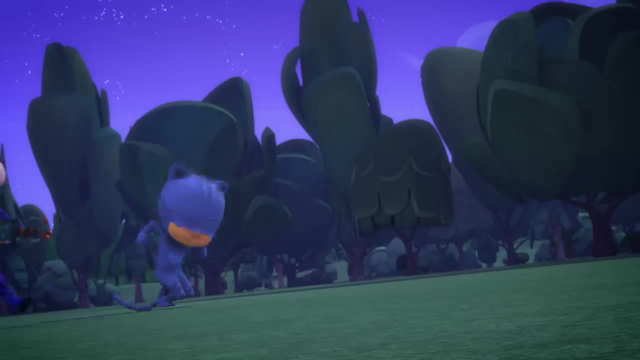 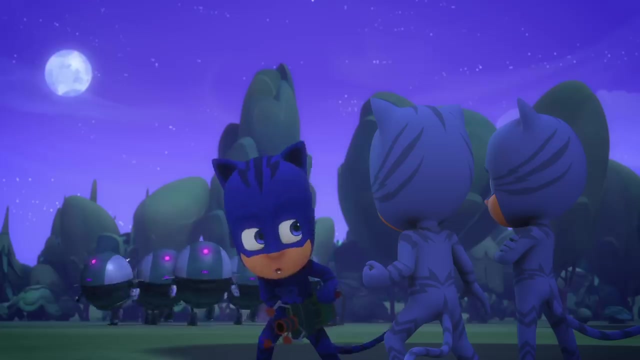 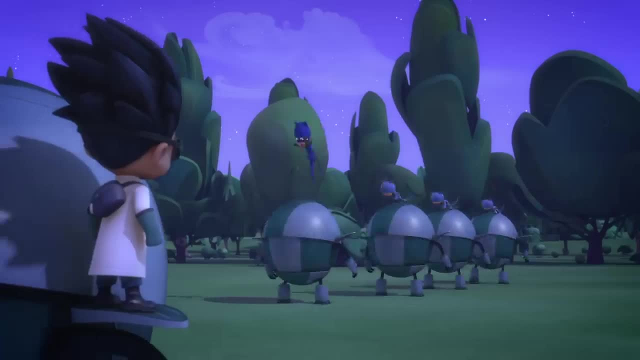 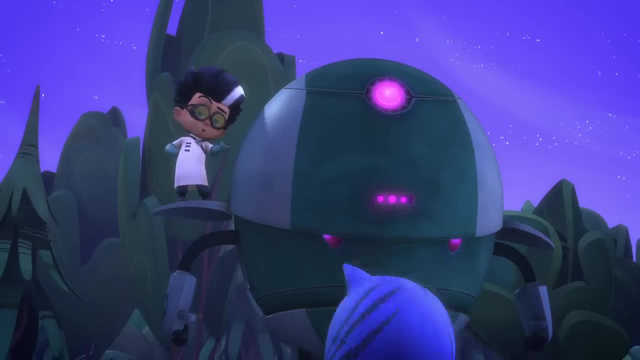 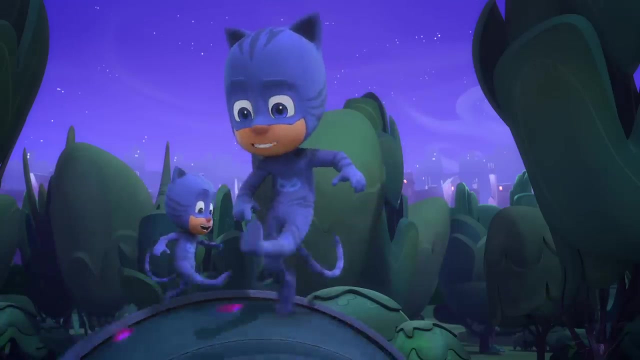 Oh, Oh, So long. robots, Not so fast. Looks like your copies have their own plans. What are you doing? Make them roll away. I've got a better idea. I'll spin this one until it gets extra dizzy. I'll race this one around the city until it's totally lost. 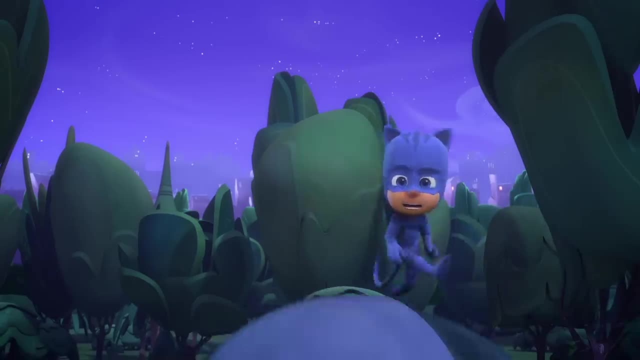 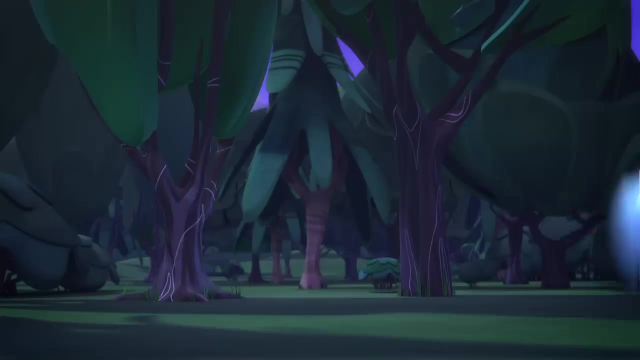 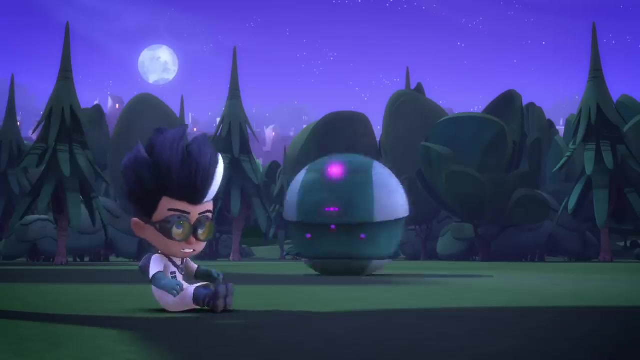 I'm just going to run mine as far as I can. This is amazing exercise. We have to get that machine back. Can we please do our plan now? Just give me one more try. I've got another idea, And with all these Catboys it can't fail. 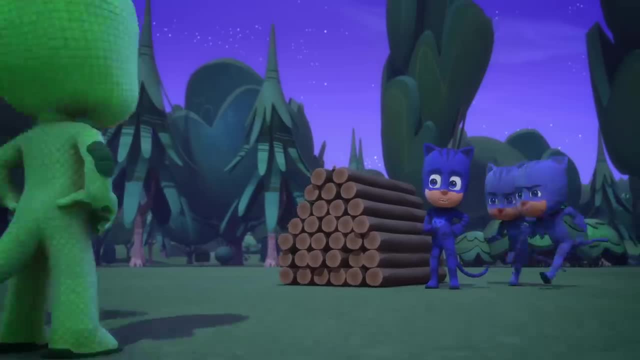 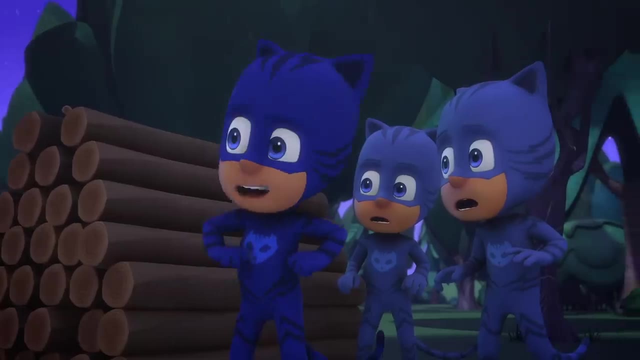 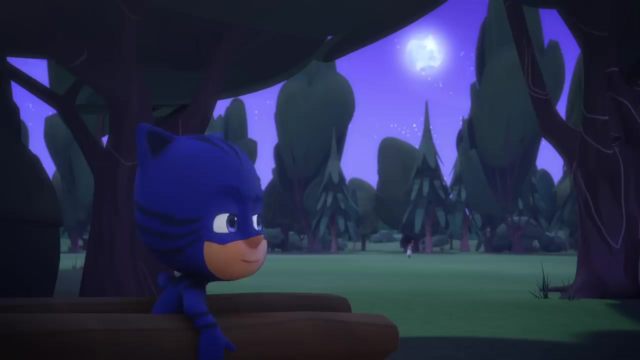 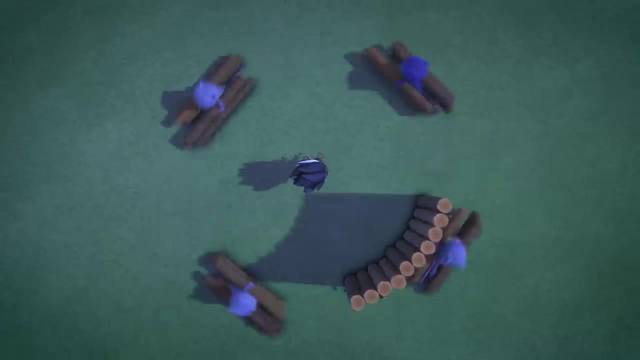 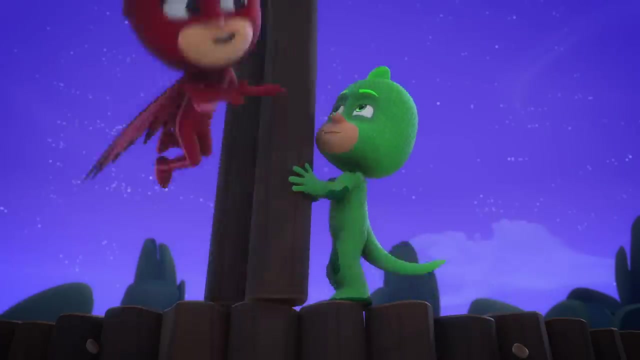 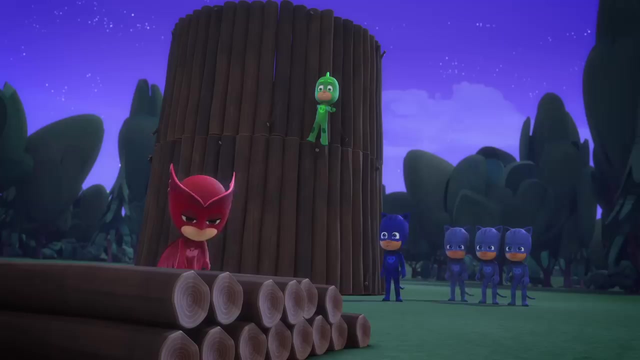 We'll use these logs to fence Romeo in. But how will we get the machine back? Huh, I'll explain later. Hurry, Huh, No, Why you PJ pests The robots. Let's build a robot trap instead. 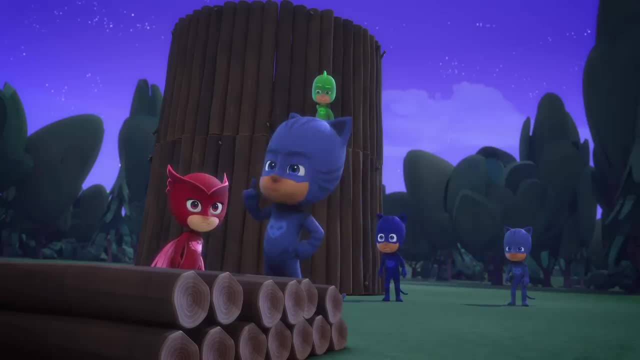 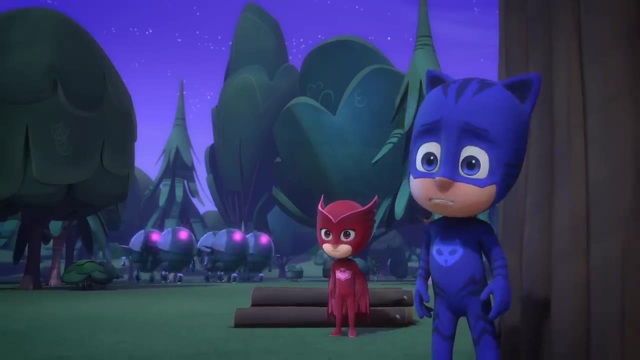 and spring it when they come back. I'm going to build a robot catapult. If I run on a log super fast, it'll trip up the robots for sure. Wait, Stop. We need those logs, I need them. Stop, Foggle the plan, Please. 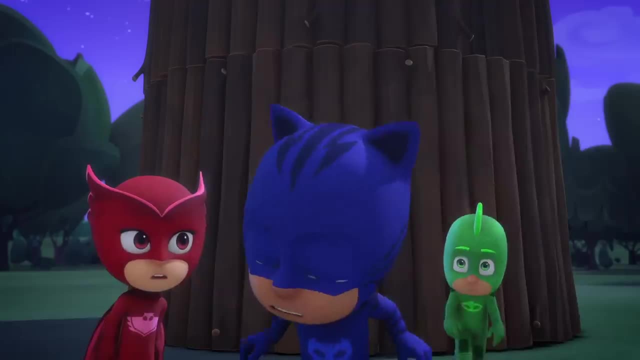 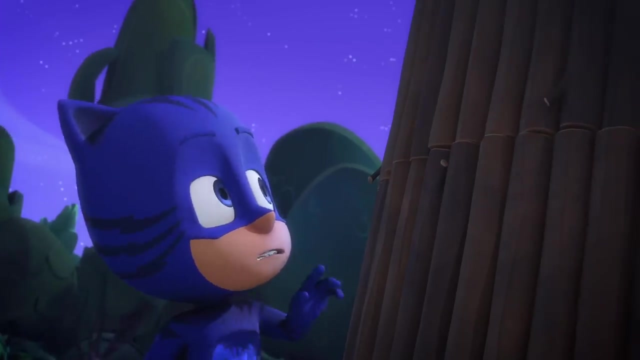 Let's do my plan, My plan. Just wait till you see my catapult. It's terrible. What's gotten into them? They're doing their own thing Like you. I can still fix this. I'll get the machine, Don't worry. 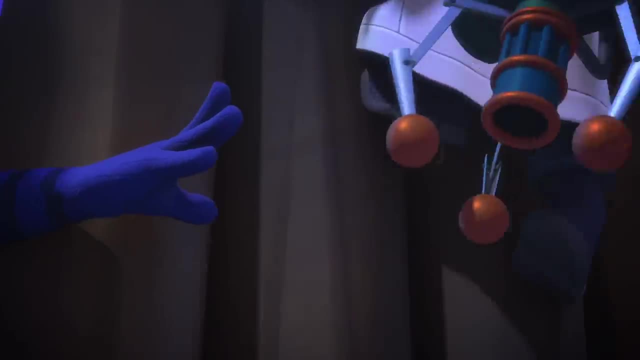 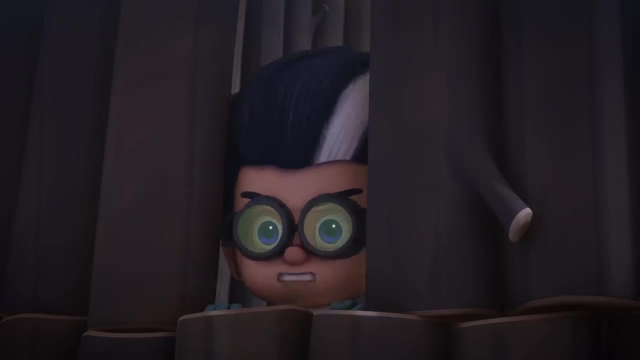 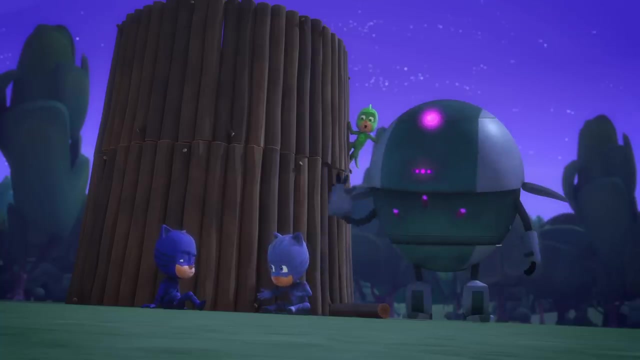 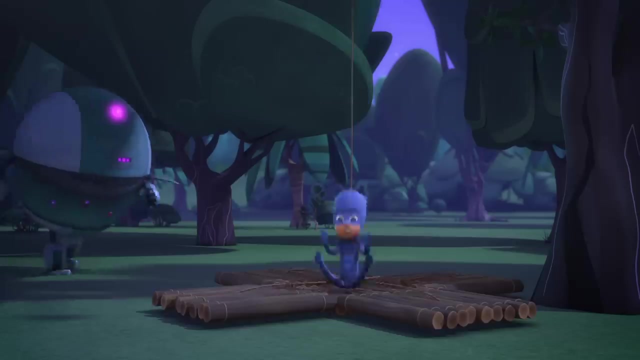 Catboy puts in a pod, Grabs the multiplier Coming through. Ah Robots, Where are those PJ pests? You ruined my plan. Hey, You ruined mine. Look out, Uh-oh, This is heavy One Catboy Coffee Master. 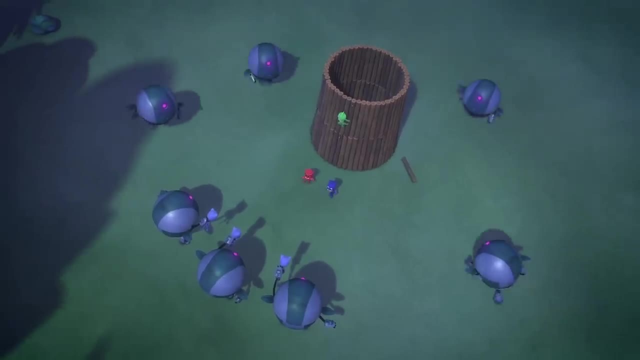 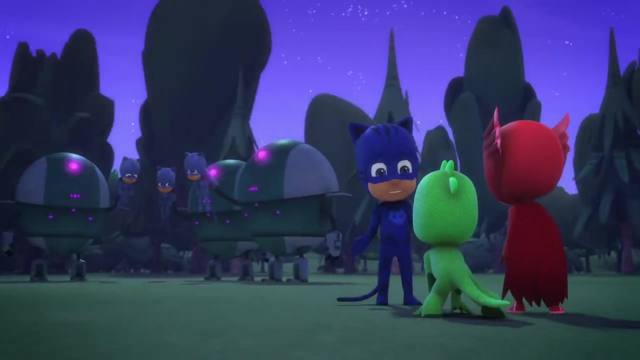 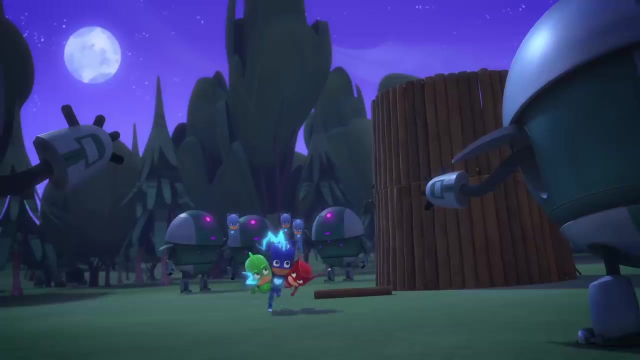 One Catboy Coffee Master. This is a catastrophe. You should have listened to us. We're a team, remember? I'm sorry, I forgot that. My coffees totally did. Sorry, It's time to be a hero, Super Cat. 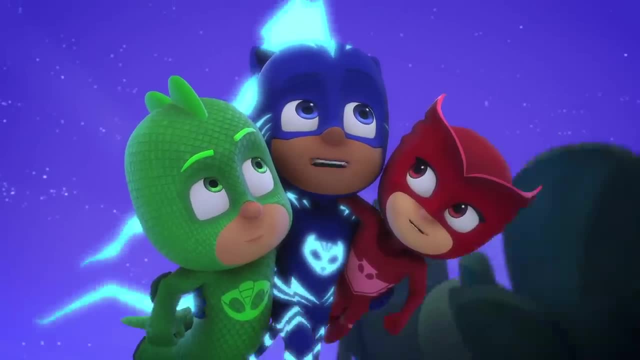 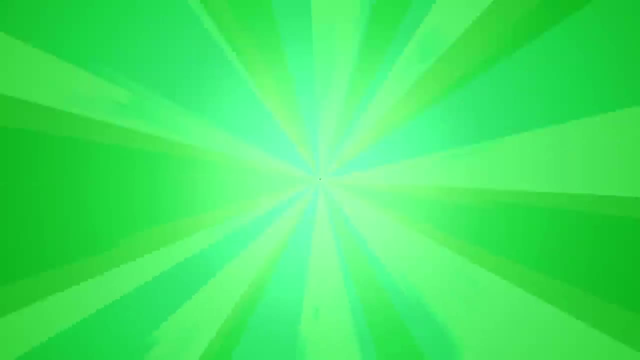 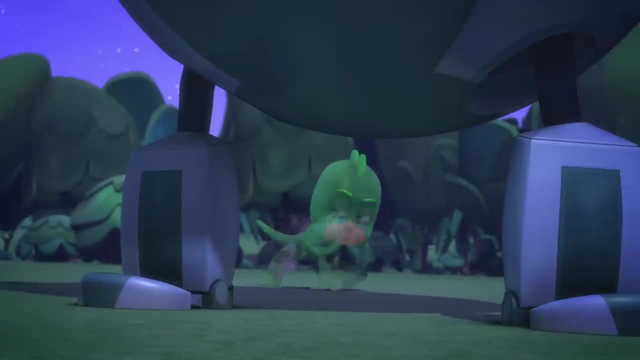 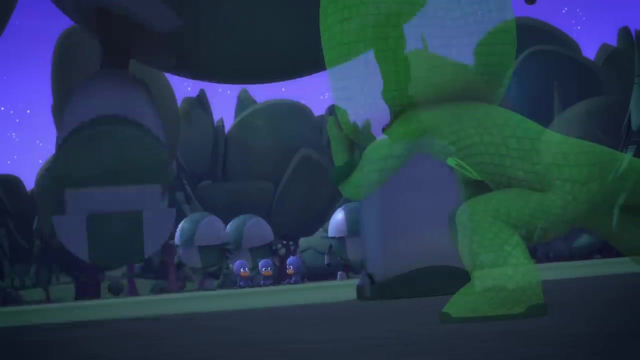 If we free my coffees, there'll be enough of us to beat the robots. Any ideas how? Team? I have a great one: The PJ masks. They're over by those trees behind you. Drop the Catboys in, Get them. 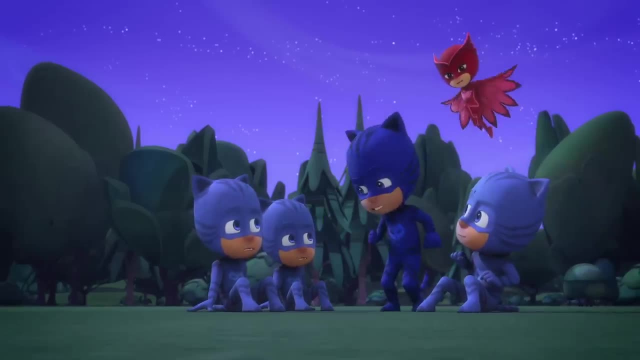 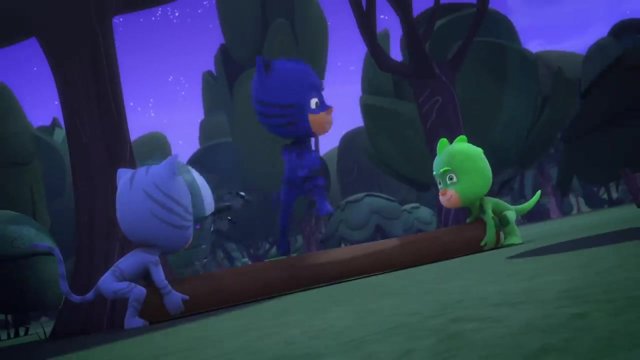 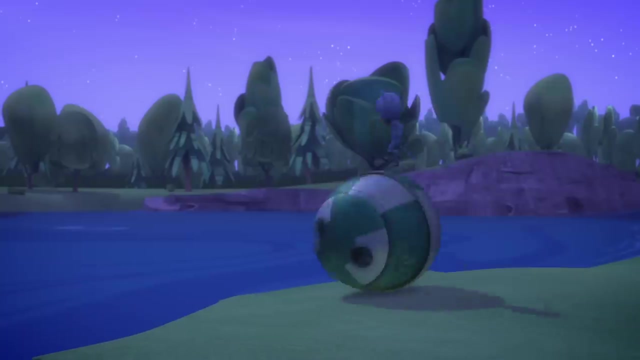 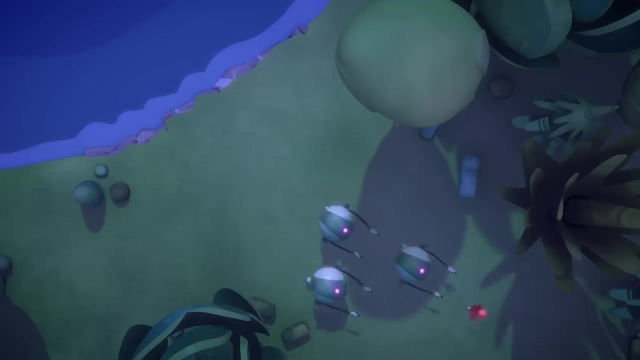 Stop tin cans. I'm nearly out. Okay, Catboys, Let's use your log inventions. Hello, Ow Ouch, Ouch, Yay, Here comes the rest. Let's take our places. Come on, robots. What are you PJ pests up to? 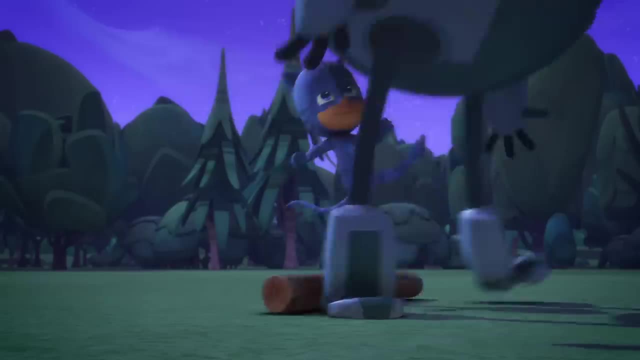 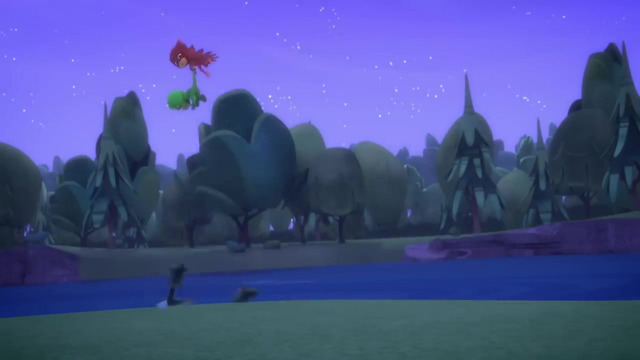 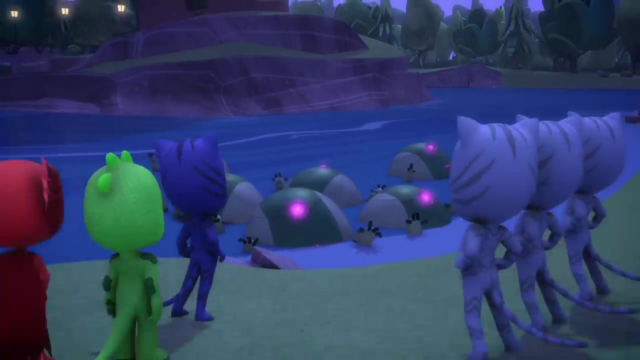 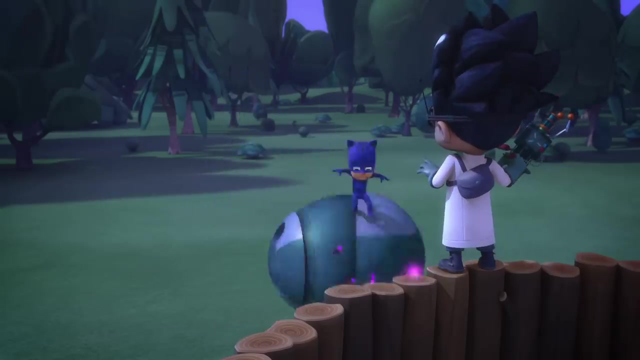 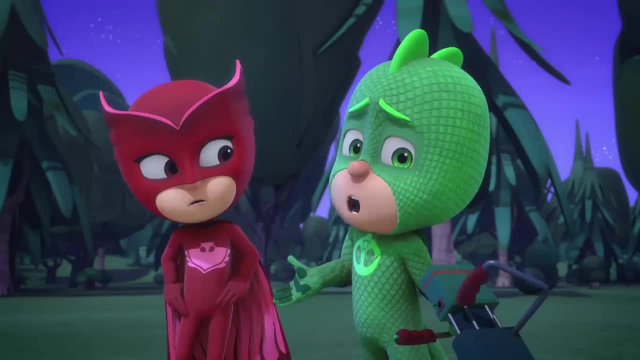 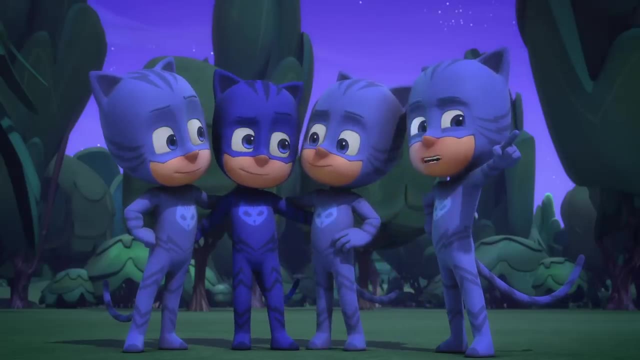 We did it. Now get those gecko muscles ready. But if I pull out the glowy thing, you'll disappear. We won't disappear, We'll just be one Catboy together again. Now that's a team. Do it, gecko. 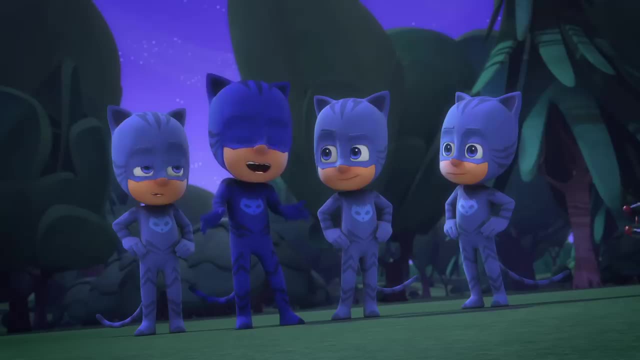 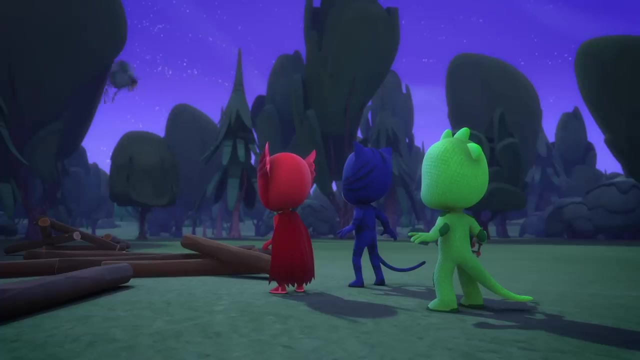 Super gecko muscles. Yeah Yeah, I'll get you PJ Pest. You got rid of my robot army, but you'll never get rid of me. Let's lock this thing up with the other one. PJ Masks- all shout, hooray. 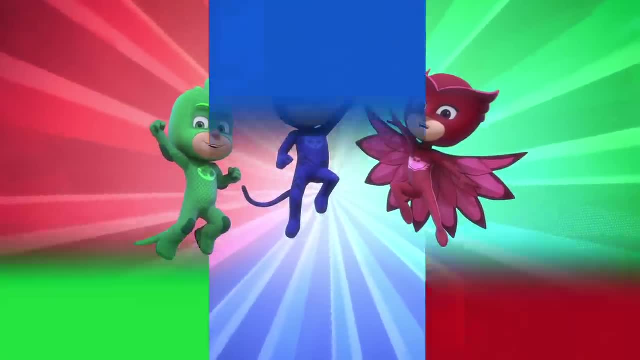 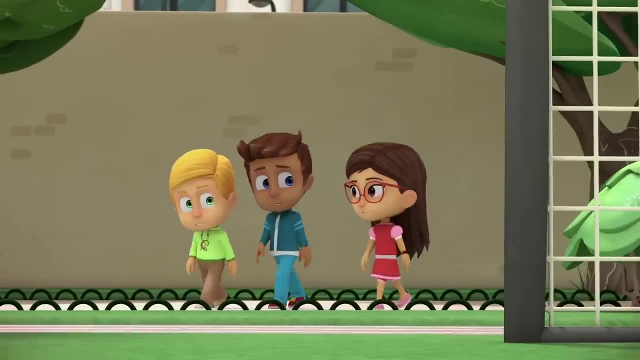 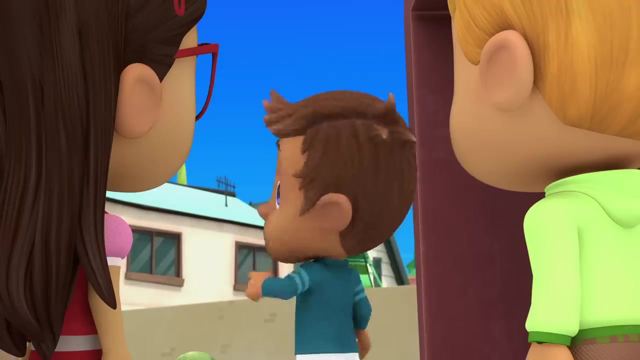 Because in the night you save the day. Everything is back to normal, And you're back to normal too, Connor, Totally. Now what are we going to play today? How about basketball Soccer? I love soccer. Let's play that. 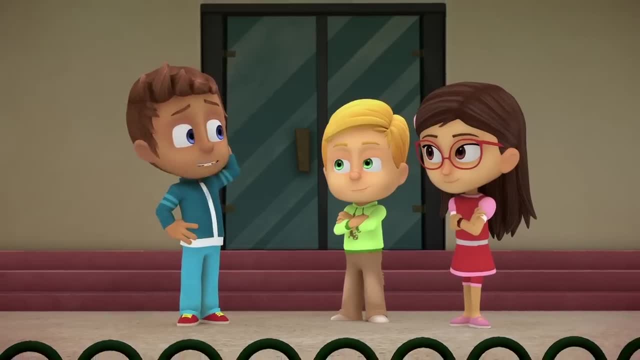 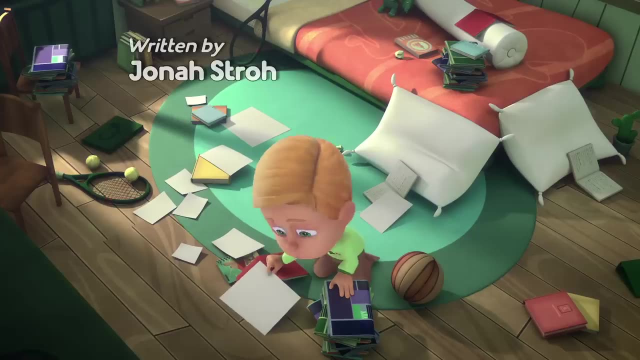 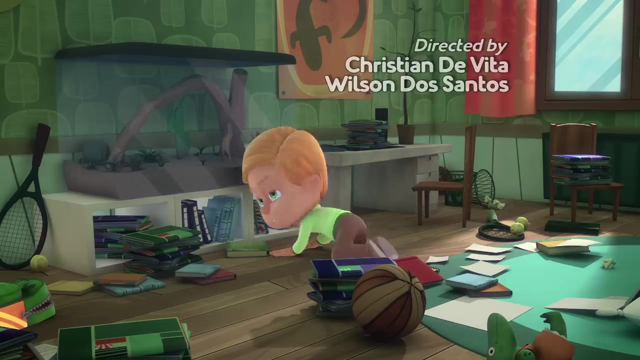 Ahem Uh, why don't you guys decide instead: Super-sized gecko? Come in Greg. This is Connor Over. Ugh, Where'd my walkie-talkie go? Hmm, Yeah, Ew, gross. Come in Greg. 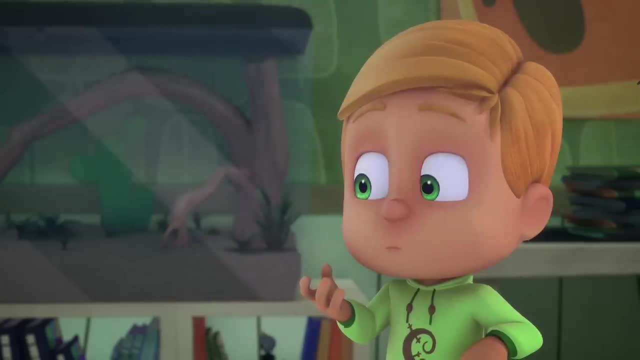 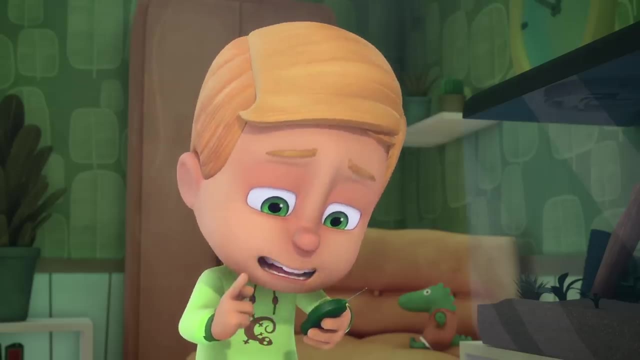 Hmm, Oh, there it is. Thanks, Lionel. Hey Connor, Oh wait, I mean copy that, Connor Over. Hey Greg, What are you doing Cleaning my room? It's a little messy And my mom won't let me go to the bathroom. 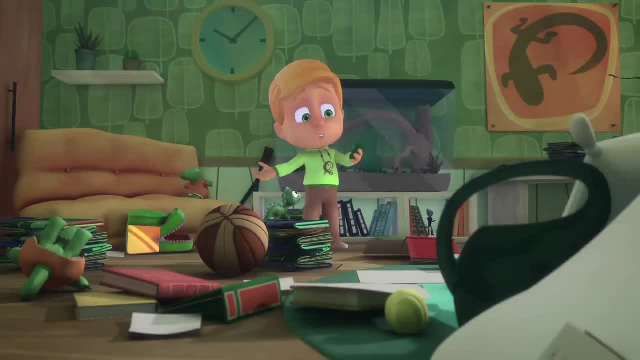 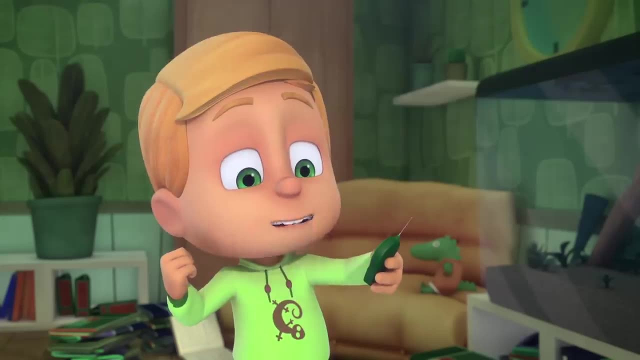 I'm sorry. I'm sorry. I'm sorry Mom won't let me go to the parade tomorrow if I don't clean it up. The parade's going to be awesome. I bet you can't wait for the lizard float. Yeah, it's my favorite. 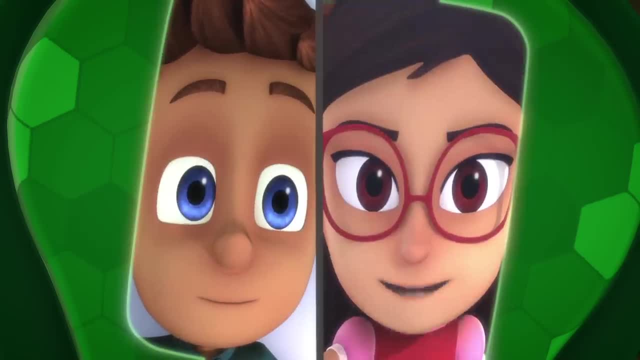 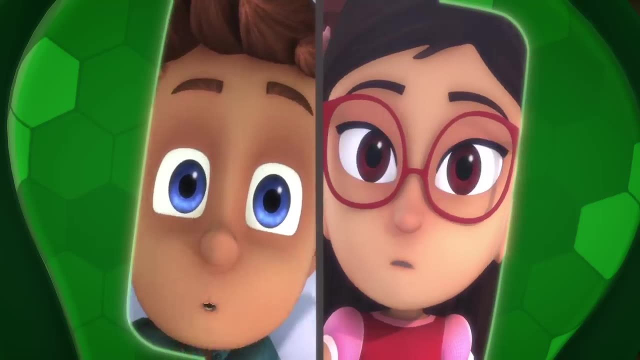 You better get cleaning then I'm going to HQ with Amaya, in case any nights have villains trying to ruin the parade. Go to HQ Without me, No way. But what about your room? Don't worry, I'll tidy up this mess later. 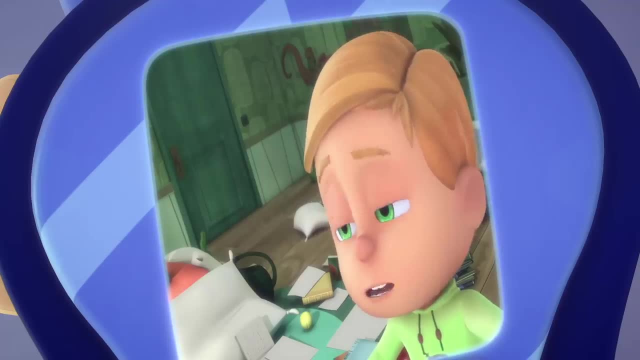 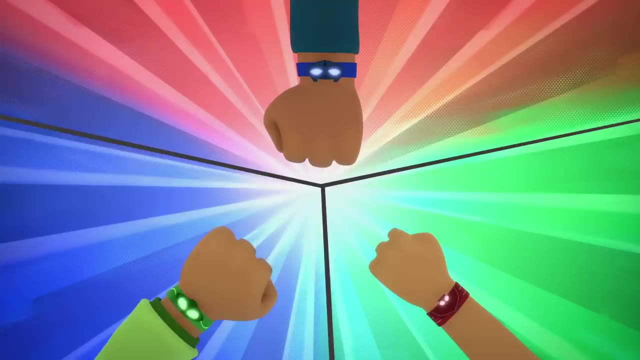 And I want to grab my camera for the parade. It must be at HQ. I can't seem to find it here. Okay, PJ Masks, we're on our way. It's the night to save the day, Night in the city. 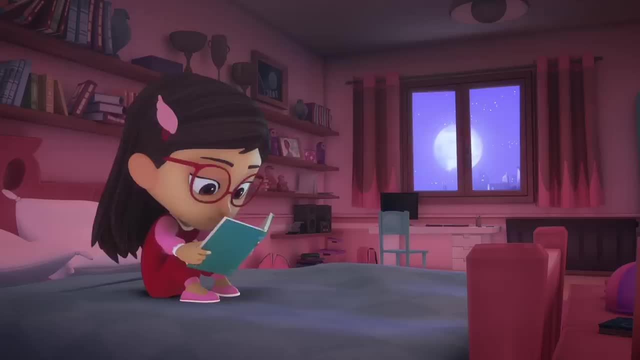 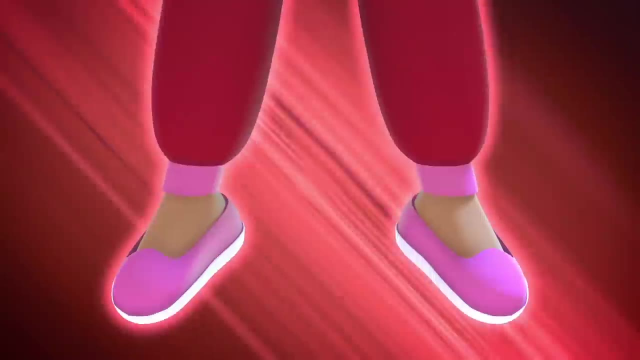 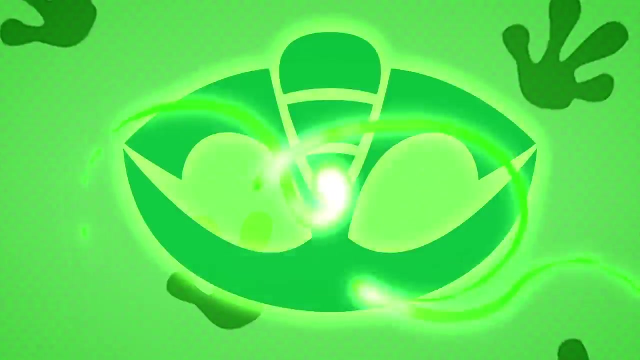 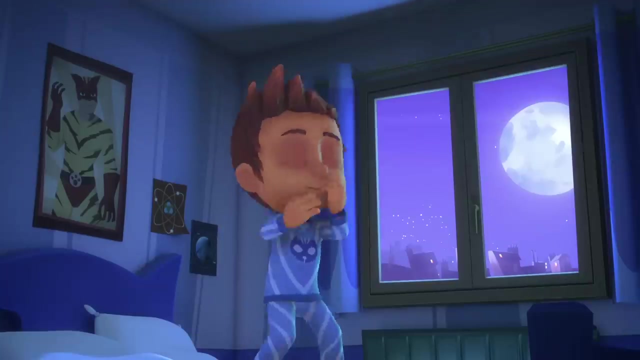 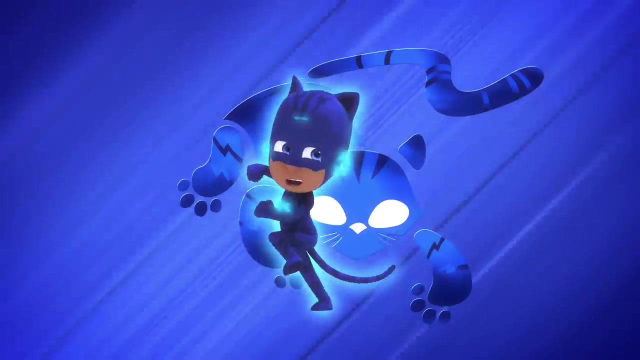 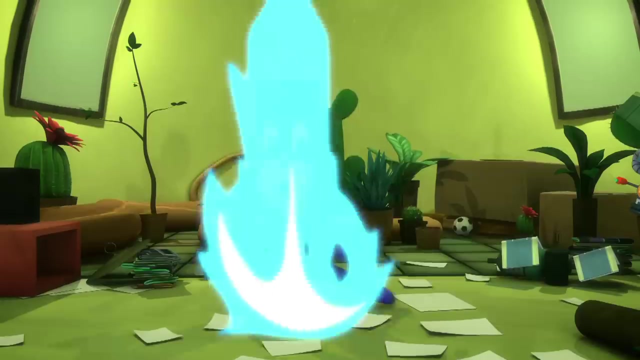 And a brave band of heroes is ready to face fiendish villains to stop them messing with your day. Amaya becomes Owlite- Yeah. Greg becomes Gekko- Gekko, Yeah. Connor becomes Catboy, Lucky J. 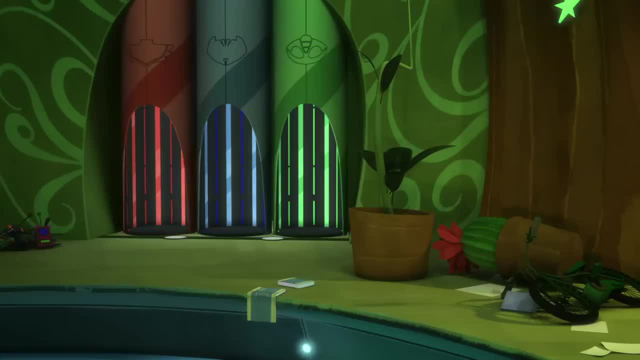 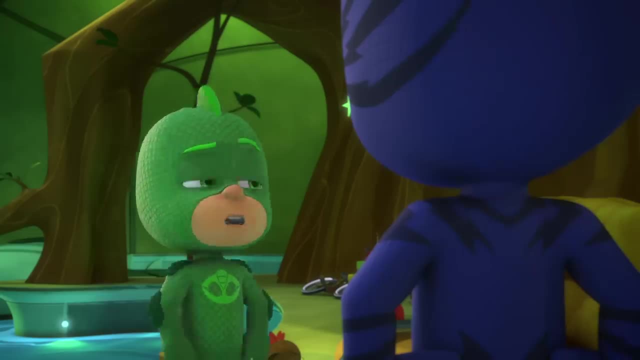 Yes, Gekko, it's as messy here as in your bedroom. You said you were going to clean this up. Right, I was going to do it. I'm going to clean this up Later. Here's Romeo's Sniffle Whiff and here's the small-sizer. 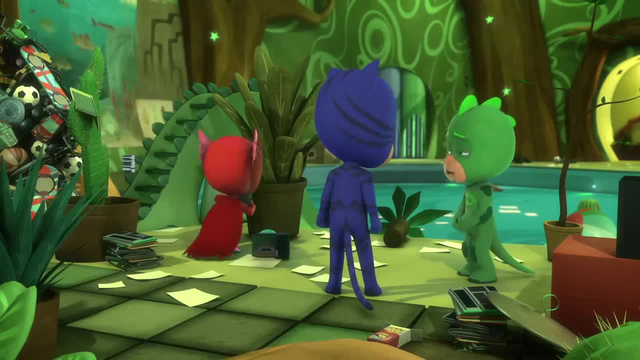 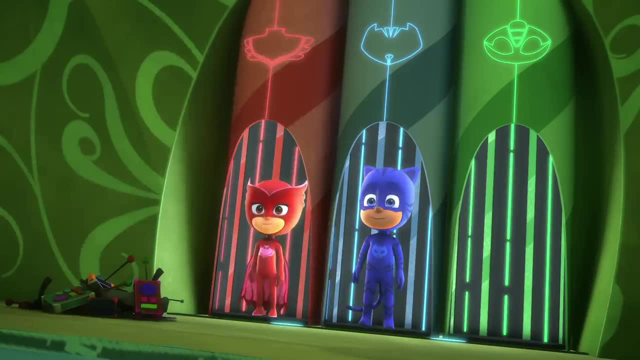 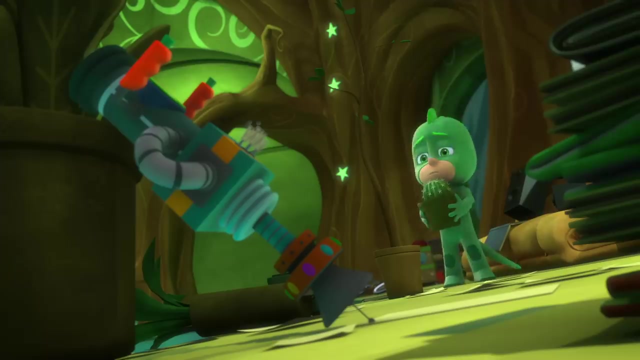 You were supposed to put them away somewhere safe. Yeah, I know, but It's okay. We'll keep an eye out for parade trouble while you clean up. No playing with Romeo's gadgets. Okay, But it's not playing if I use the small-sizer to clean up. 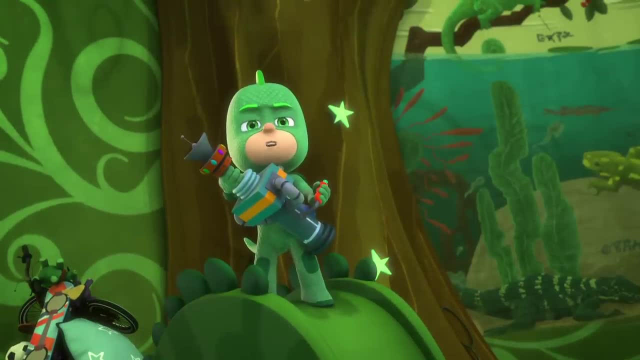 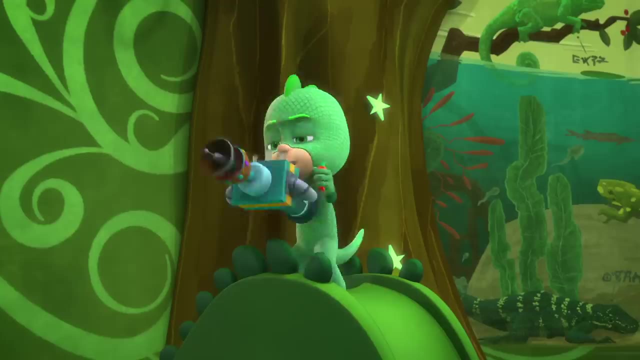 I'm Romeo, and once I've talked to Romeo, once I've tidied my room, I'm going to take over the world. Mwah-ha-ha-ha-ha-ha. Hmm, I wonder what this button does. 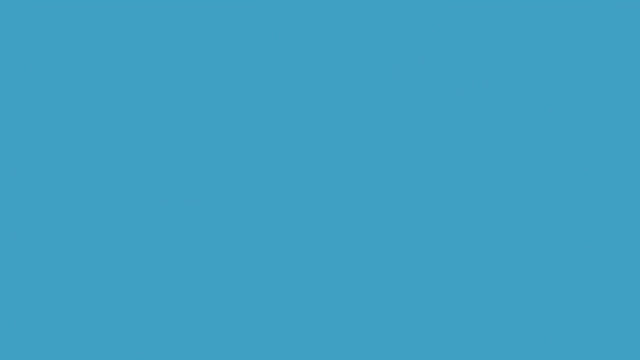 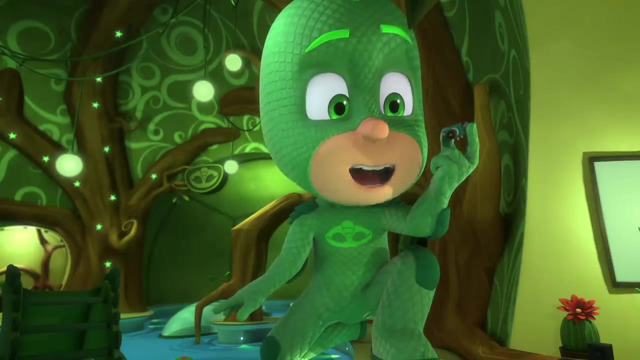 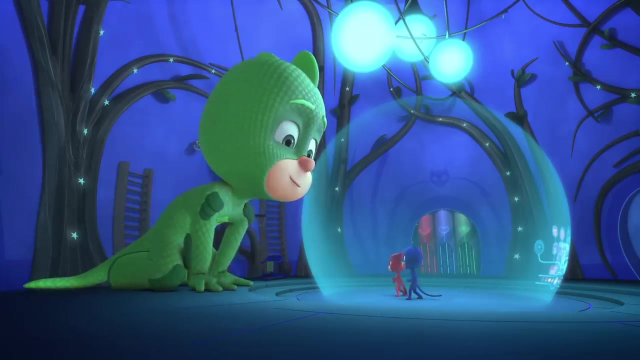 Ow Aw Ugh, Slithering Serpents. Now it's a super-sizer. Awesome, Hi guys. Huh, Gekko, Who did this to you? I might have kind of hit myself with Romeo's small-sizer. 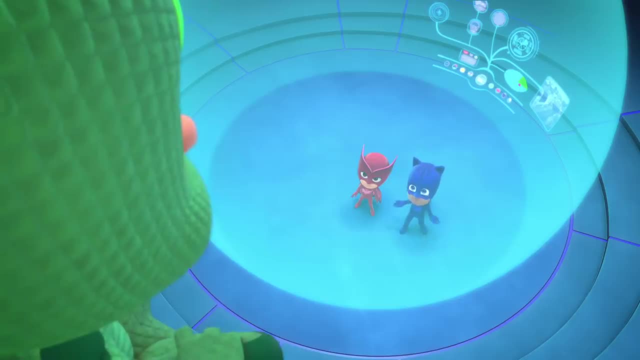 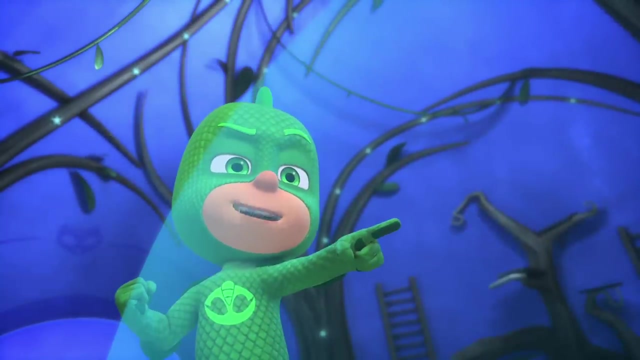 but in reverse. so now I'm big, Don't worry, we'll get you back to normal. No, it's really cool being Giant Gekko. I'll stop anyone messing with the parade. I'm huge. Uh-oh, trouble at the parade ground. 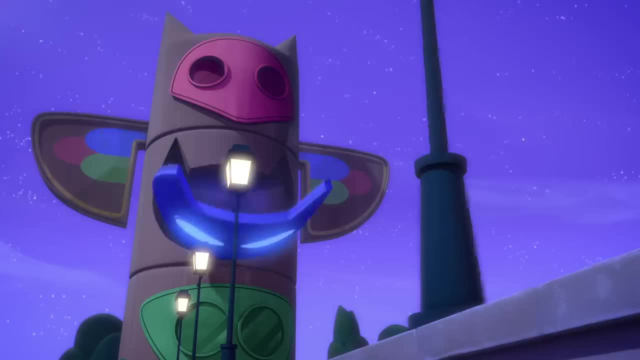 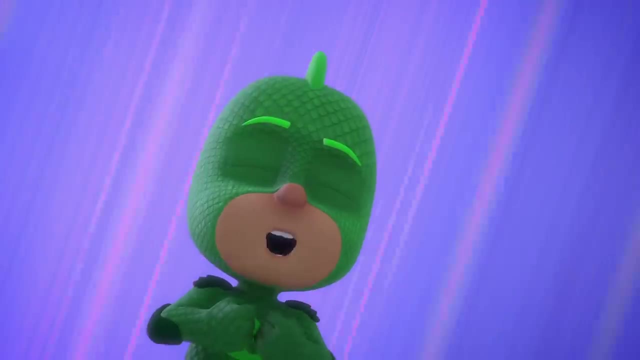 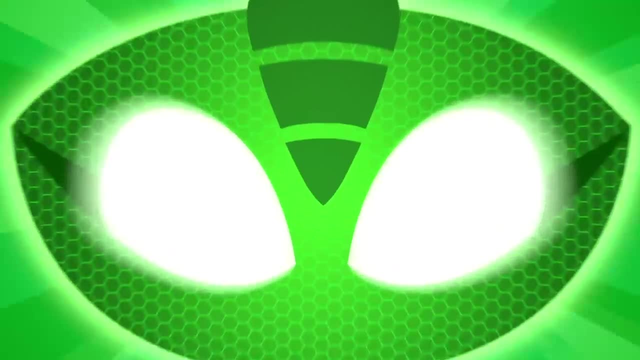 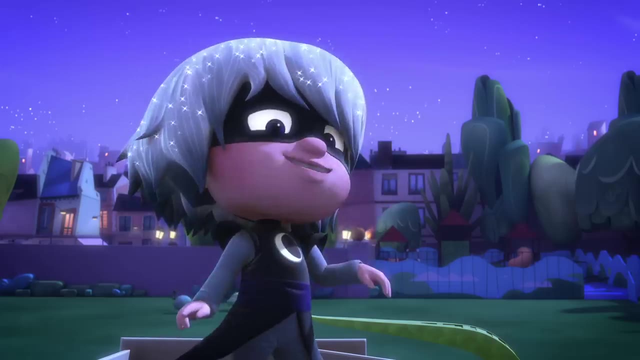 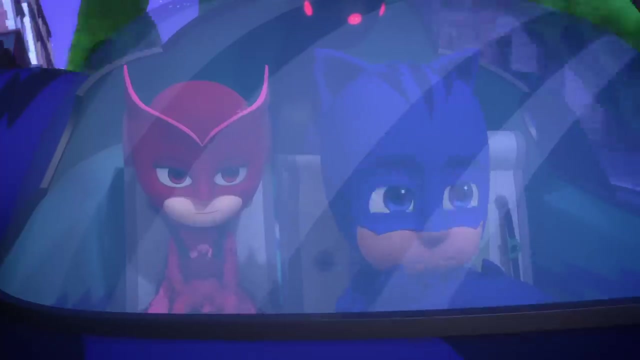 Roar, This parade will be mine. moths, We're going to steal these floats and make me the parade queen. Now cheer my lunar loveliness. Roar Slithering Feathers. What's happening? I'll get you to the parade ground super-fast. 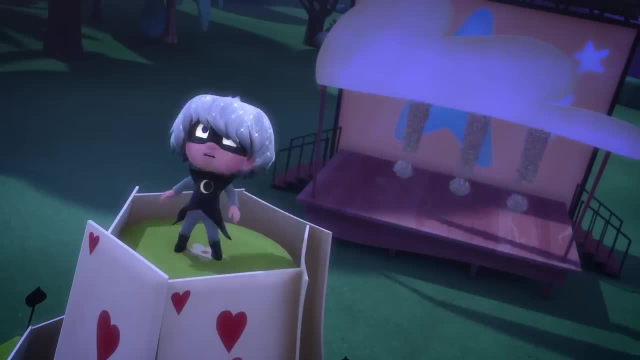 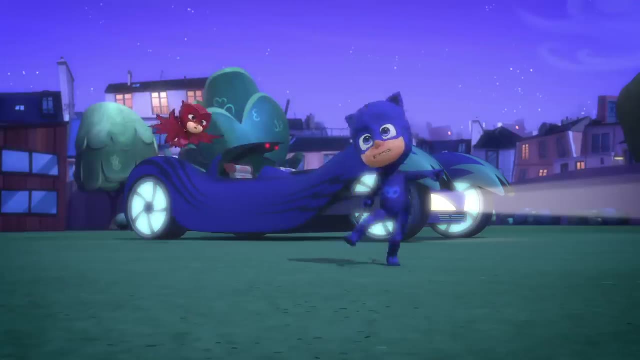 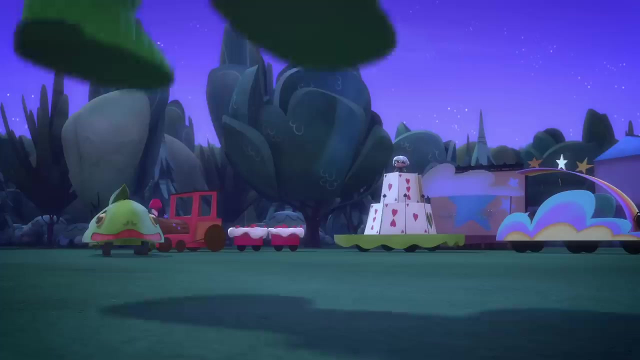 Whoa, Whoa, Ah, What? Whoa? Ah, Ah, Ah, Ah, Ah Ah. Nice entrance, do-gooders, Roar. Ah, What is that? It's Giant Gekko here to stop you taking the floats. 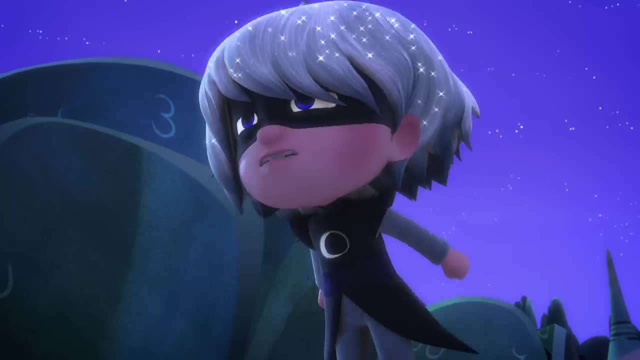 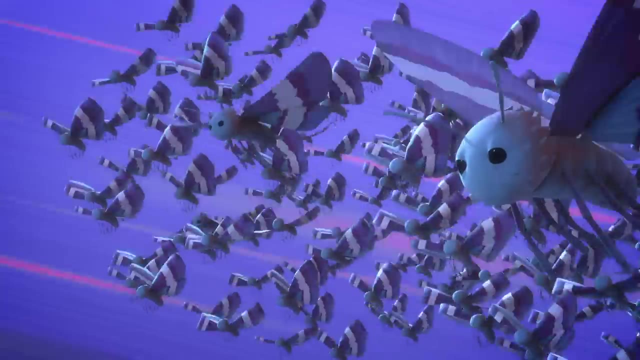 especially the lizard one. It's my favorite. No way, Once I've got them all, I'm taking my Luna Parade down Main Street And waking everyone up. Get him moths. Ah, Boo, Ah, Ah, Ah. 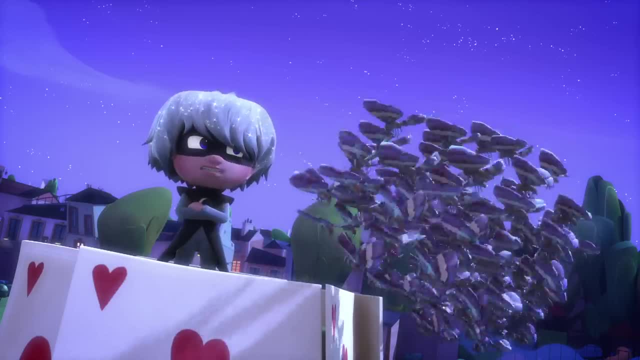 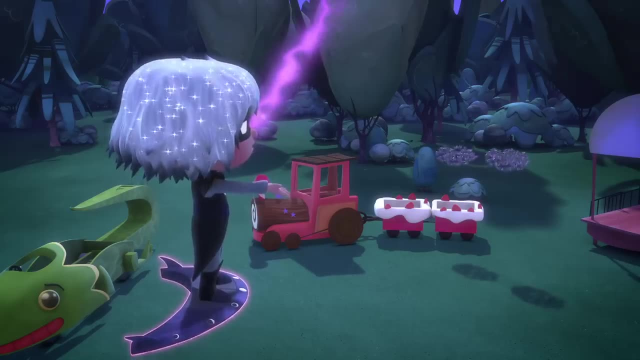 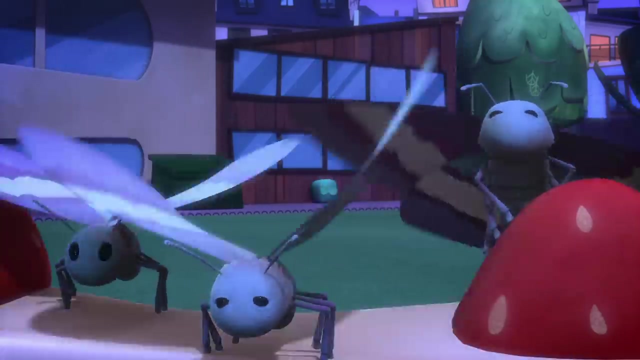 You just can't get good help these days, Luna-Bard. Ah, Moths, get the other floats and follow me. Ah, Ah, Ah, Ah, Ah Ah, Come on, Pick them up. You're not putting your antenna into it. 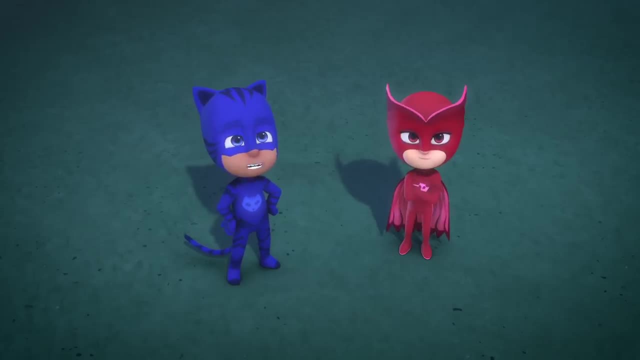 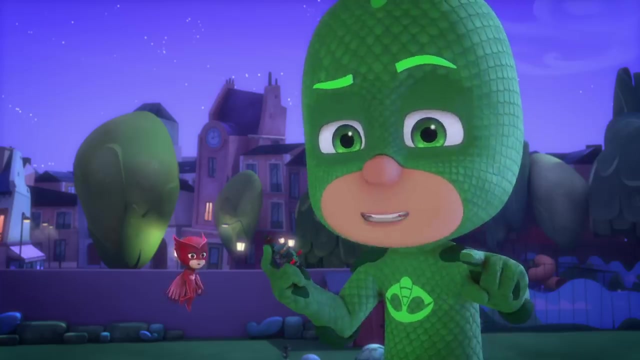 We can't let her wake everyone up and see her. But don't worry, I've got a plan. Wait, so do I And mine's big Gekko. what are you doing? Supersizing this bin, If I make it just a bit bigger. 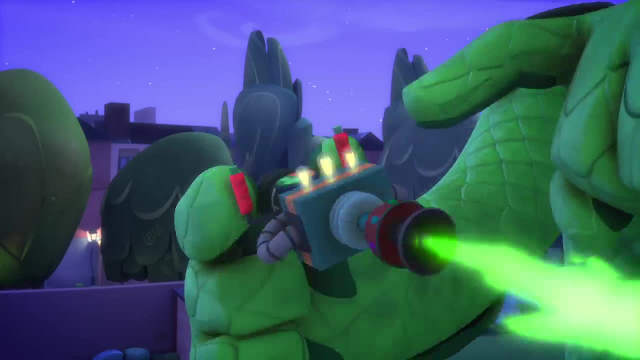 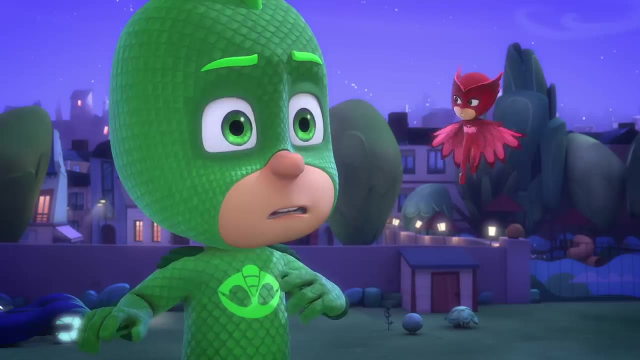 it'll be perfect to hold Luna Girl and her moths. Ah, Oh no, Oh yes. Hurry, Gekko, shrink it. Don't worry, I'll fix that later. I just need to make the bin even bigger. 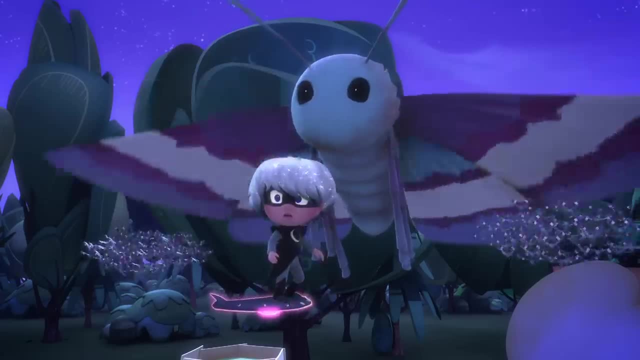 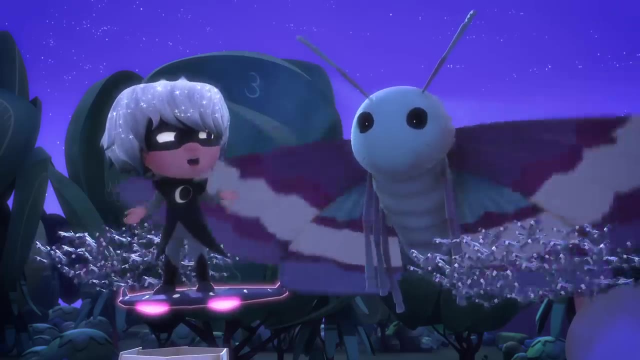 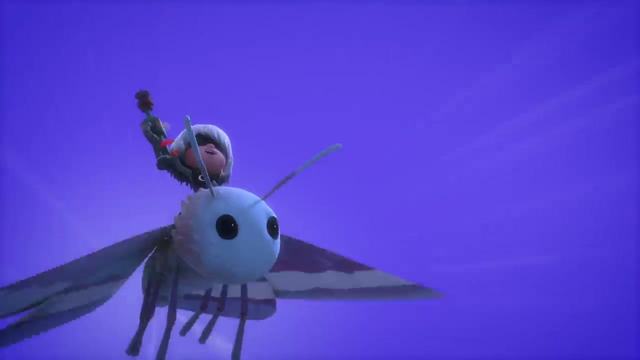 Look out The big PJ Masks just made a big mistake. Wait, who needs a Luna-Bard when I've got a super moth? Ah, This supersizer is mine, All mine, And now I can have all the floats. All I need are more giant moths. 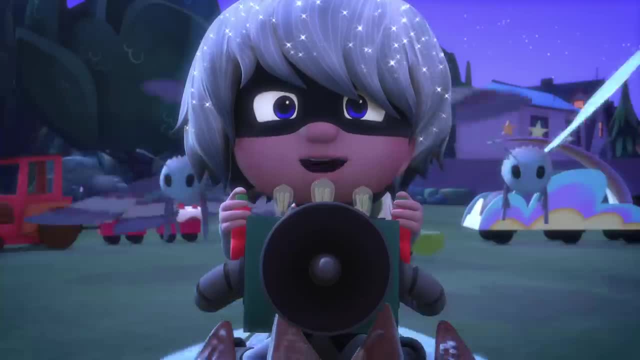 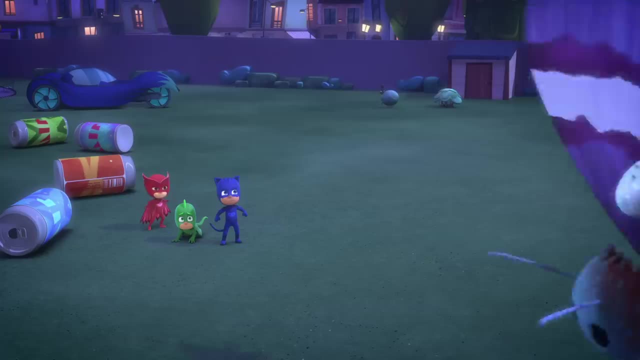 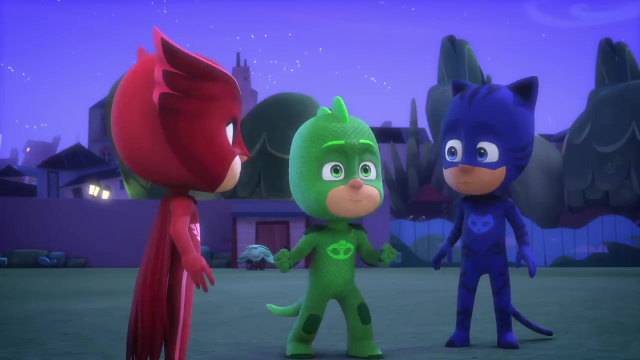 And one more thing: See you later, alligator. Oh, but you're just an itty-bitty lizard now. What are we gonna do now? Get the supersizer and make me big again. No, Gekko. First we have to clean up the giant moth mess you made. 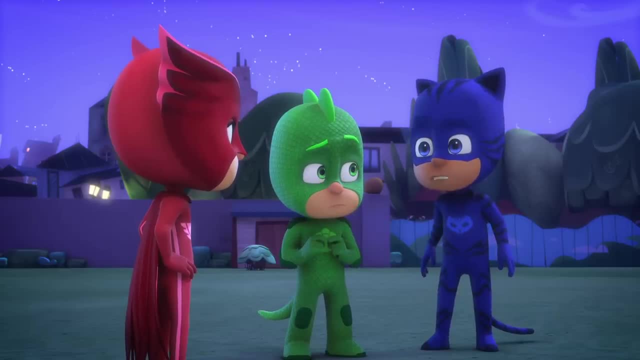 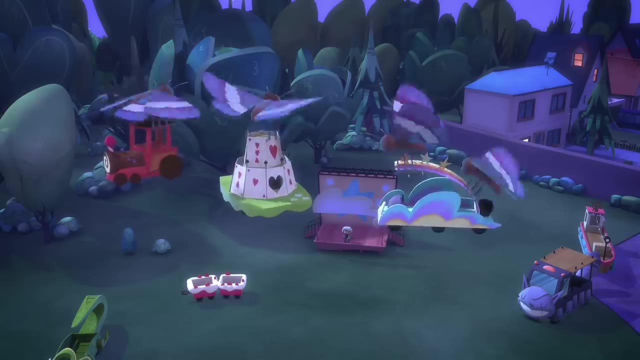 Okay, Owlette, get the moths to chase you till we get the supersizer from Luna Girl, Then fly them past Gekko and he'll shrink them. Good, giant moth, Good Hey moths, Bet you can't catch me. 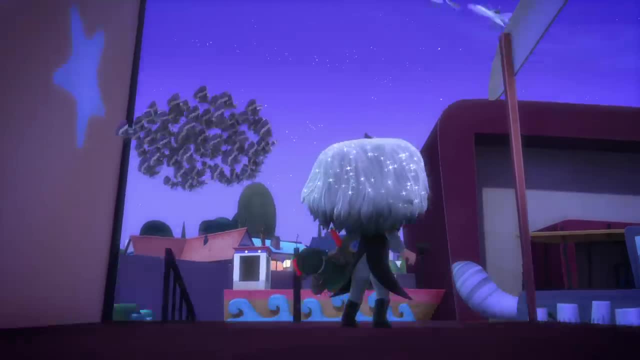 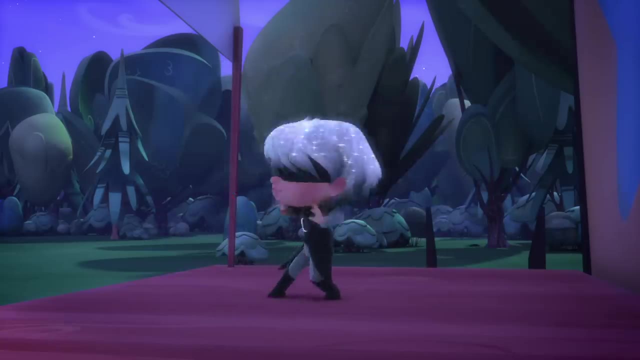 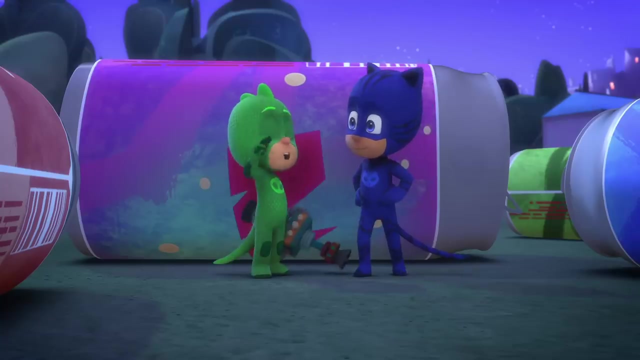 No, Come back here, Super Cat's feet. Ugh, I'll take that, thanks. Remember Gekko, When Owlette flies by with the moths? shrink them down. Got it, Catboy? Great, I'm gonna check on Luna Girl. 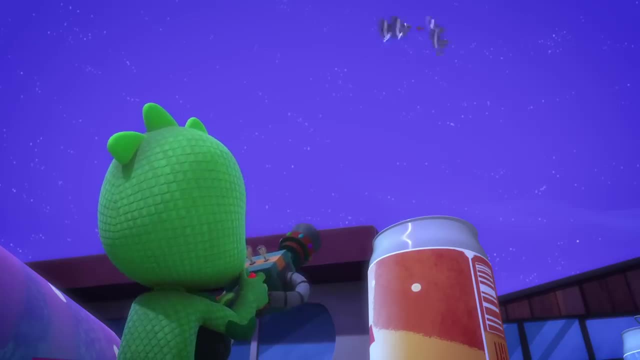 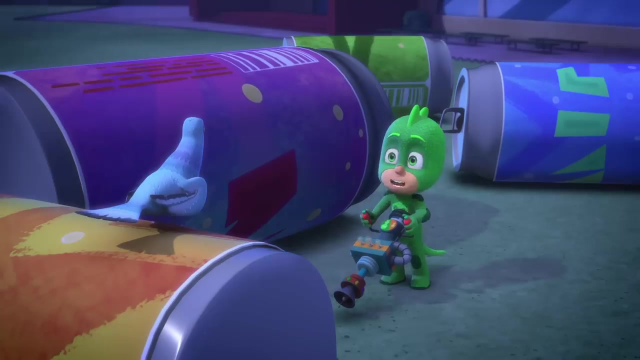 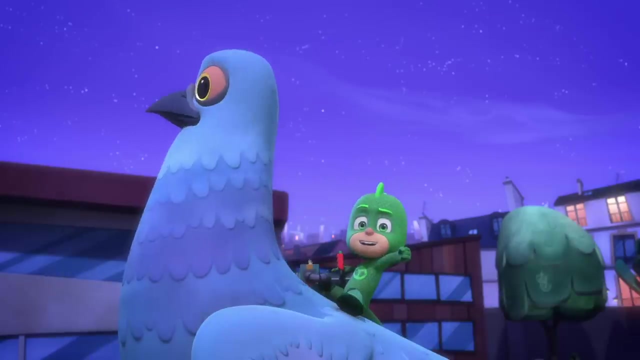 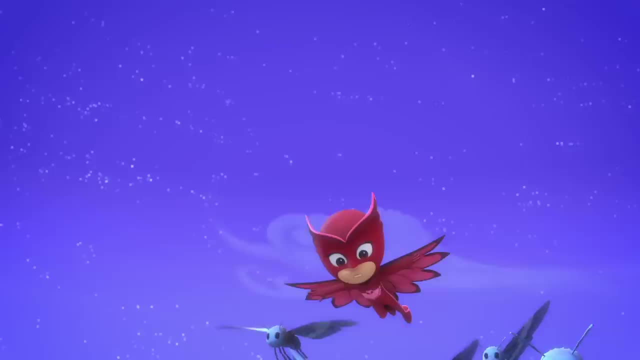 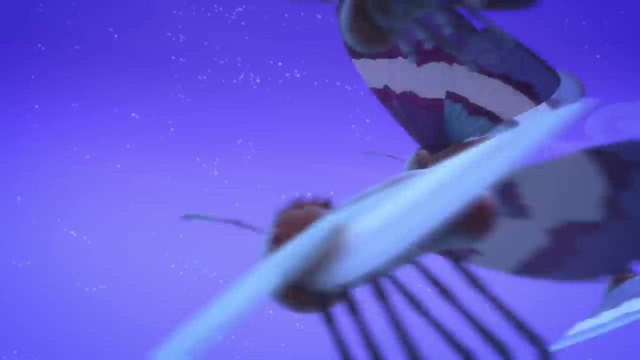 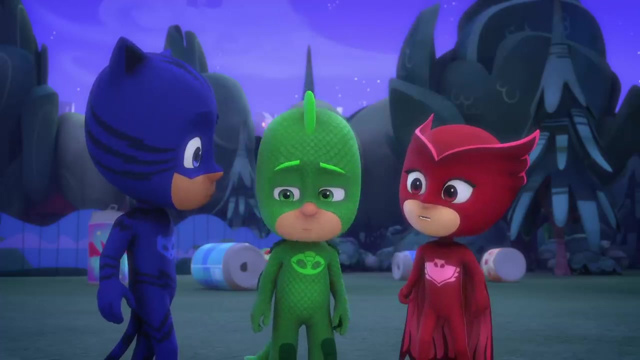 Ah, Ah, Ah, Ah, Ah. Gasp, Gekko, Gekko. Ah, yes, Are you okay? Gekko, Yeah, Ha-ha-ha, Looks like I win PJ Pests. The whole parade is mine. 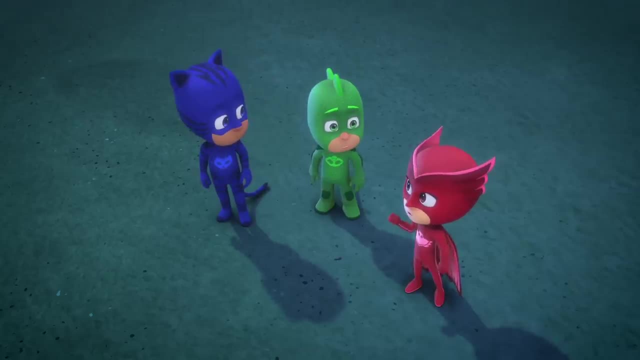 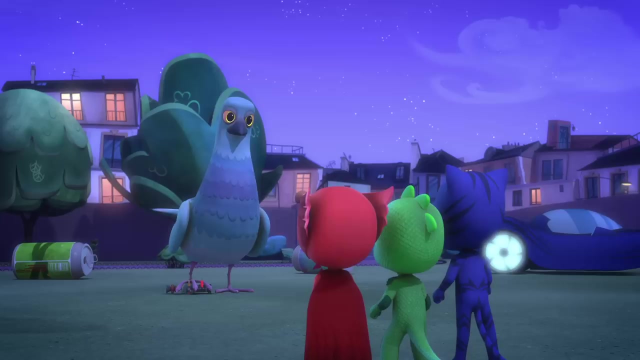 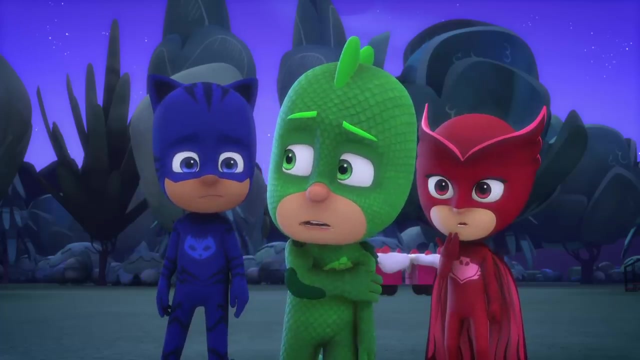 All mine. Gotta shrink those moths. It's our only chance. But I lost the Super Sizer again. There it is, Huh, Ah, Now, what are we going to do? Oh, this is all my fault. I'm sorry. I didn't clean up my messes when I made them. 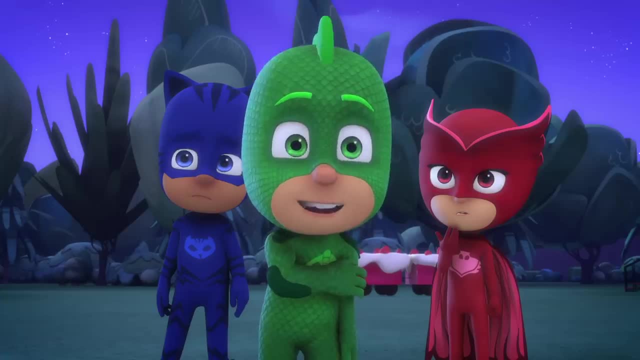 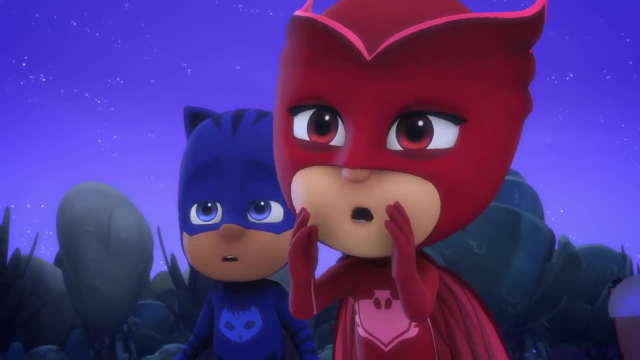 Huh, Wait, It's time to be a hero. Caw, Caw, Caw, Be careful, Gecko, Don't do anything to get it excited. Oh, that's exactly what I'm going to do Here. birdie, birdie, birdie. 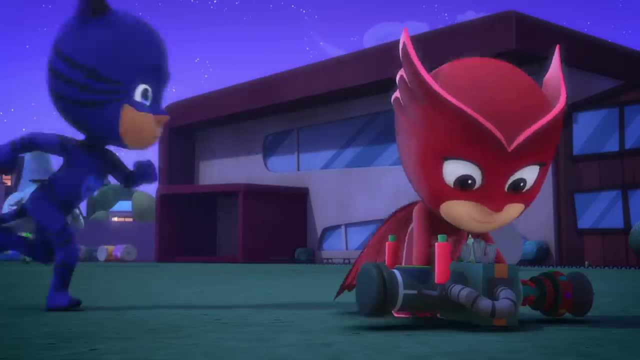 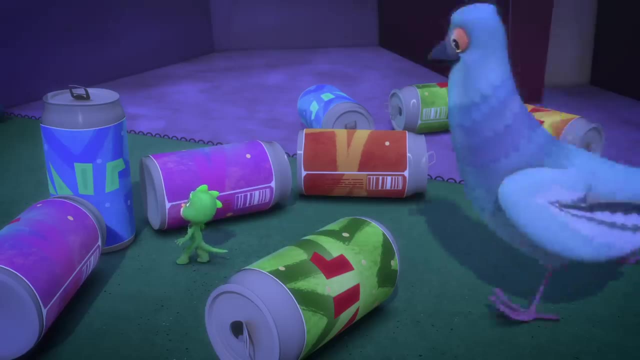 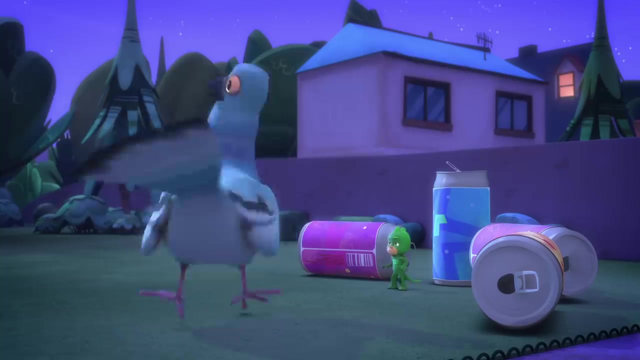 Yeah, Caw, Caw, Catboy, let's catch up with Luna Girl. Nice work, Gecko. Uh-oh, I should have cleaned up this mess too. Super Gecko, Muscle, Huh, Oh, you think this is a game. 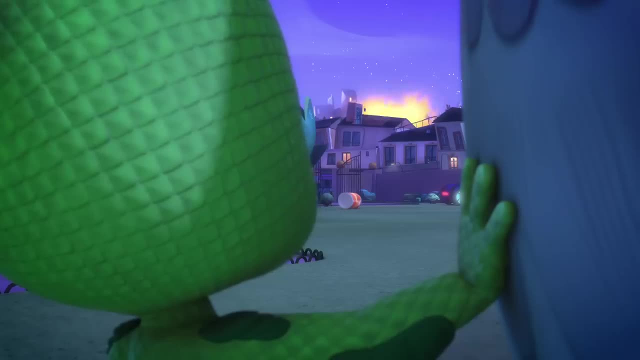 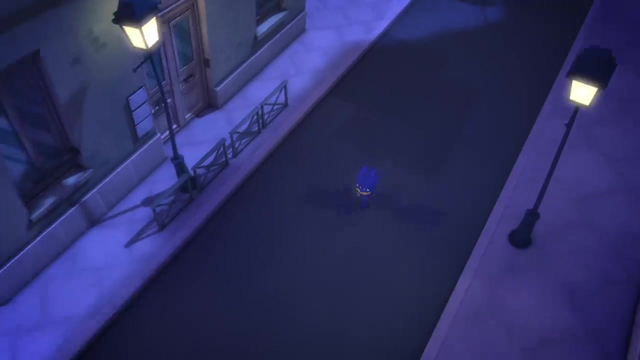 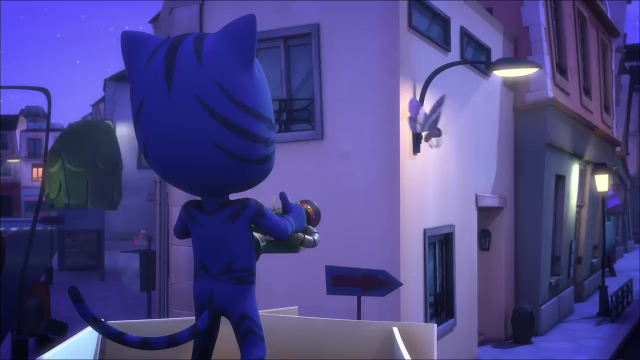 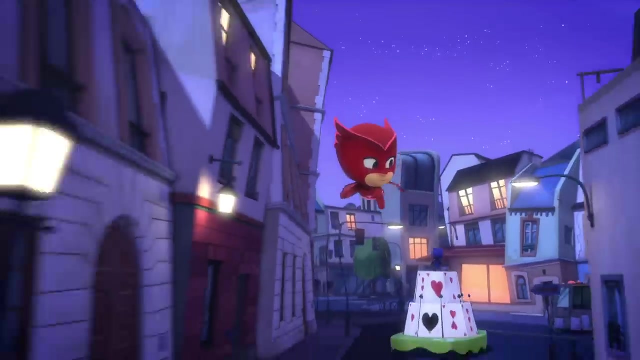 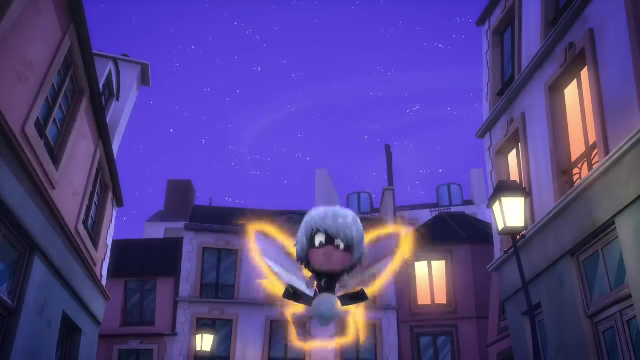 Good bird, Huh, Catboy and Owlette need my help And you've given me an idea. Oh dear Huh Catboy, Super Owl Wing, No, No, No, No, Yes, Yes, Yes. 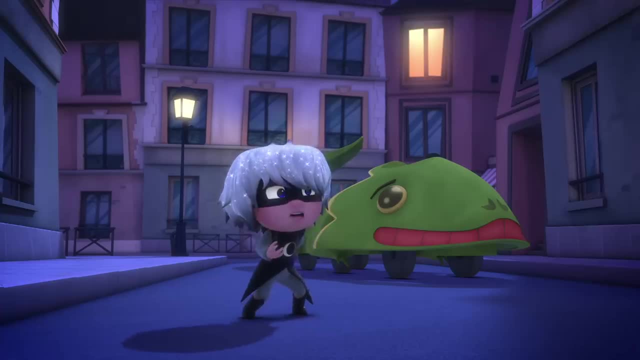 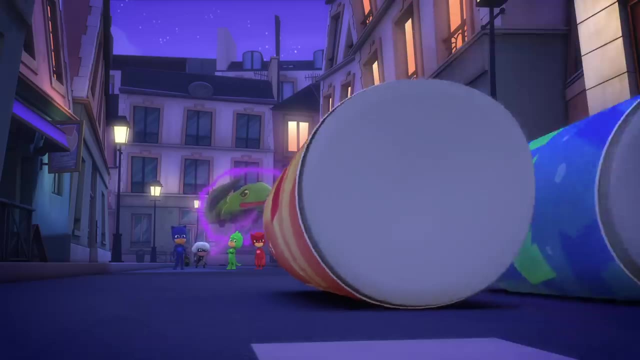 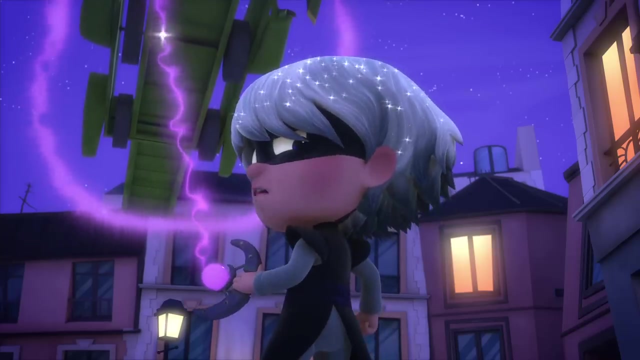 We've shrunk all the mods. Oh, I can't have all the floats, But I can still take your favorite Lizard Boy, Luna Bird. We've got you now. Luna Girl, Think a few cans can stop me. I must have shrunk your brains too. 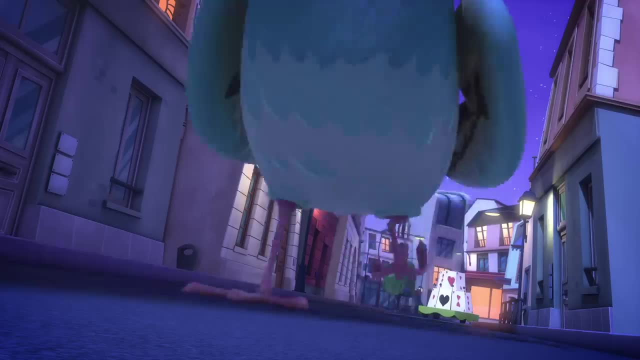 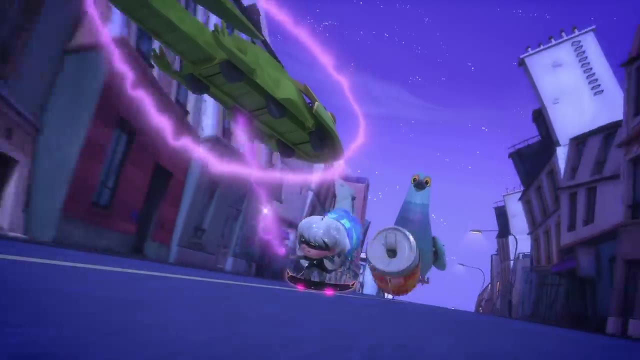 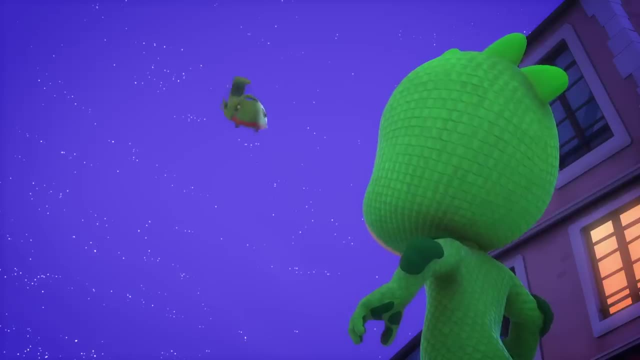 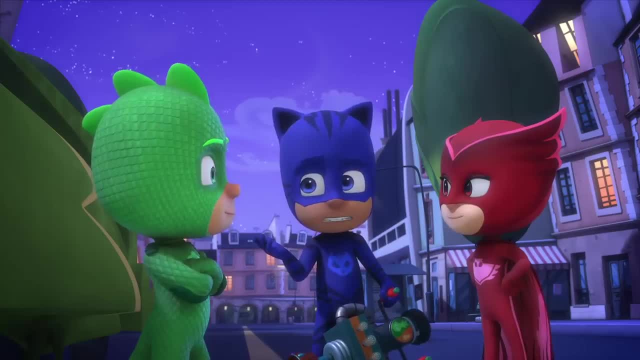 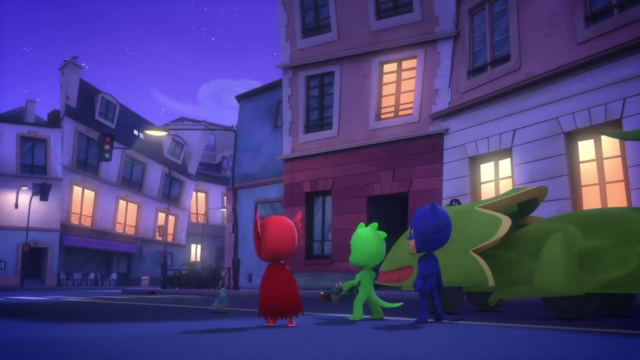 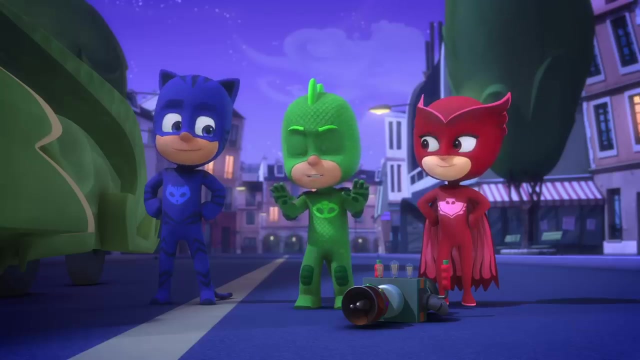 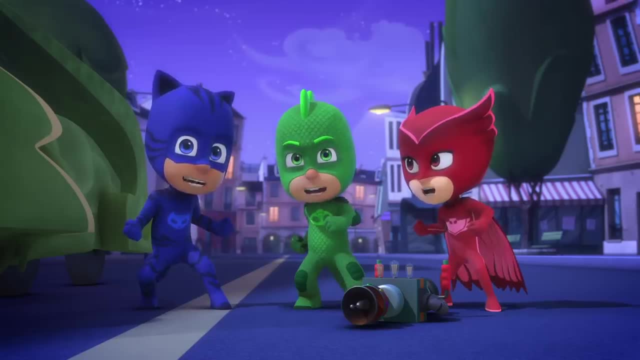 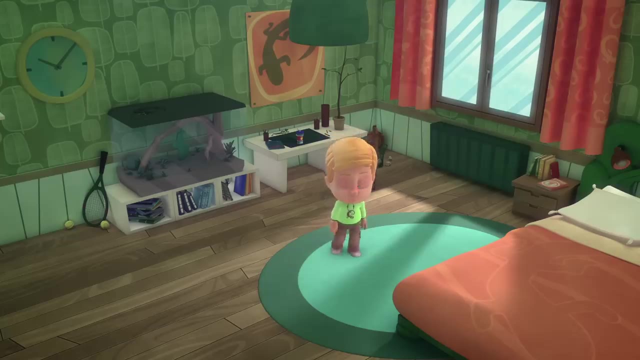 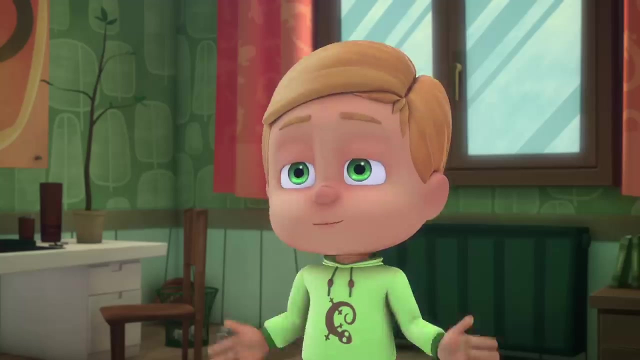 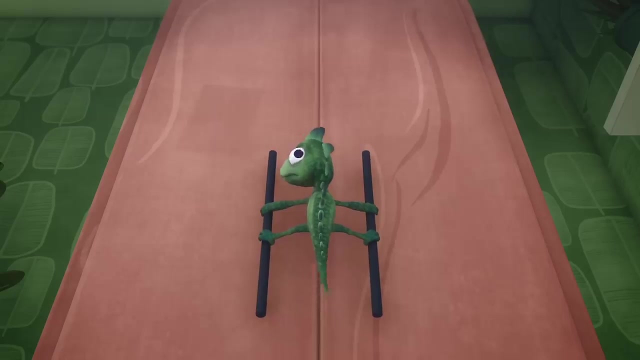 PJ Masks. all shout: array, Cause in the night we save the day. Whoa, It looks great in here, Greg. It took forever, but now everything's put away and I'm ready for the parade. Uh-oh, Get down. 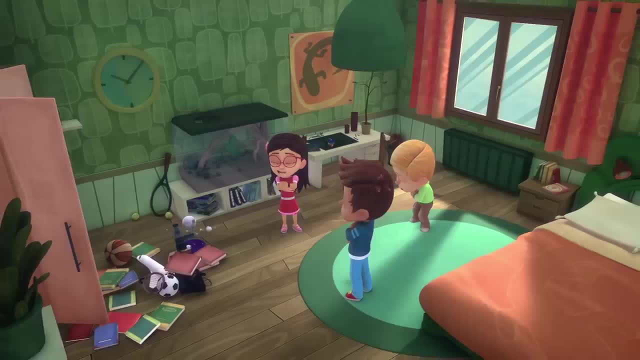 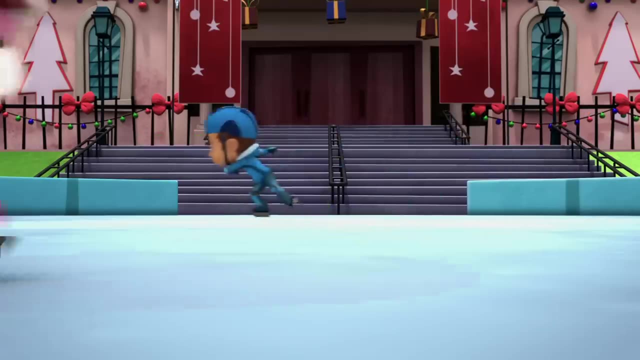 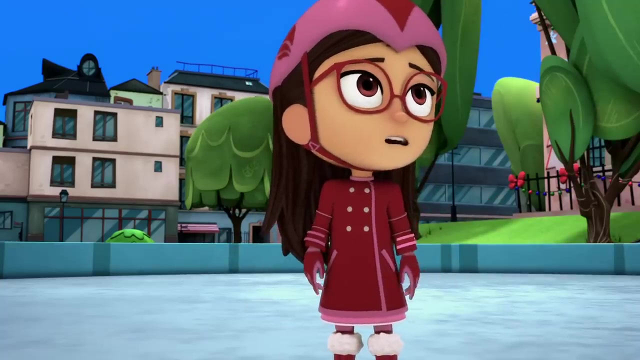 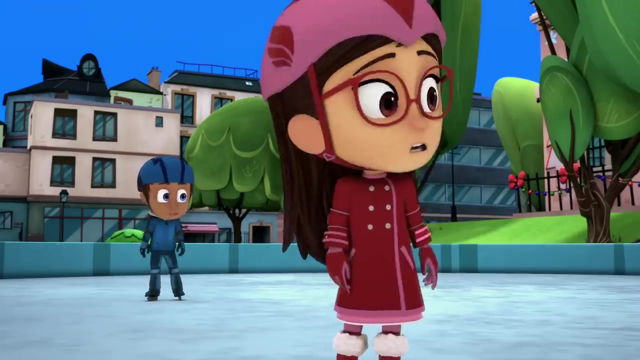 Oh, at least Lionel found my camera. Gecko saves Christmas O'Connor, it's Christmas tomorrow and it still hasn't snowed. Snow would be amazing, but we'll still have a good time. Whoa, I can't do this. 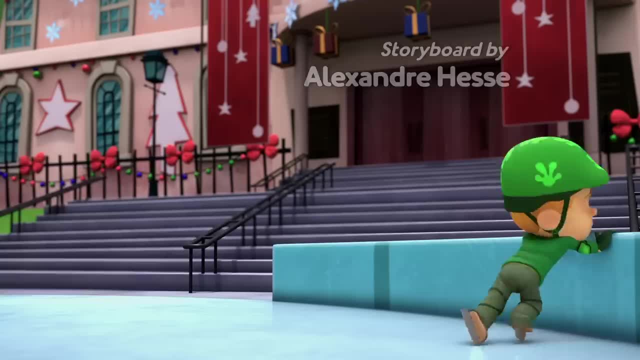 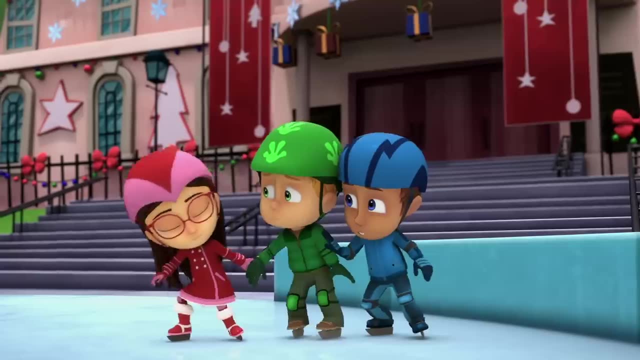 What's wrong, Greg? It's the day before Christmas, Aren't you excited? Not about ice skating? I've never done it before and I'm not any good at it. We'll help you. Come on, just try. It's all part of Christmas, like the tree? 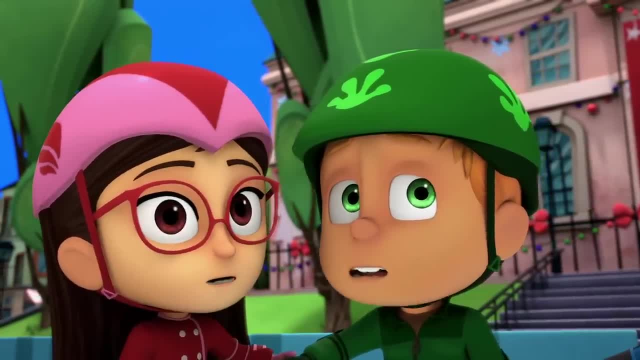 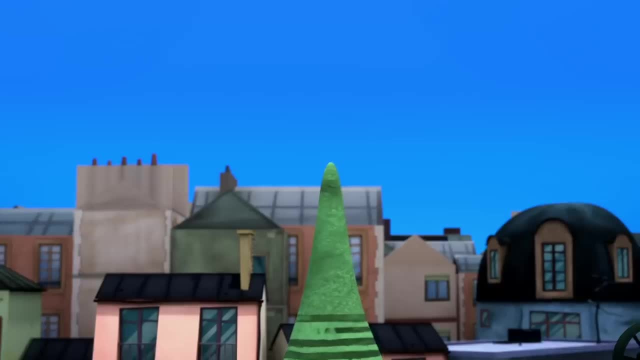 Yeah, with all its lights and decorations. What lights and decorations? Oh no, Where'd they all go? Where are all the ornaments And the tinsel? Even the star has disappeared. Oh, They were so beautiful And there were so many. 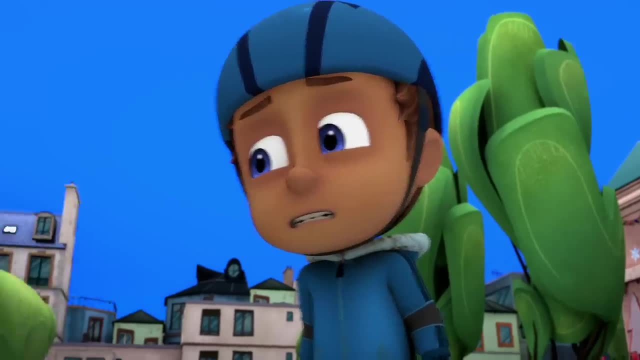 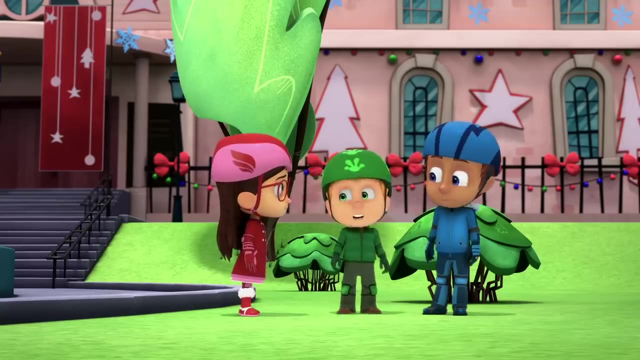 They can't just be gone. Someone must have taken them last night, But how did that someone get up there? It's so high. We're going to find out, And we won't need ice skates to do it. PJ Masks, we're on our way. 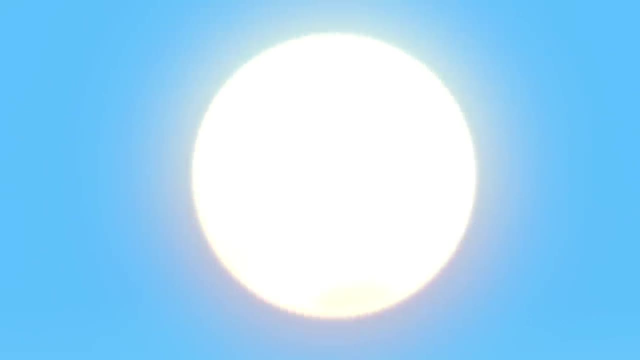 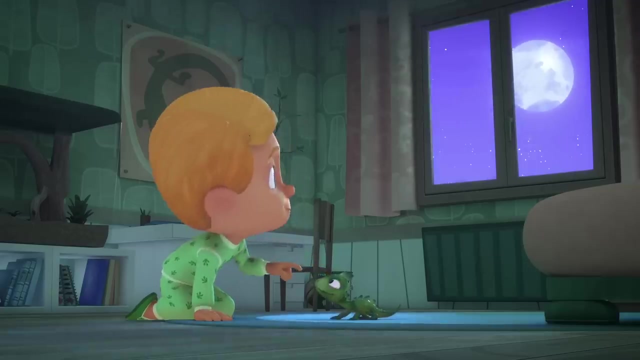 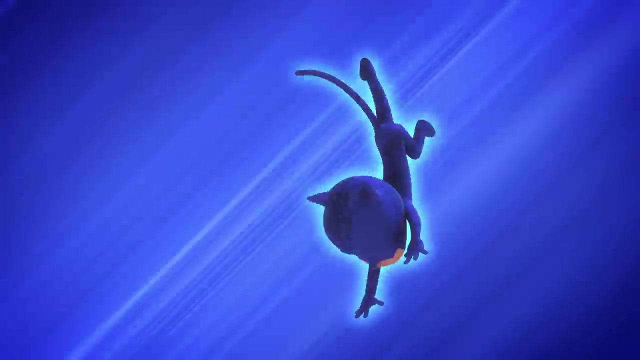 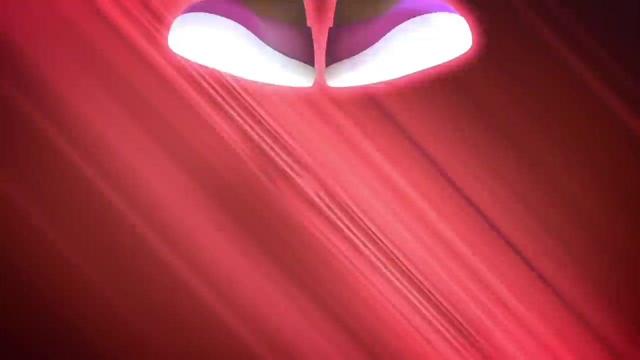 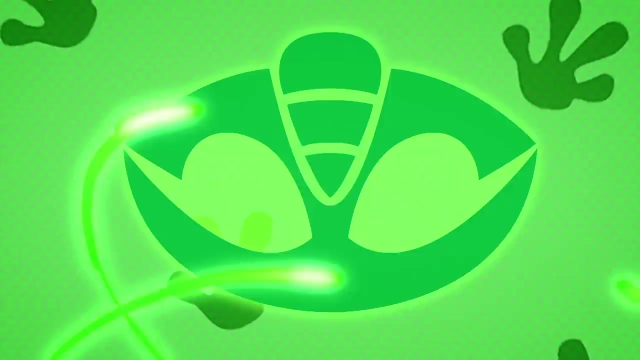 Into the night to save the day, Night in the city, And a brave band of heroes is ready to face fiendish villains to stop them messing with your day. Connor becomes Catboy, Amaya becomes Owlette- Yeah, Greg becomes Gekko. 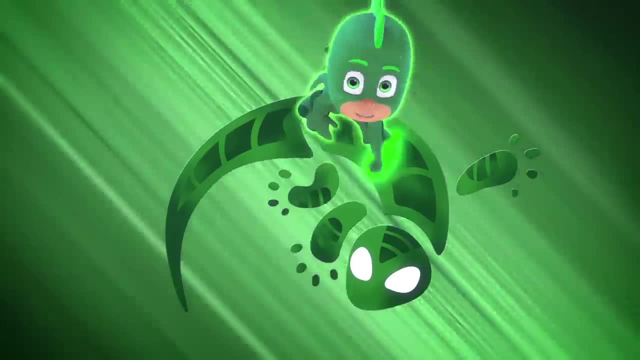 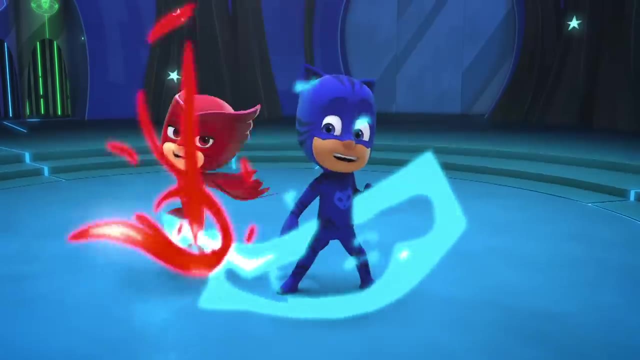 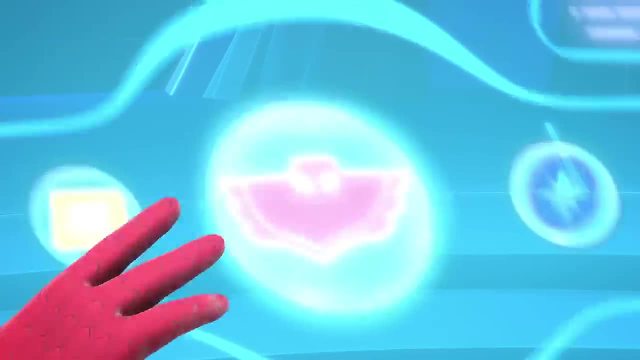 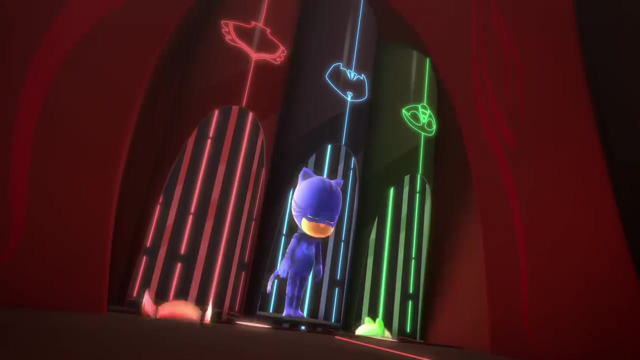 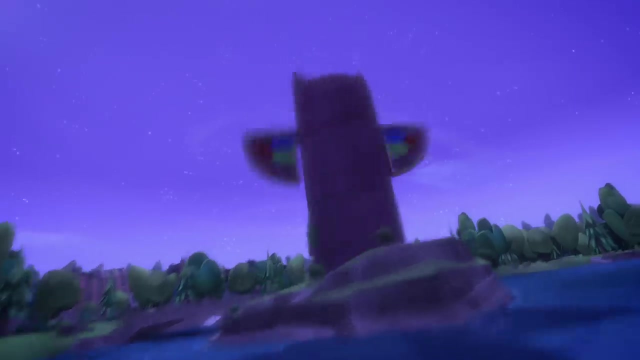 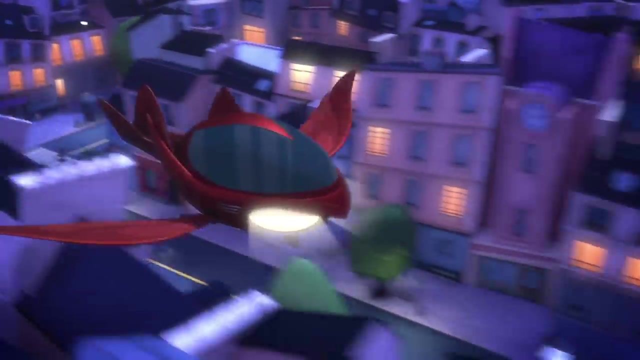 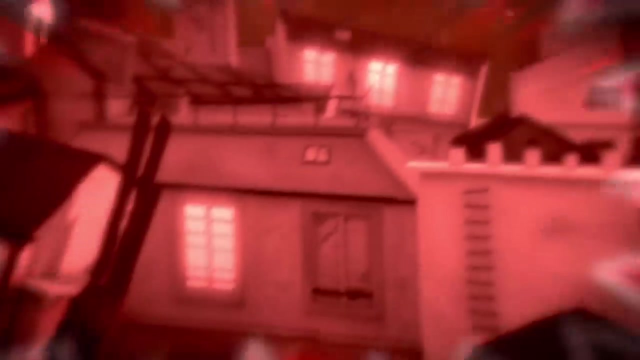 And we need to get up high too. Come on to the owl glider. Look, It's Luna Girl Gasping Gekko. she's taking everyone's presents. It's Christmas Day tomorrow. No one will have anything to open. 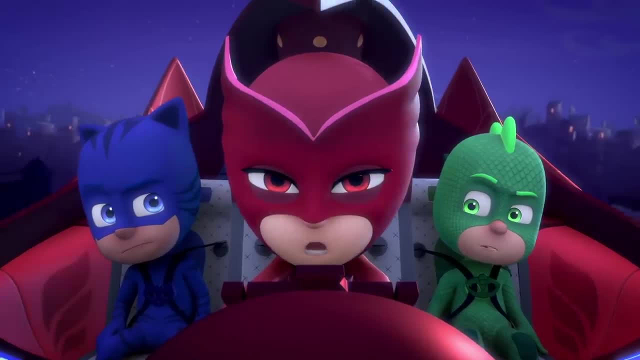 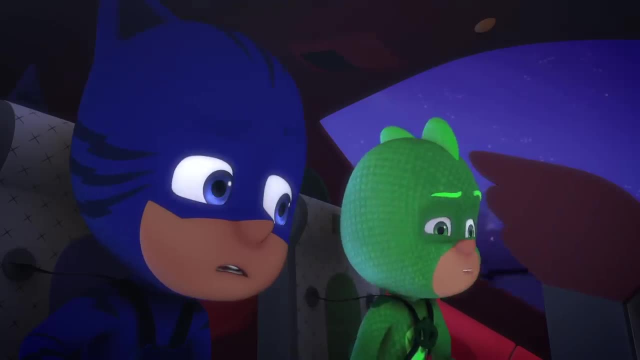 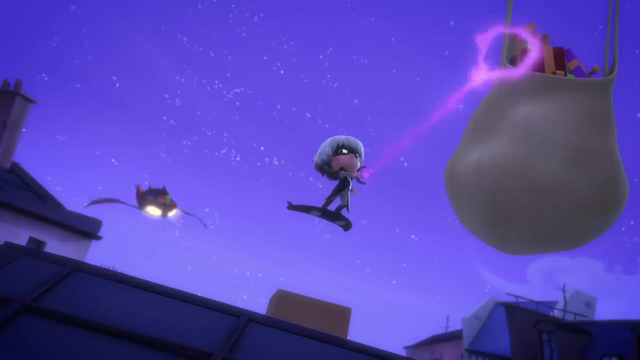 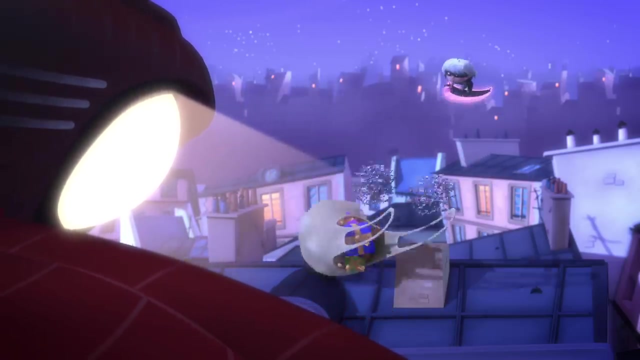 Oh, Oh, Oh, Oh, Oh, Oh, Oh. No one will have anything to open. Luna Girls, give those presents back. They don't belong to you. Forget it. Goodie, Goodies, They're mine. Christmas is all for me. 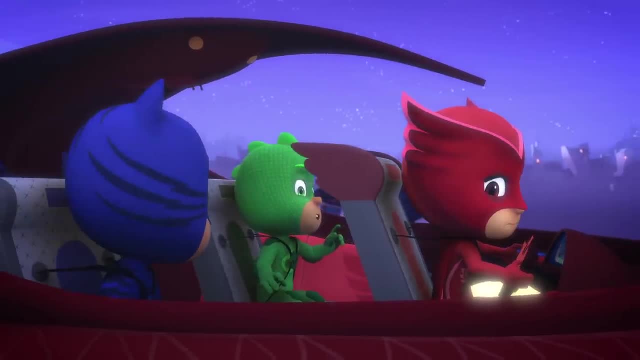 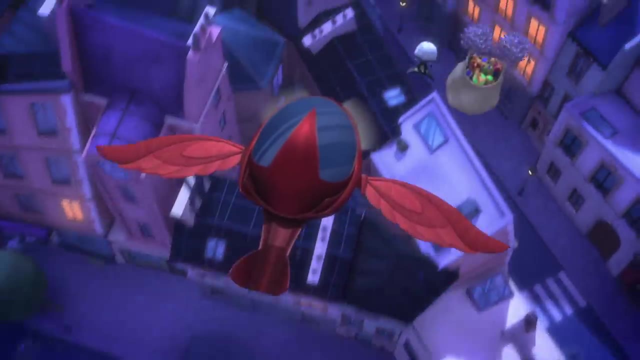 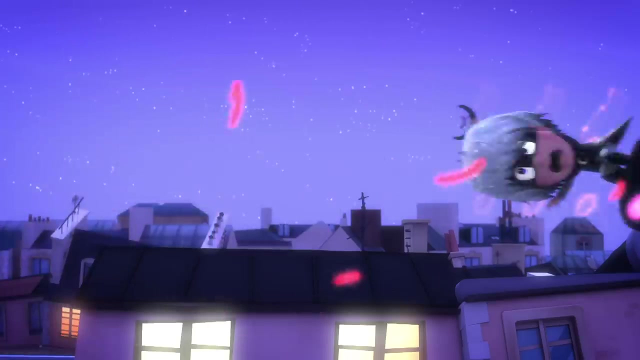 Me, Me, Hey, if we could get her Luna Board, she won't be able to reach the chimneys. Good idea, Gekko, Let's go, I'll get her down to the ground. Owl wings, Oh, Oh. 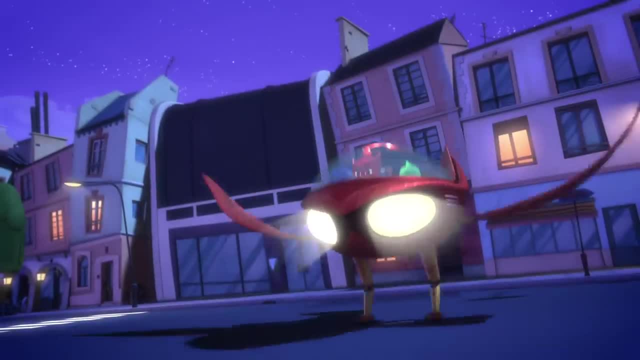 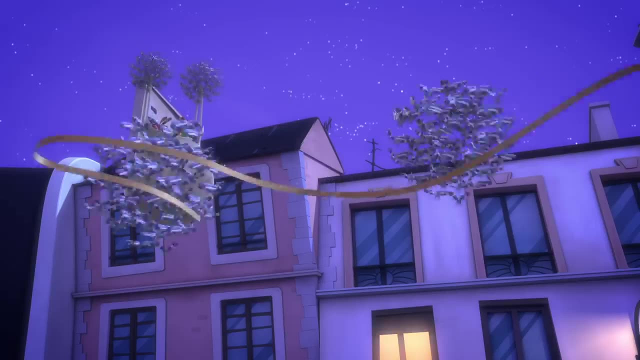 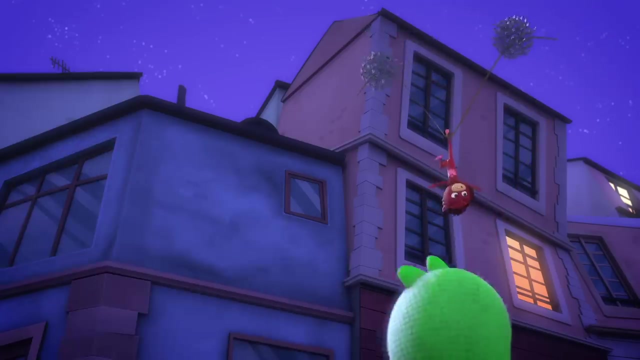 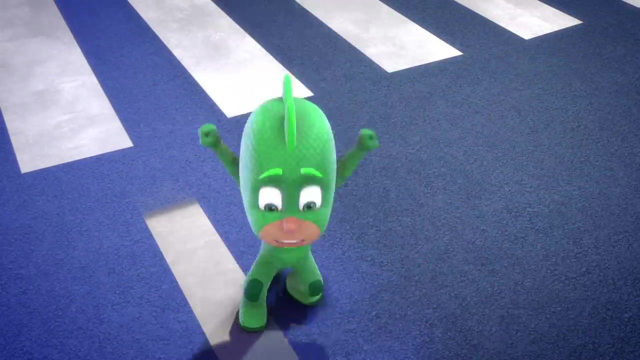 Oh, Ah, Owl wings, look out Quick, Gekko, Fly the Luna Board away from Luna Girl. But I've never ridden a Luna Board before. I won't be able to do it. Huh, So long, Kitty. 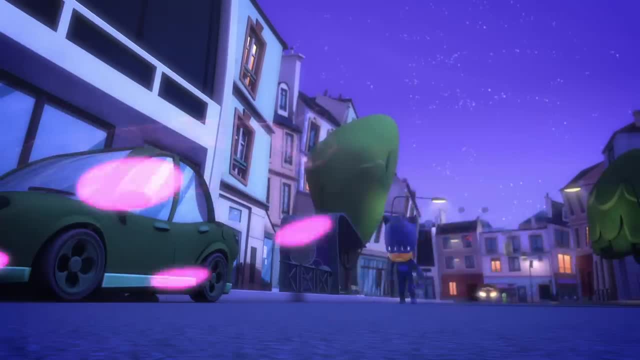 I'm out of here. Whoa Gekko, are you okay? Yes, I knew I wouldn't be able to fly the Luna Board. Sorry, It's okay, Let's just go after her. The Owl Glider's too big to chase her down there. 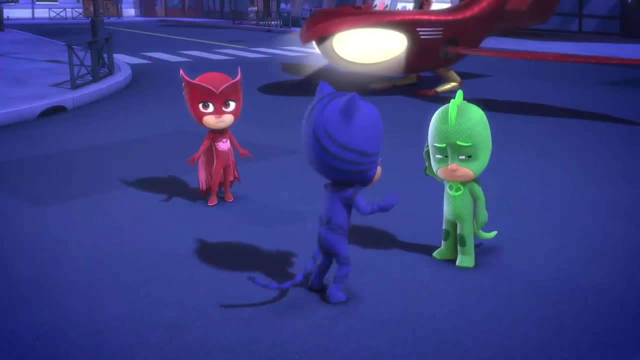 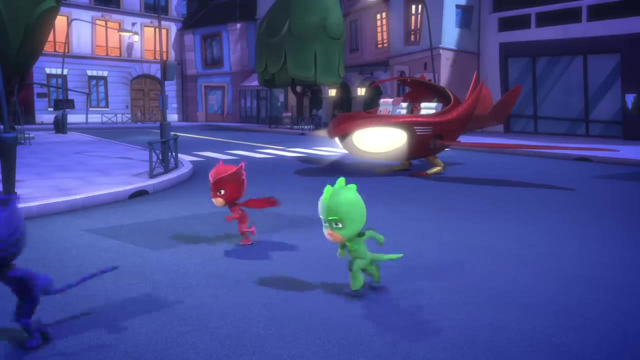 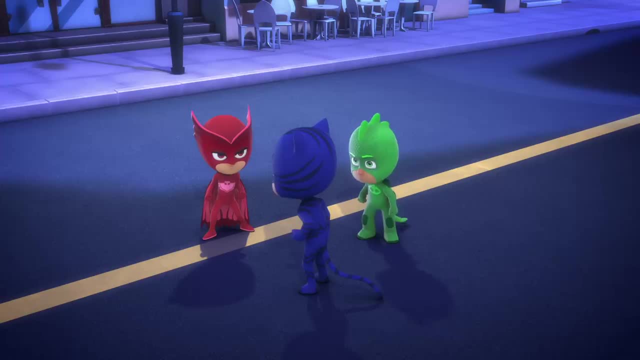 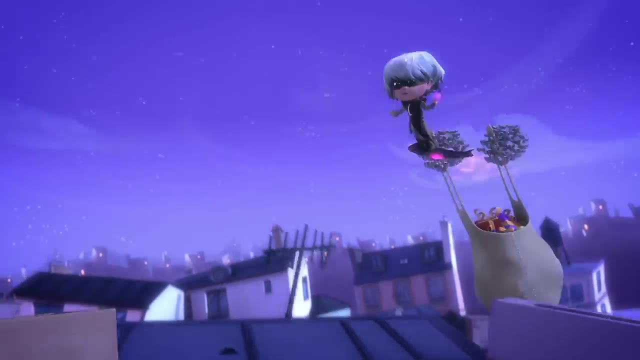 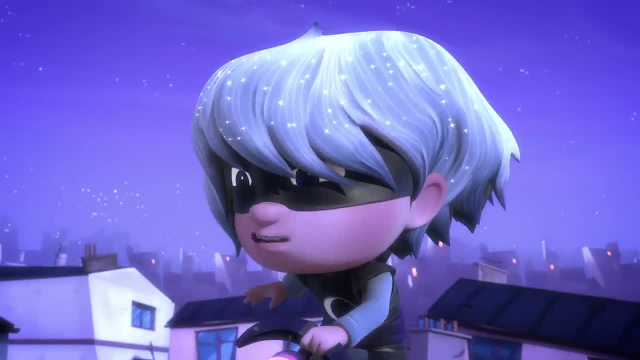 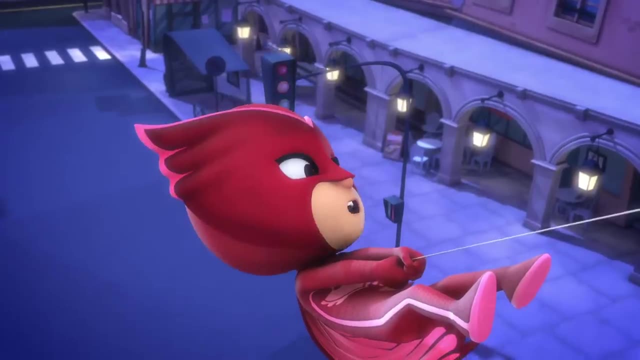 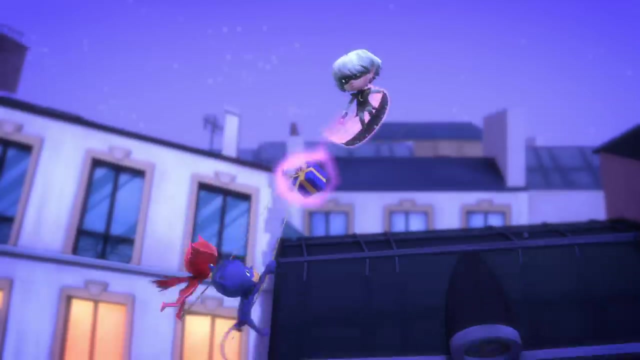 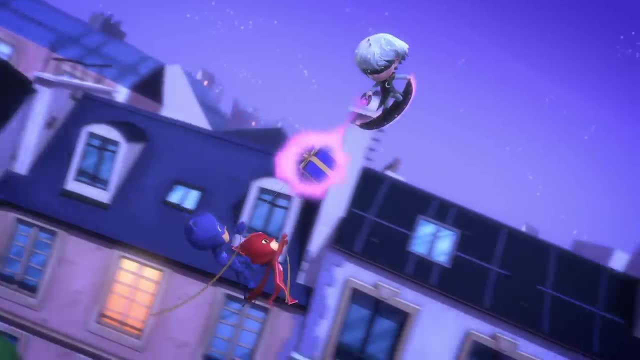 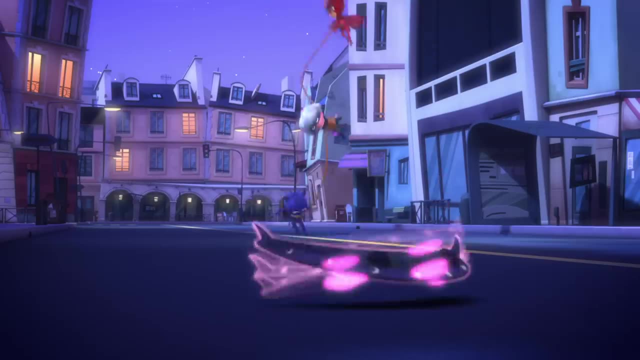 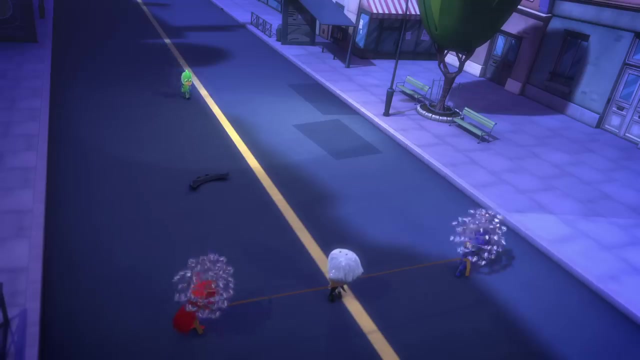 Well, let's see if cats really do land on their feet. Catboy Mom: Huh, Shoo, Shoo. No, I'm coming, Gekko, hop on the Luna Board and get it out of here. Get on it again, But I'm no good. 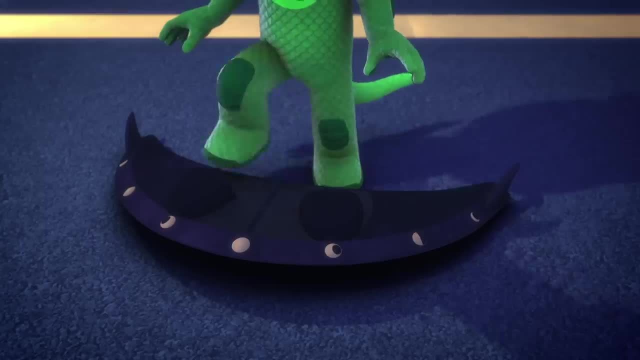 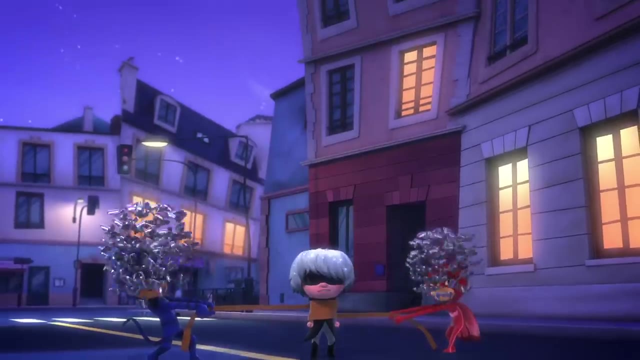 Go on, Gekko. I bet you will be if you just give it a try. Whoa, slithering serpents. This is even harder than ice skating. No way I can't do this, Gekko. 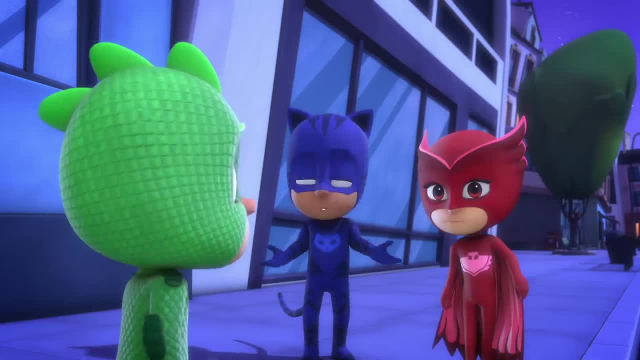 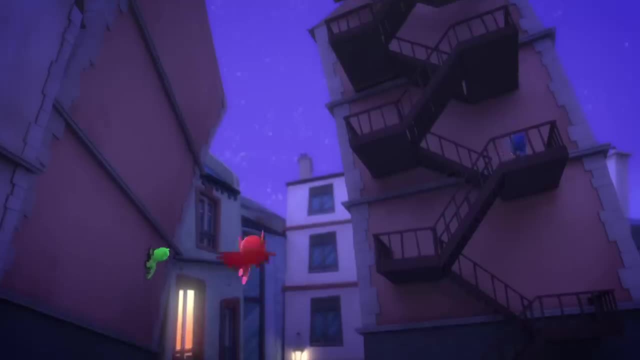 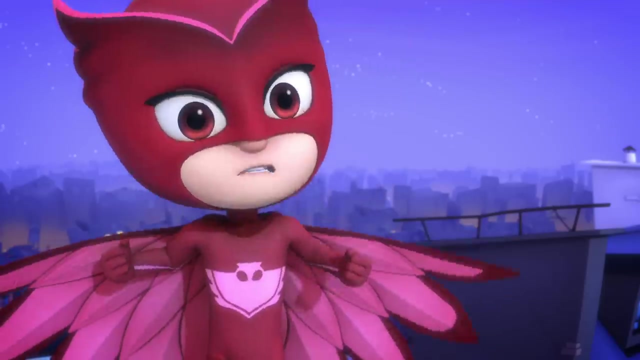 Are you okay? I'm no good at new things. Okay, don't worry, I'll let Nell take care of it. Let's catch up with Luna Girl. Ha ha ha. That's it, Luna Girl. Time to stop. 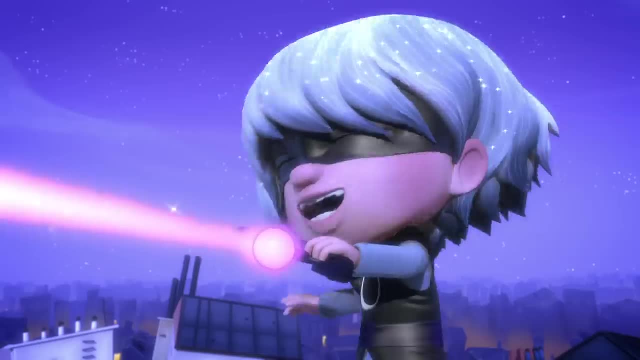 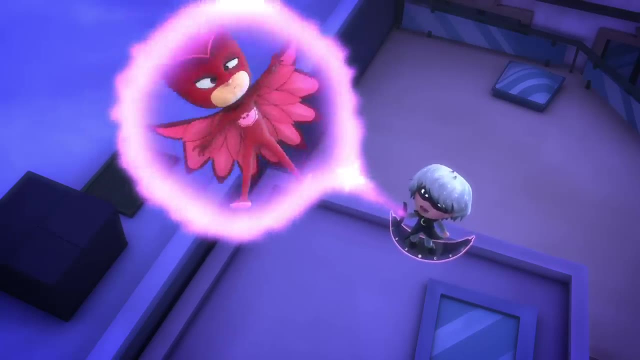 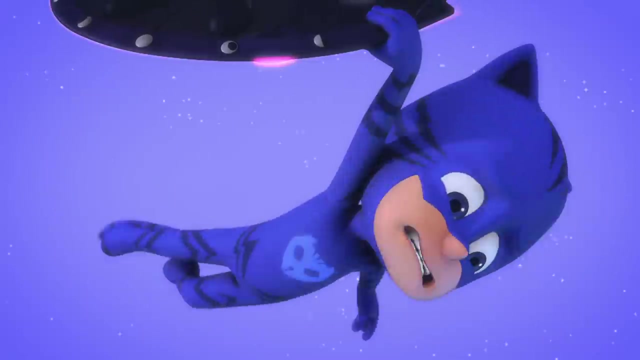 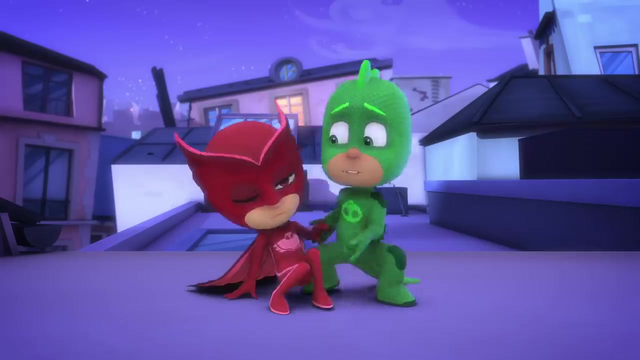 Time to stop you. you mean Slithering feathers Owlette? Did I ruffle your feathers Owlette? Sorry, Super Ken-ju Gekko, help Get off my Luna Board Owlette. what do we do? 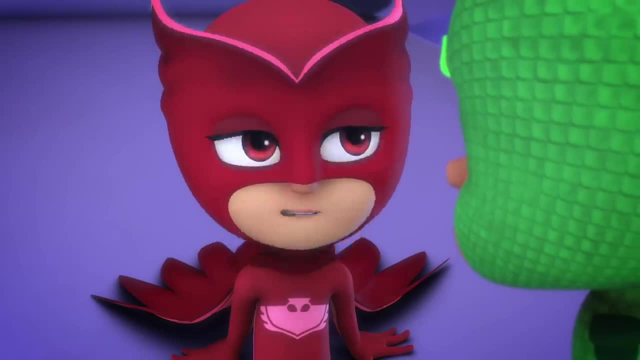 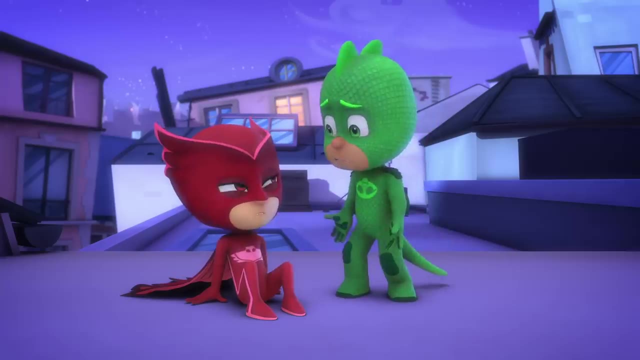 I'm too dizzy to do anything right now, Never mind fly straight enough to help. You need to jump on the Luna Board again to help Catboy Again, But I'm no good at riding it. You don't know if you're any good at it because you keep jumping off. 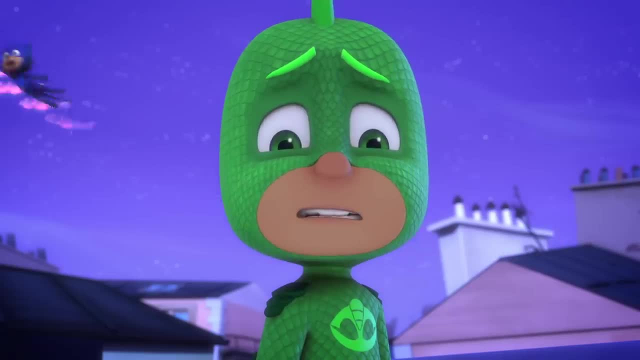 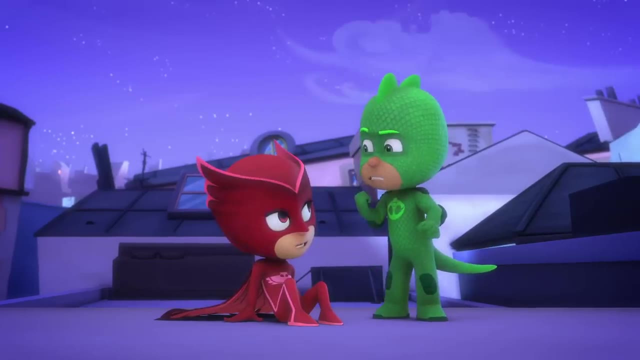 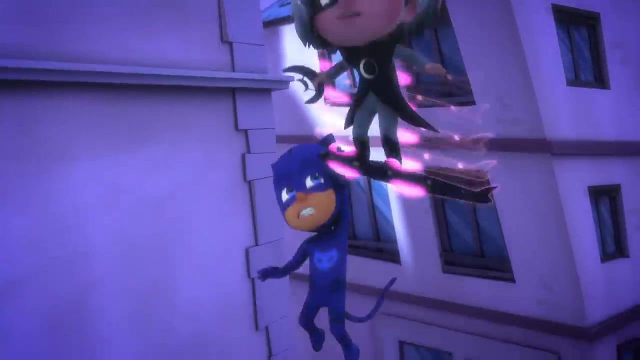 You need to really try. You can do it. Help Catboy. You're right, Owlette. I've got to at least try to save him. It's time to be a hero. Super Gekko camouflage. Where'd that loopy lizard disappear to? 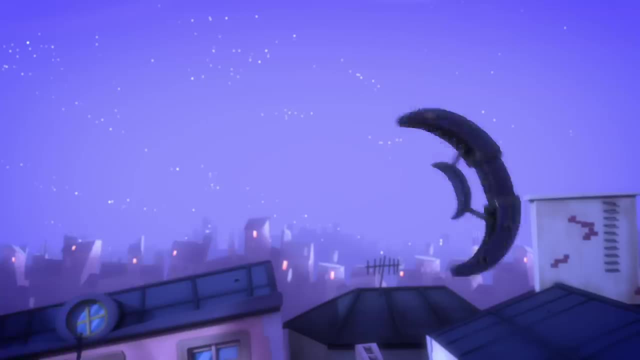 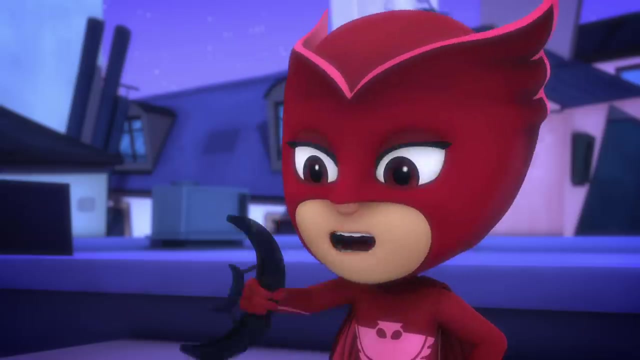 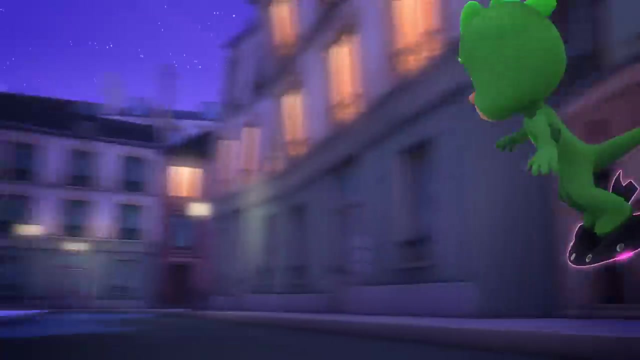 What? Where'd you? Ow, Huh, Whoa, Ah, Hey, Thanks, That's mine, Whoa, Hang in there, Gekko, You can do this. Ah, Gekko, I'm losing my grip, Pull me up. 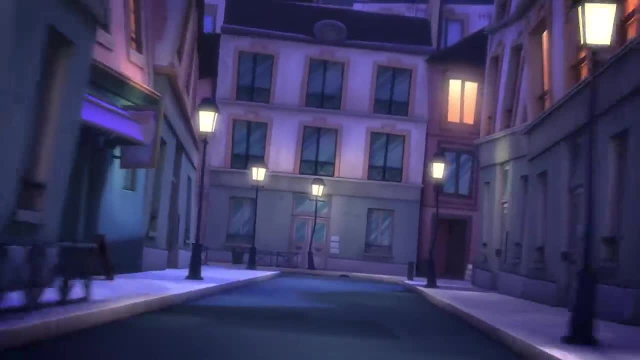 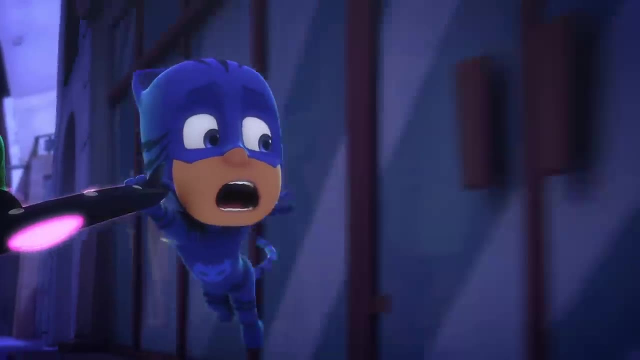 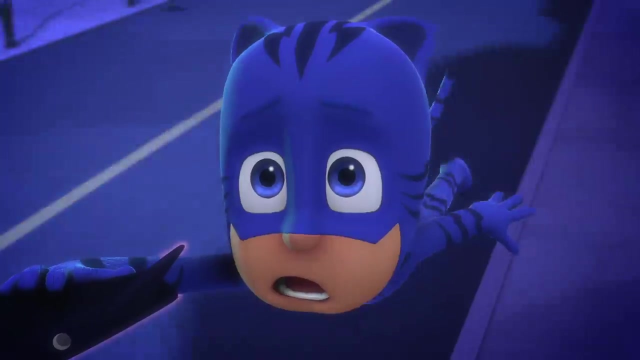 Whoa, But if I bend over I lose my balance. Hang on, I'll get you safe, I promise. I just have to stay on and try to fly this thing. Ah, Gekko, Look out. Whoa, This is kind of cool. 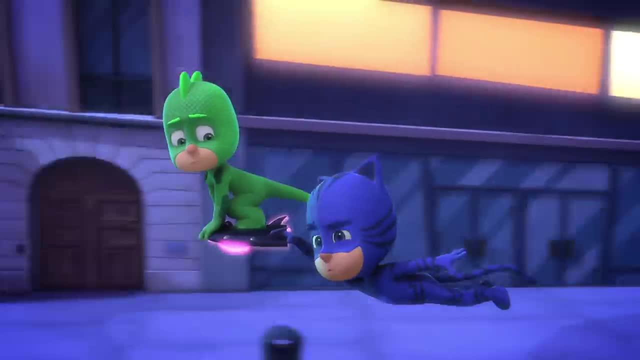 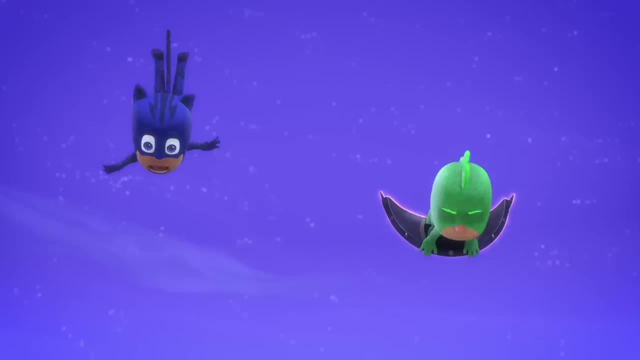 Whoa, But ours. I've got to keep going. Watch out for the wall. Yeah, Wriggling reptiles, We're too high. Ah Ah, Ah. Don't panic, Gekko, or we'll crash. 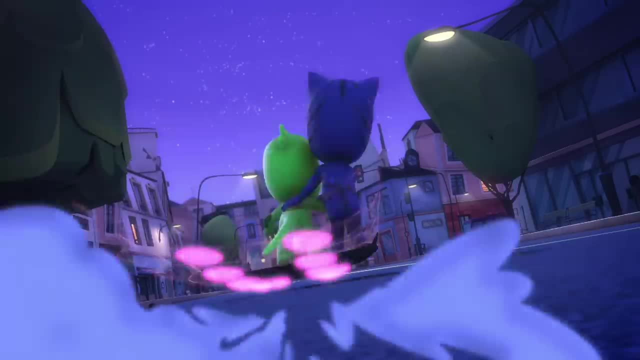 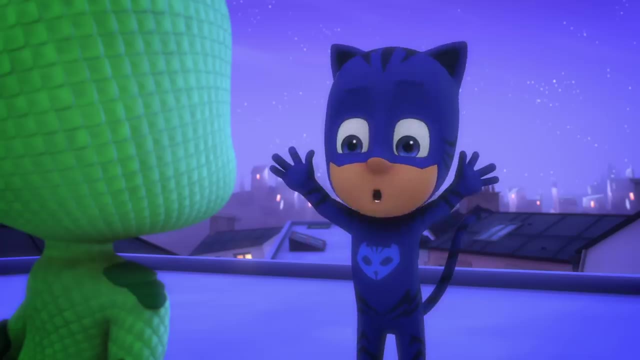 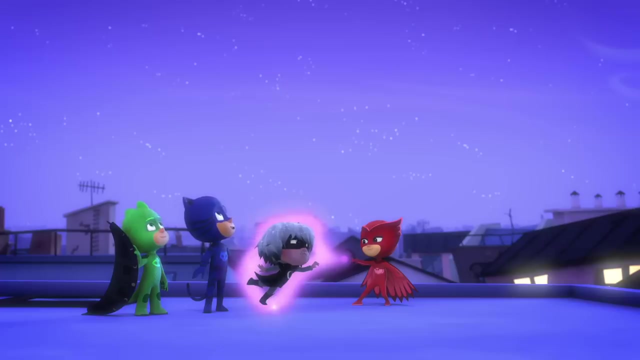 Right, Careful, Whoa. Yes, I'll just bring you down slowly, Way to go. I knew you'd get the hang of it. See, You just had to give it a try. Yeah, Mutts, Let me go. you PJ pests. 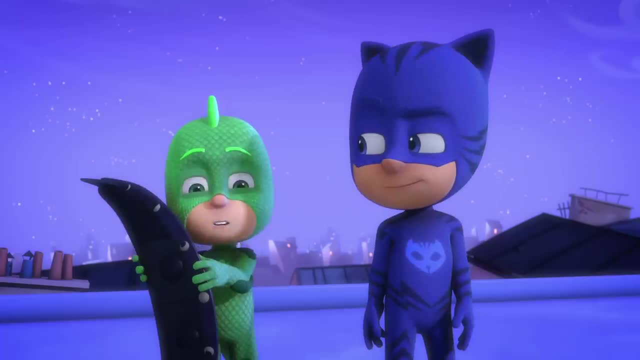 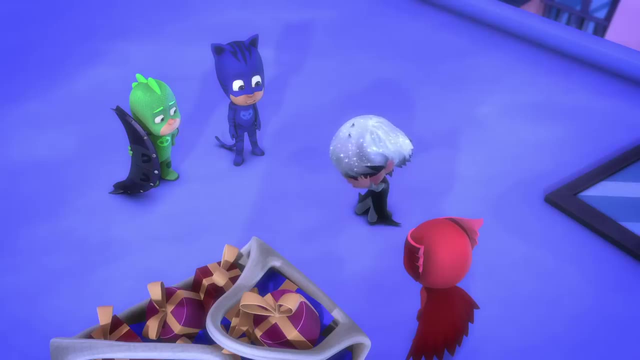 It's over. Luna Girl, Yeah, we've got your Luna Board, So you can't steal any more presents. Oh, Oh, it's not fair. I never get a real Christmas. I'm just here by myself. What You mean? you're all alone at Christmas. 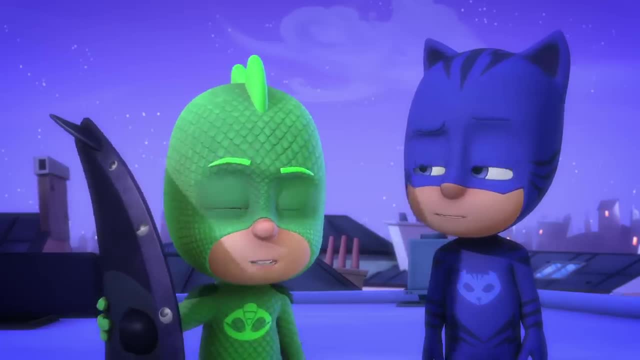 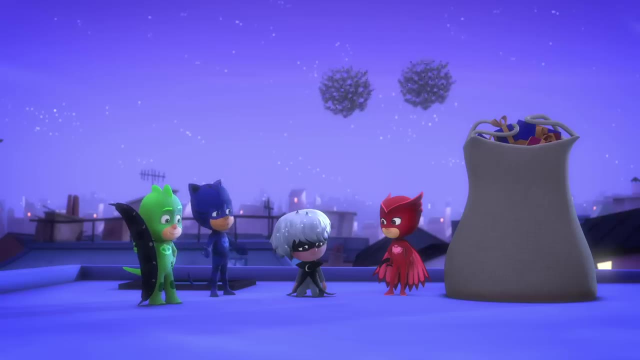 But that's really sad. Hey, why don't you spend the rest of Christmas Eve with us, With you? Yeah, We've got to put all these presents and decorations back. anyway, You can help, Then we'll all have Christmas together. 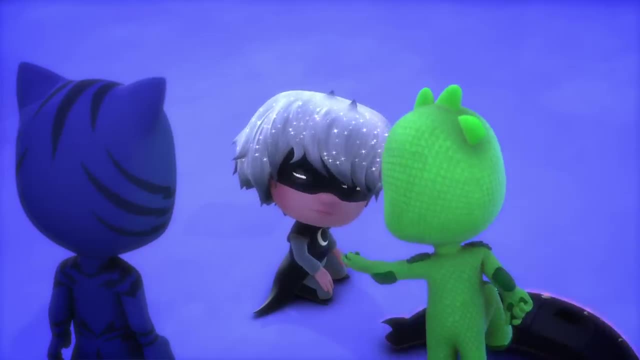 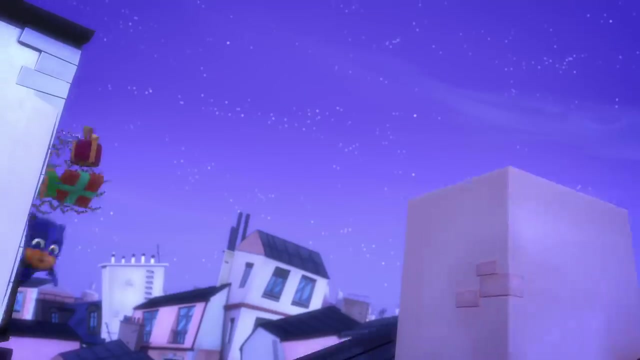 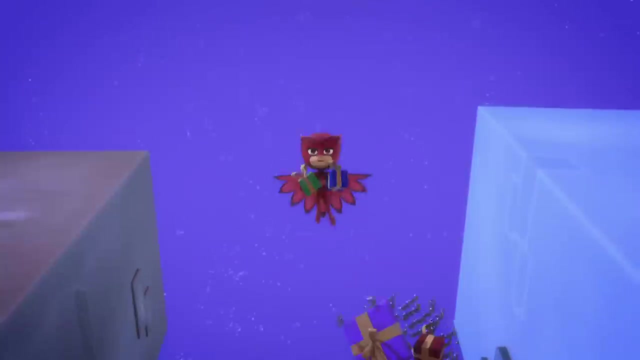 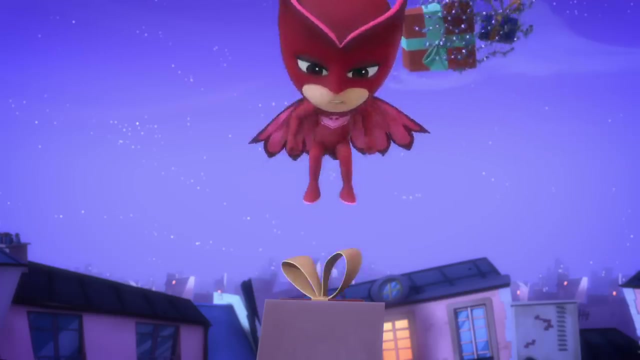 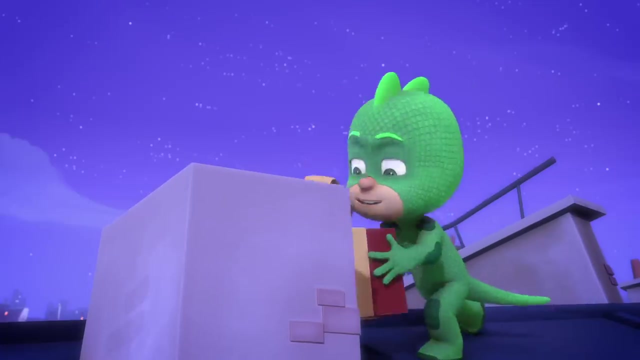 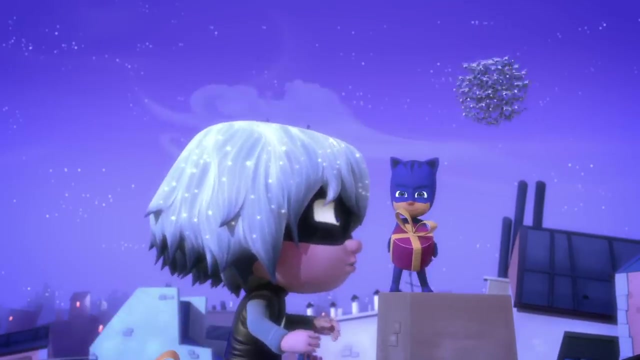 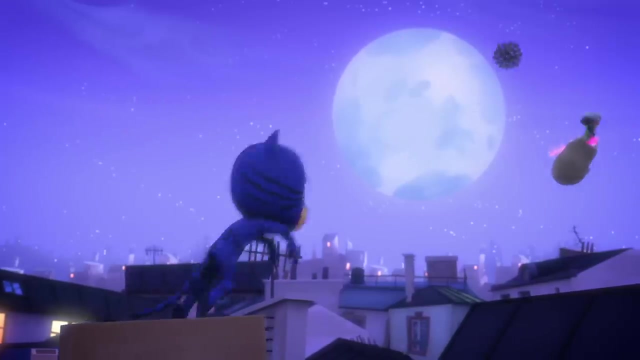 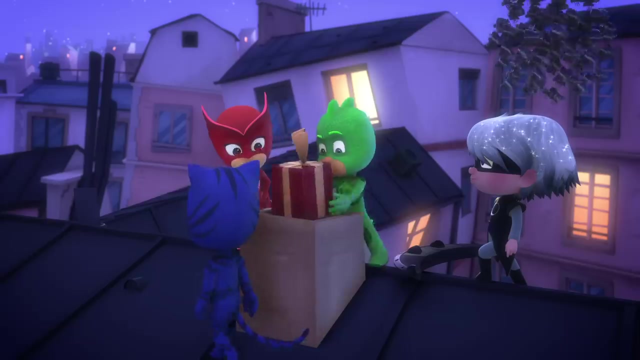 What do you say? Okay, I guess. Then hop on, We're going to save Christmas, Yay, Oh, And now for the last one. Excellent, And you're getting so good at riding the Luna board, Gecko, Thanks. 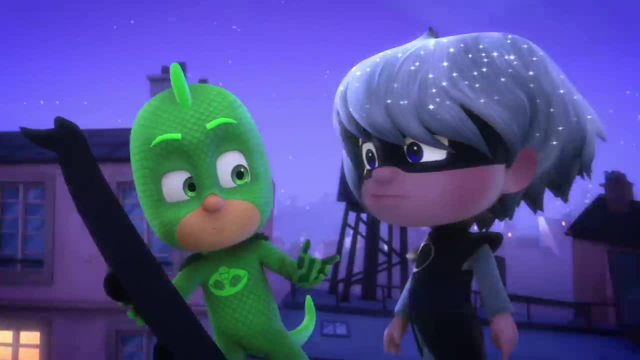 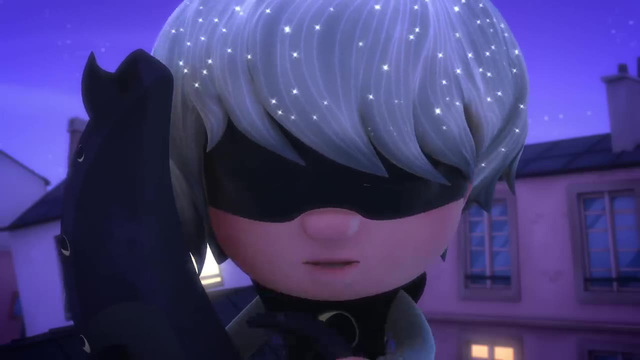 Now that I have the hang of it. I love it. You really helped us out, Luna Girl, so you can have your board and magnet back. Okay, But I guess you have to go now. so Christmas is over for me, Don't worry. 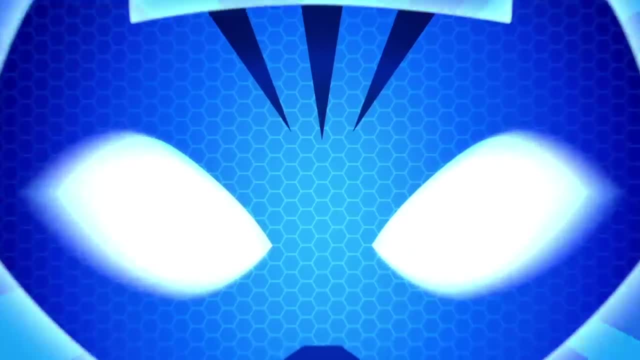 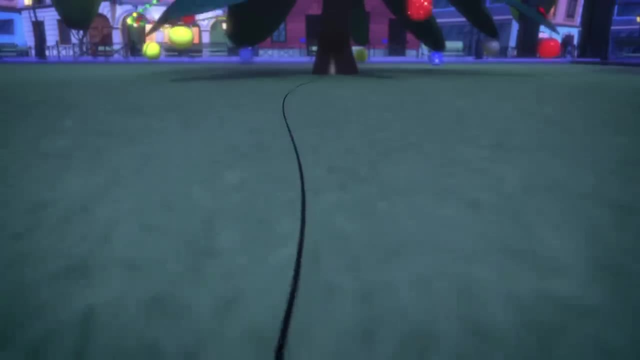 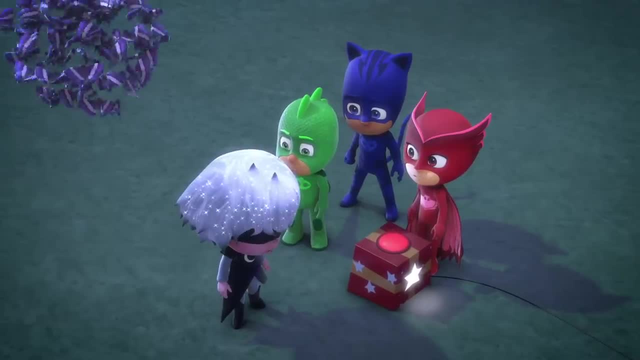 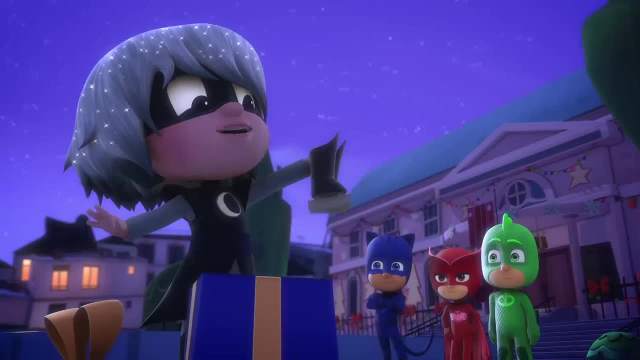 I guess. But now Christmas really is over and I didn't get any presents. Oh yes, you did Ice skates, But I've never skated before. That's okay. Neither have I, But we'll get the hang of it. 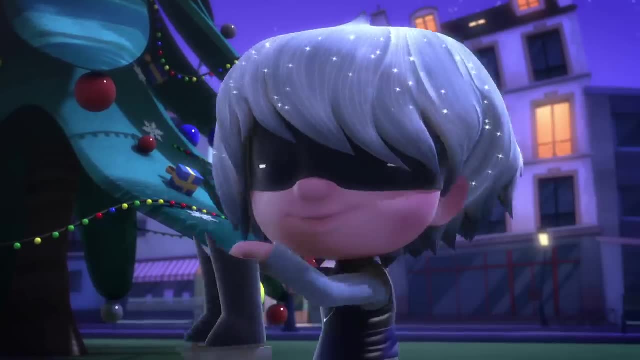 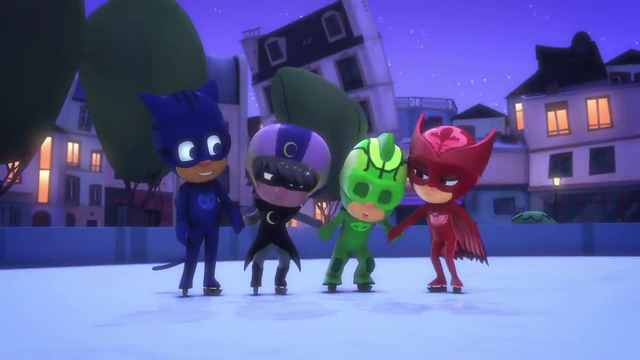 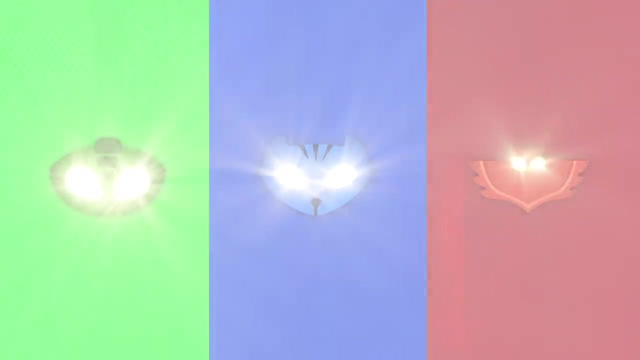 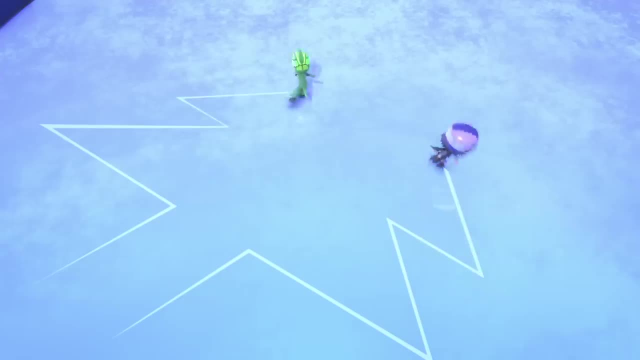 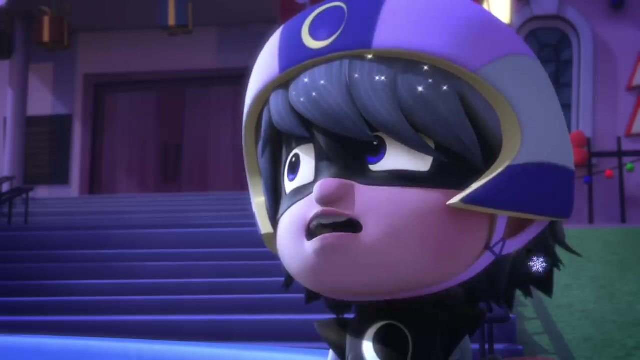 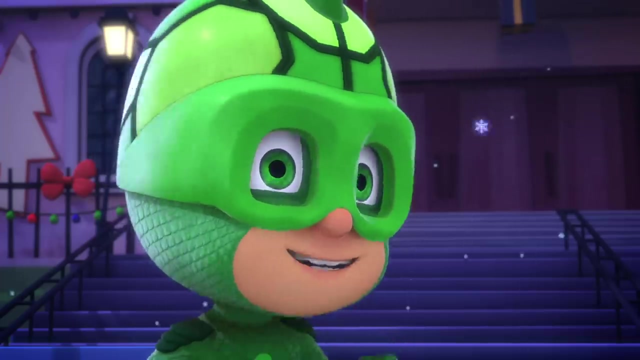 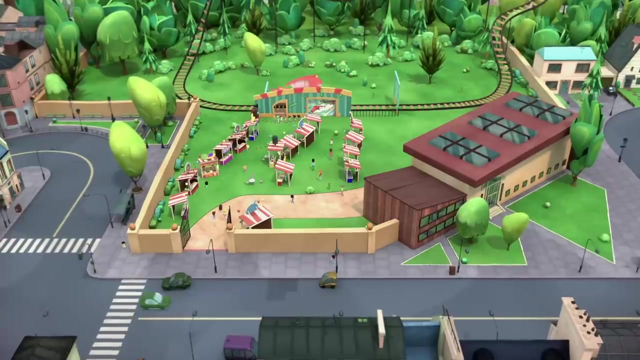 Woo-hoo, Yeah, Whoa, Huh, Hey. what's happening? It's snowing, Snow for Christmas. Catch a snowflake on your tongue, Ha-ha-ha, Blame it on the train, Owlette. 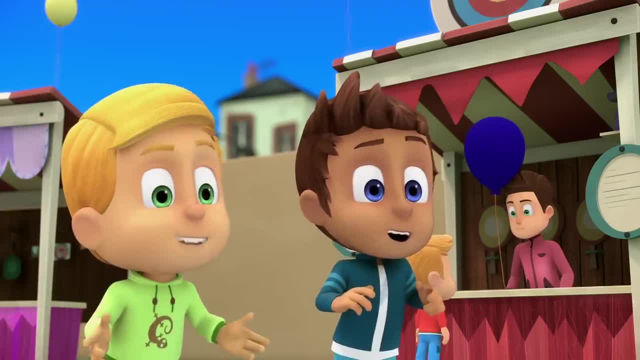 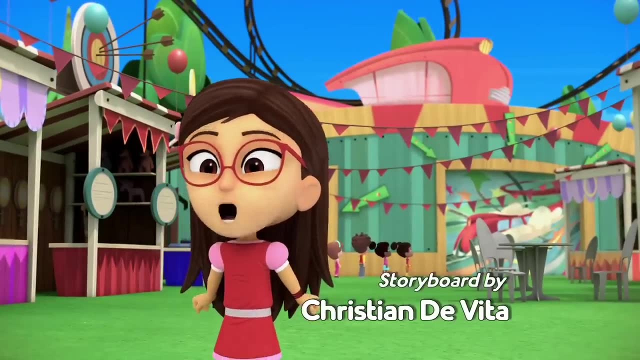 Let's go, let's go, let's go. Why are you so excited, Amaya? Because the fair's got an amazing new ride: The Fairground Flyer Train. I saw them testing it yesterday. It was so fast it's going to feel like flying. 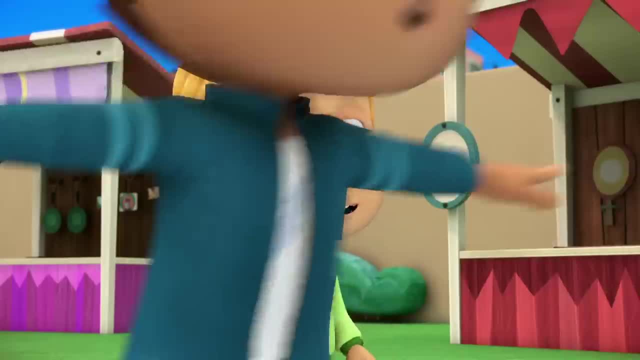 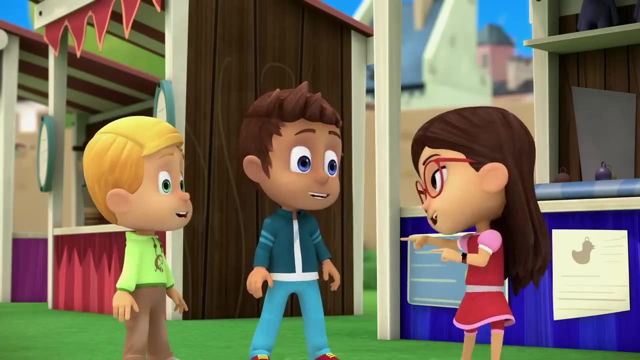 You know I like going fast: Zoom, zoom, zoom. Wow, everyone wants to ride this thing Because it's the Fastest ride in the world. Come on, you have to check it out. Hey, We were here first. 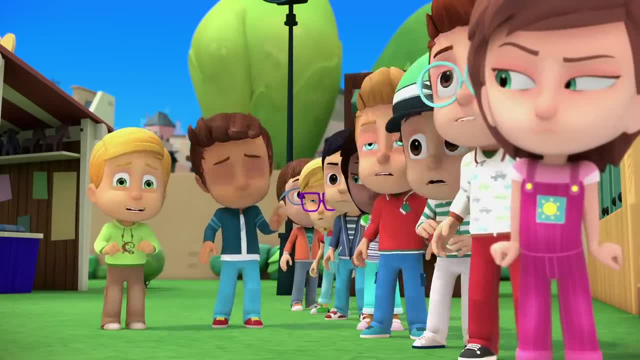 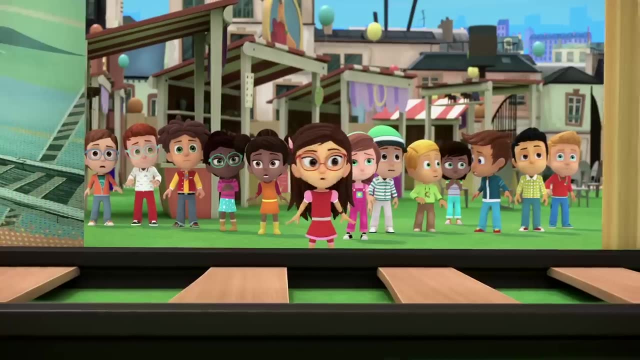 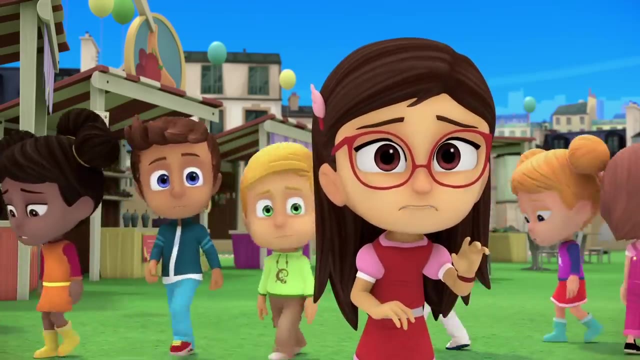 Get in line. Um Amaya, Ladies and gentlemen, boys and girls, the Fairground Flyer Train is now Gone. Where's the train? Huh, It can't be gone. Ugh, I was so looking forward to flying. 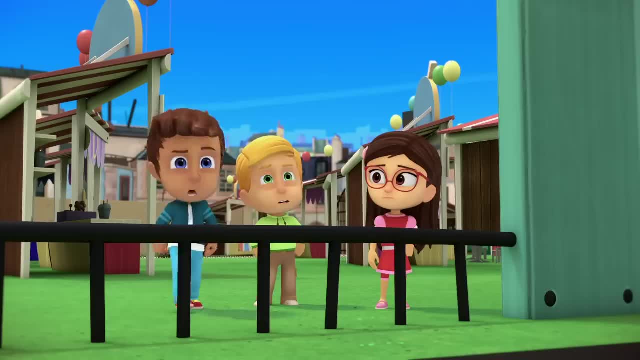 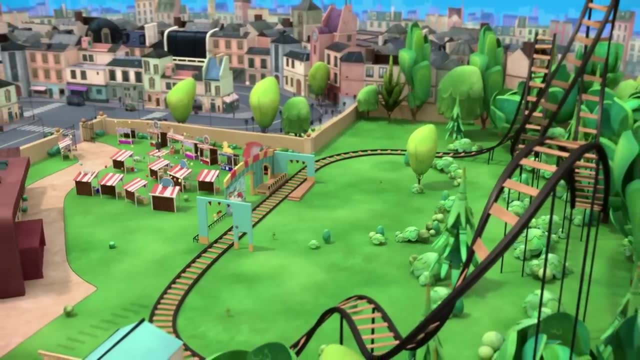 But how can a big train disappear? Uh, trains run on tracks, right. Well, there are twists and loop-de-loops, but this track is still a closed circle. So how could it get off its track and keep going? Look. 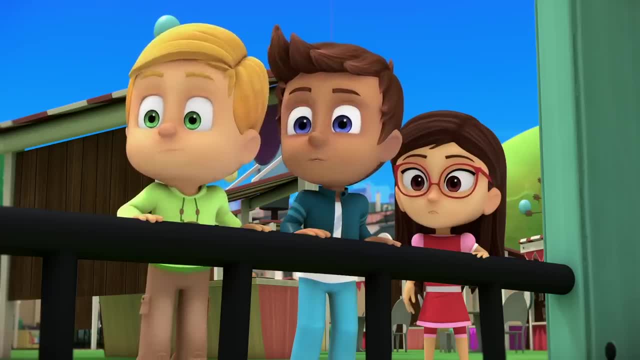 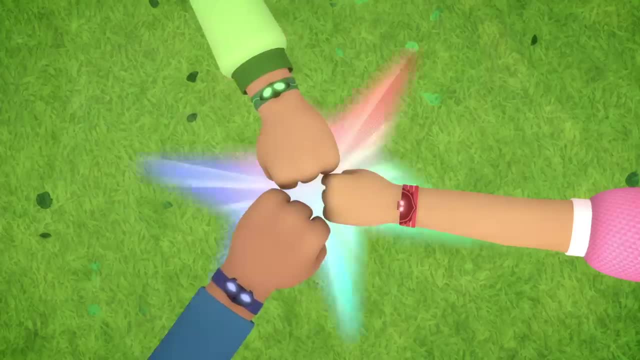 It's like there were more train tracks, but now they're gone- Train tracks that disappear. It has to be a nighttime villain: PJ Masks. we're on our way Into the night to save the day, Night in the city and a brave band of heroes. 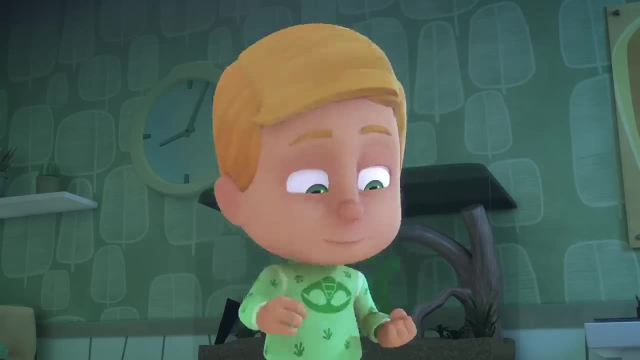 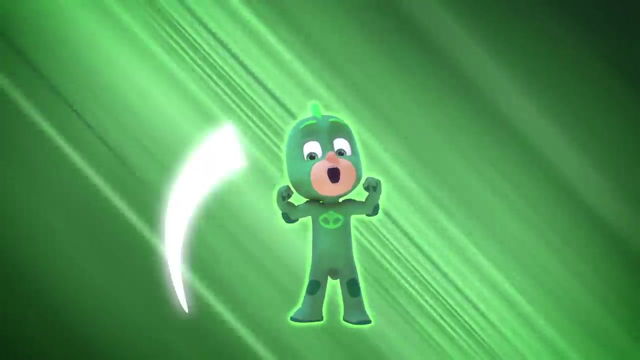 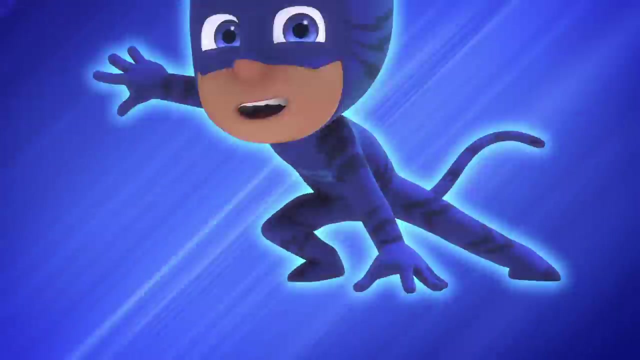 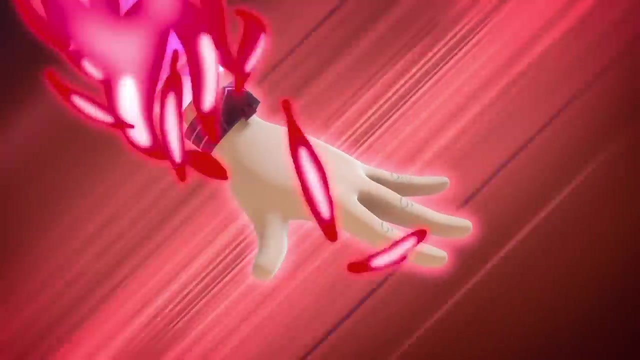 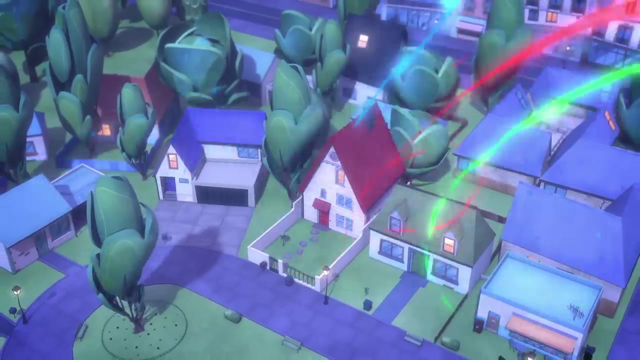 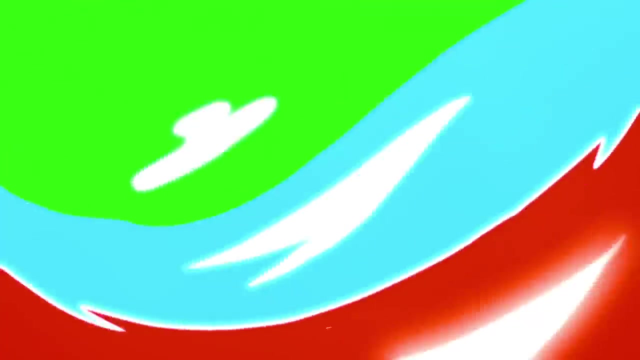 is ready to face fiendish villains to stop them messing with your day. Yeah, Greg becomes Gekka. Yeah, Connor becomes Catboy, Amaya becomes Owlette. The PJ Masks, Come on, come on, come on. 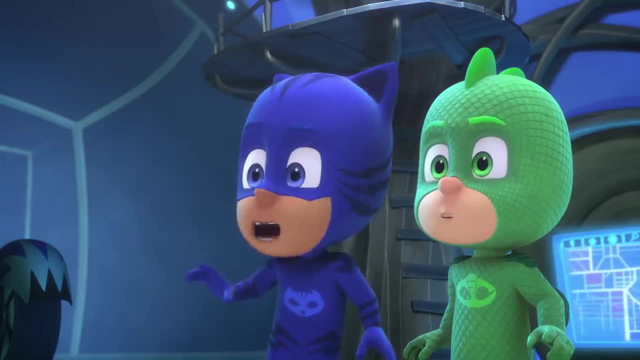 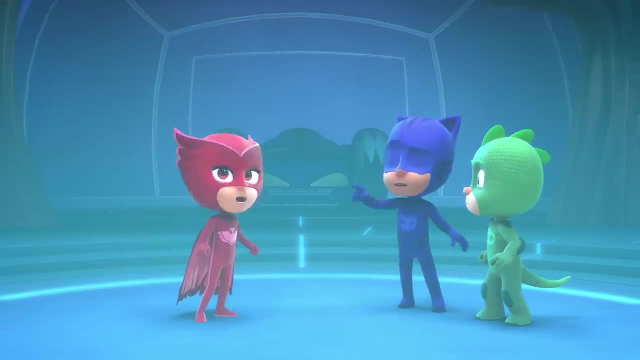 To the Owl Glider. Wait, Owlette, If we're going to follow that trail, we need to be on the ground. All right, good point. I just really want you guys to ride it. Okay, so Do the. 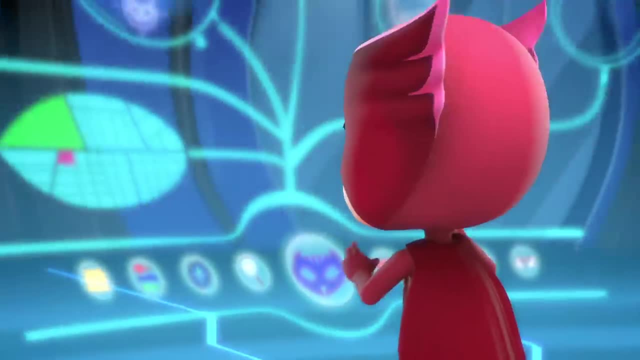 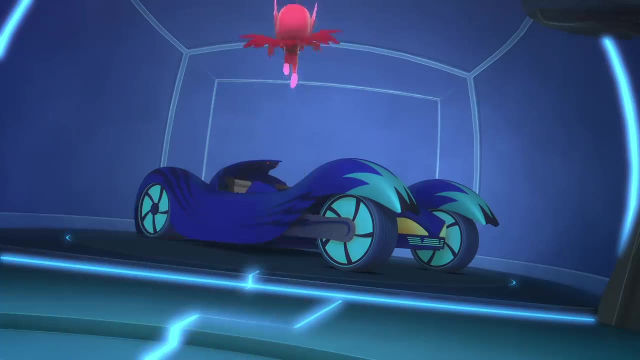 Gekka, I know let's do it. Oh, look at that. Oh, that's up there. Let's really speed it up. Let's go. Okay, let's do it If we think we're going in and out of that tunnel. 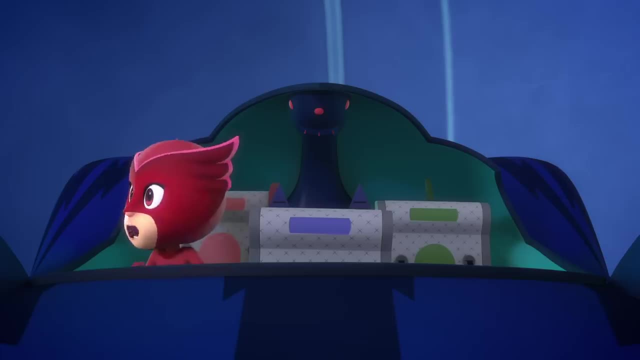 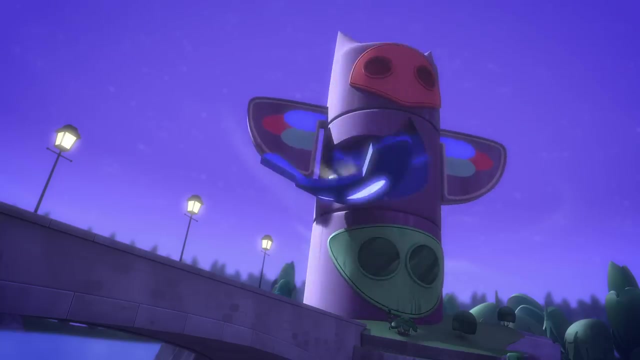 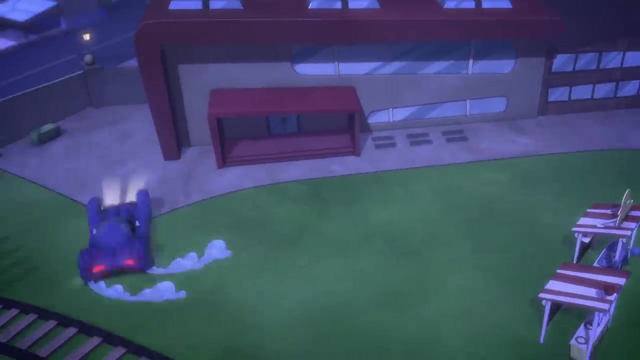 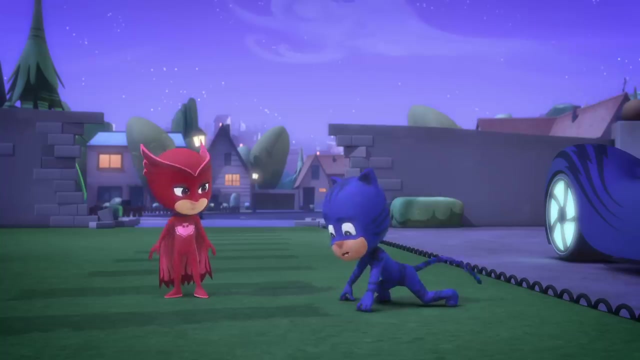 is that what you would plan on getting dela? Oh yeah, right, Right, She's really impatient. Come on, guys, let's go Ready, set, go Looking, looking nothing here. Wait, Owlette, the marks from the missing train tracks are here, remember? 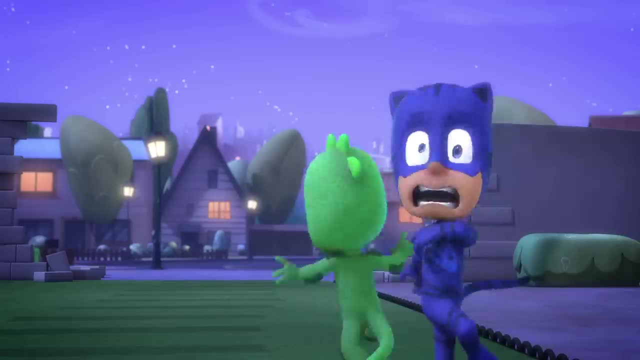 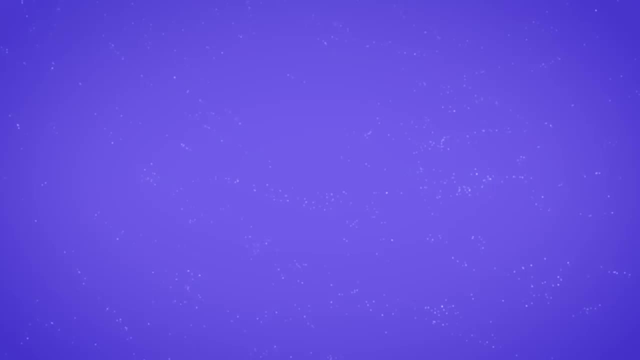 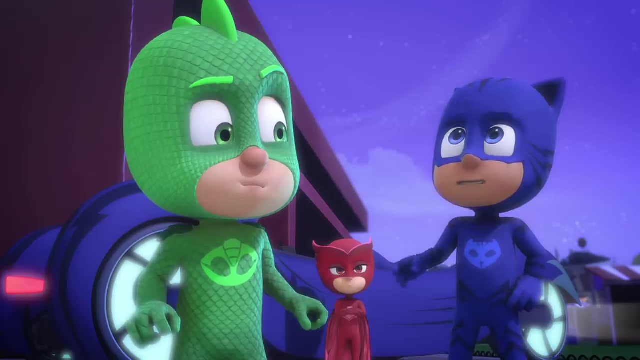 So if we follow them, we'll find the train. Yes, let's go, let's go. Ah, Was that Romeo's lab? It looked like it Gekko, but it was all over the place. Maybe there's a. 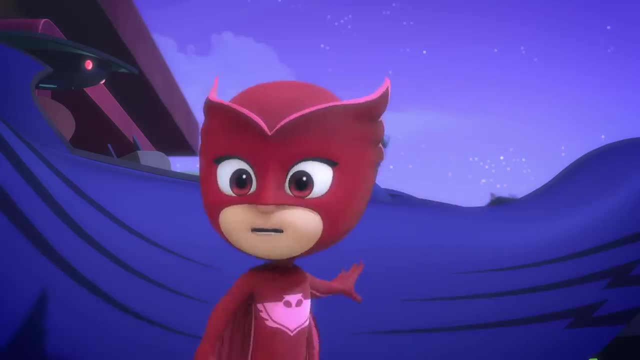 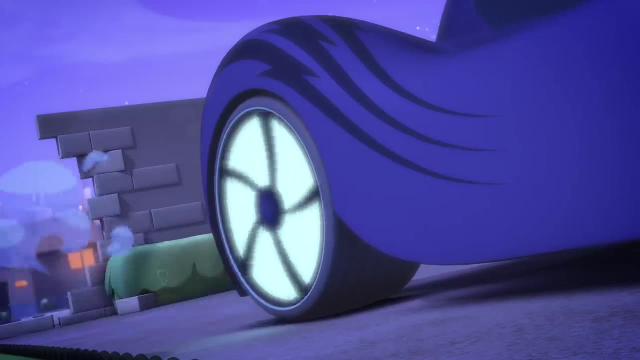 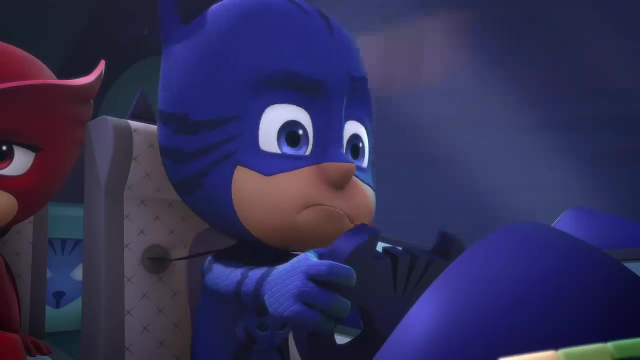 Guys, never mind Romeo. If he's in his lab, he can't be driving that train and we need to find out who is Go. go, go, Uh, OK, OK, Hmm, no more tracks. How will we find the train now? 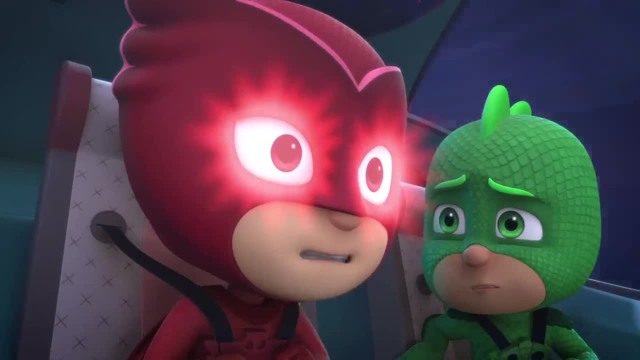 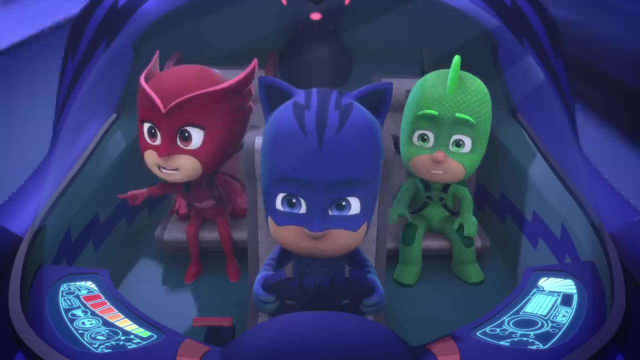 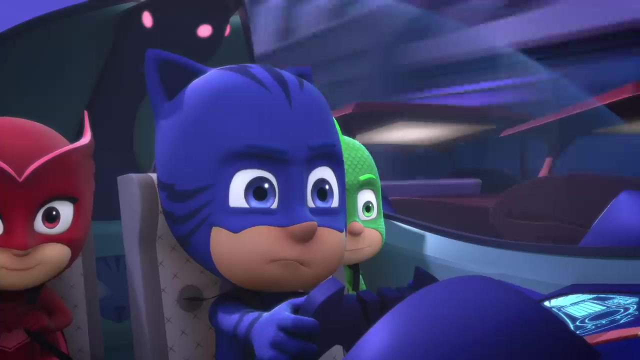 Owl-eyes. I see something up ahead, something fast. That's it the train. See, I told you it was fast. Now let's see who's driving Romeo. Well, hello, PJ Masks. But we've got to find the train. 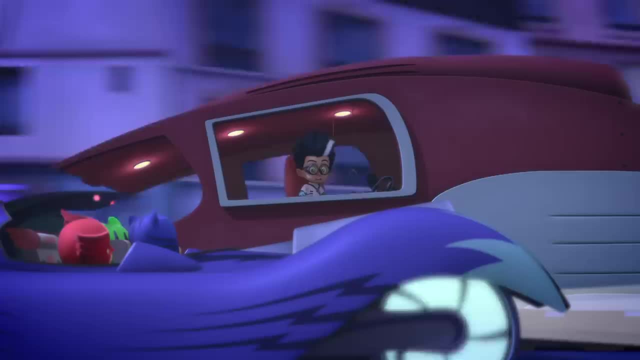 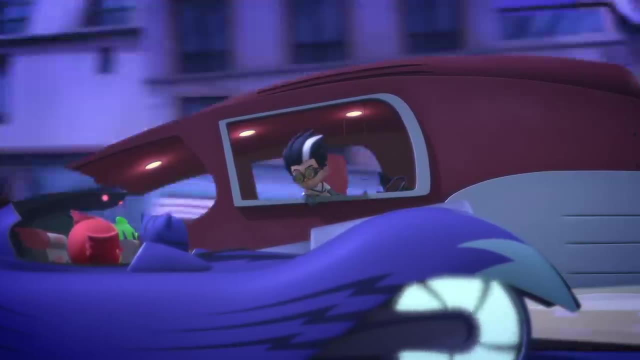 No, no, no, no, no, no. But we just saw you driving your lab. That wasn't me. No one's driving my lab. Silly thing: short-circuited and took off by itself. Good thing I've got this super-fast train to catch it with, eh. 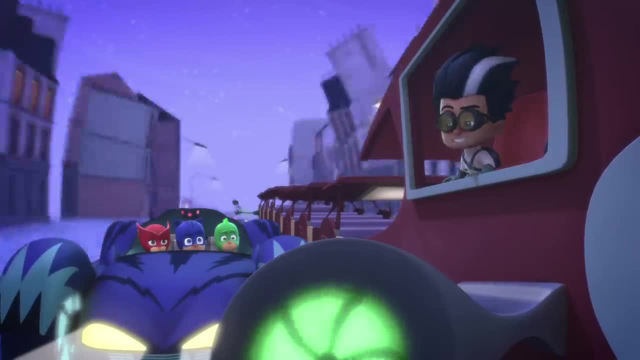 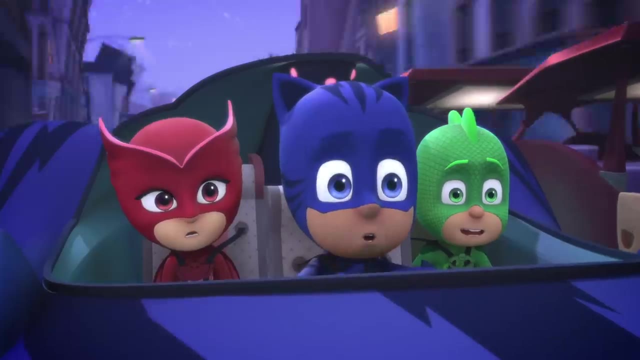 Well, where did these train tracks come from? Easy ha, Thanks to my invention, the Tracker Whacker, It makes tracks anywhere. Wow, that is pretty cool. And what's even cooler is the other one at the back that picks the tracks up again. 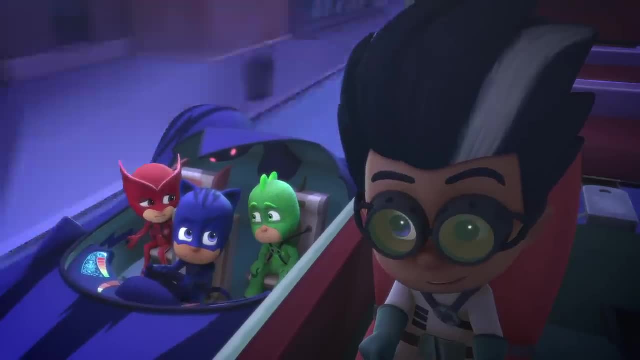 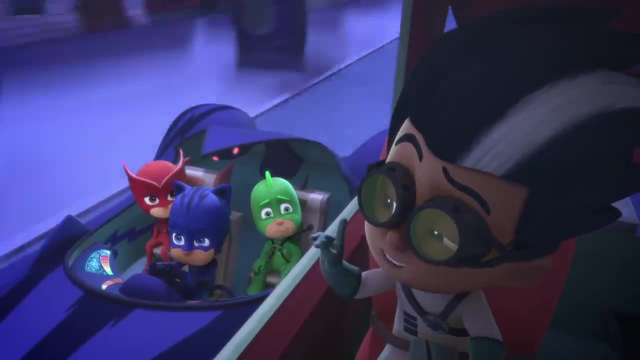 But, Romeo, you don't need this train, We can catch your lab for you. Ha Like, I'm giving this train up once I get my lab. No way, With the tools from my lab, I can make this train even faster. 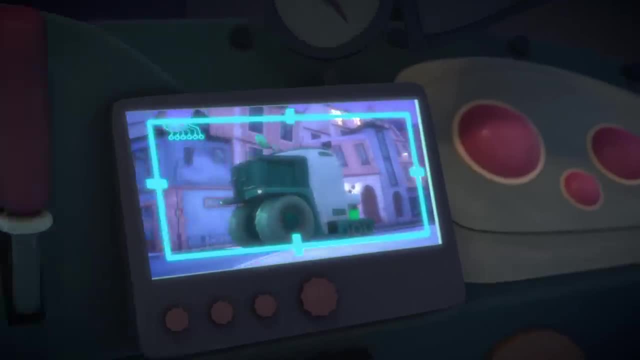 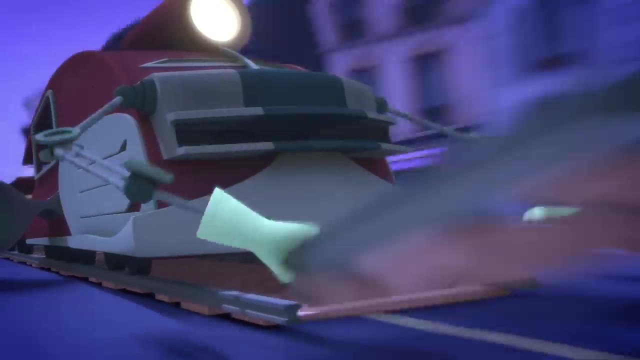 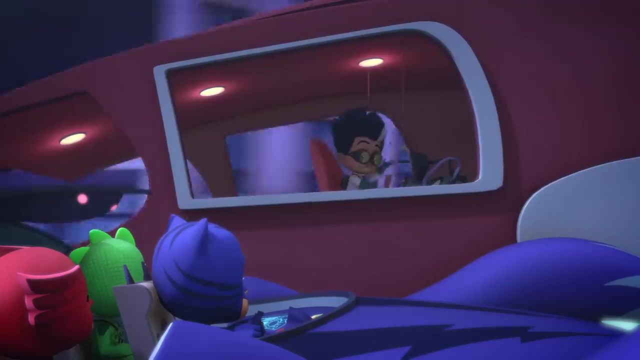 I'll be the fastest villain in the world. Huh, Aha, There you are my lab. Ha. Bye-bye, PJ Masks. Looks like you've missed this train. Woo-ha-ha-ha, We've got to stop him from catching his lab. 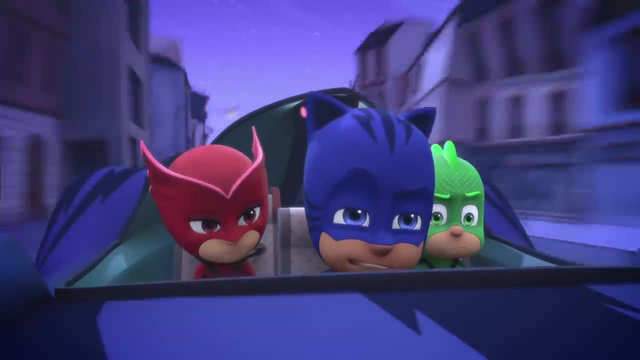 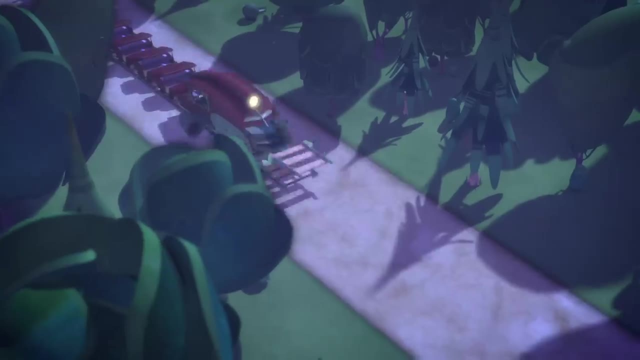 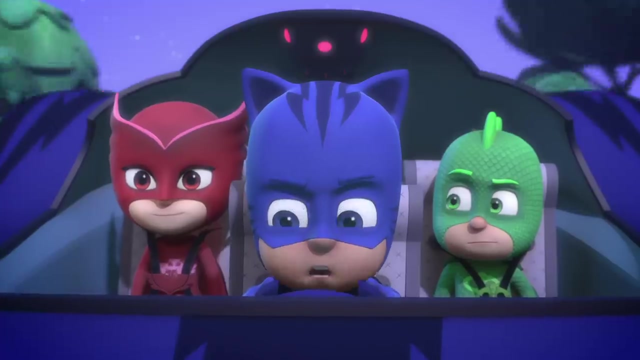 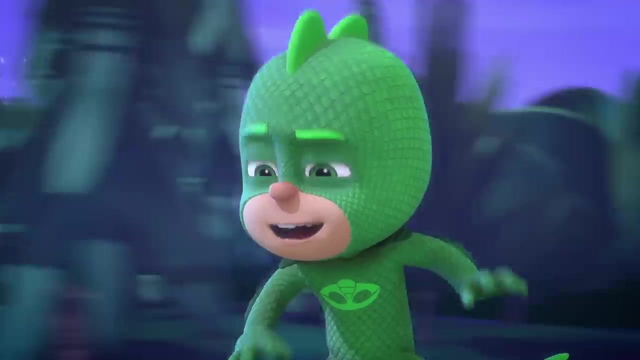 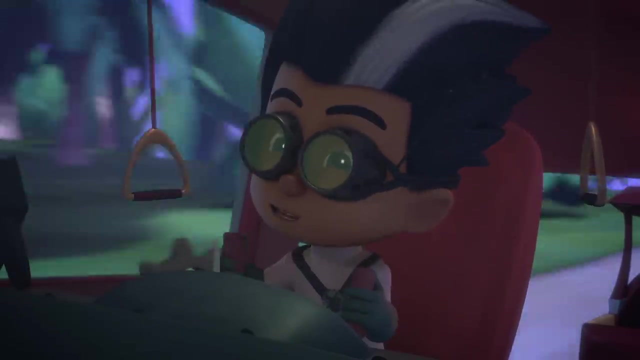 and making that train even more dangerous. On it. Owlette, Here we come, Romeo, Autopilot, Awesome. And wow, This train is pretty cool. Ha, I've almost caught up with you, you naughty lab, Ha. 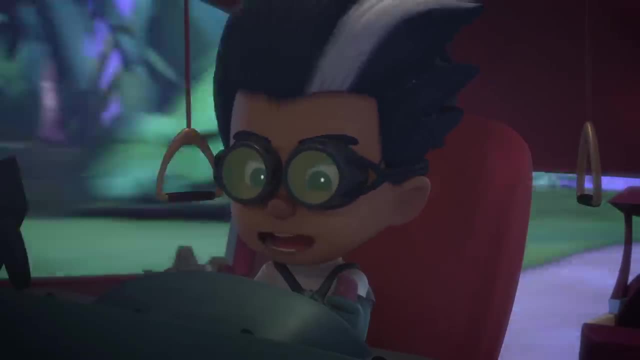 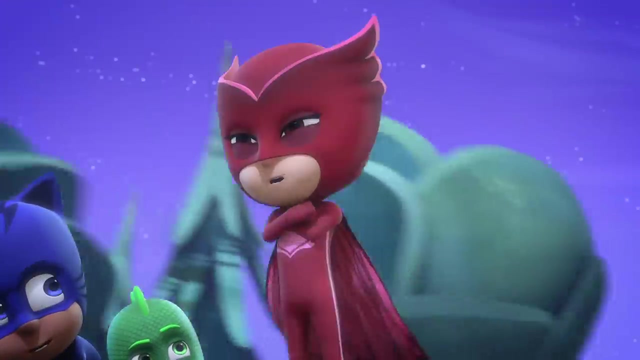 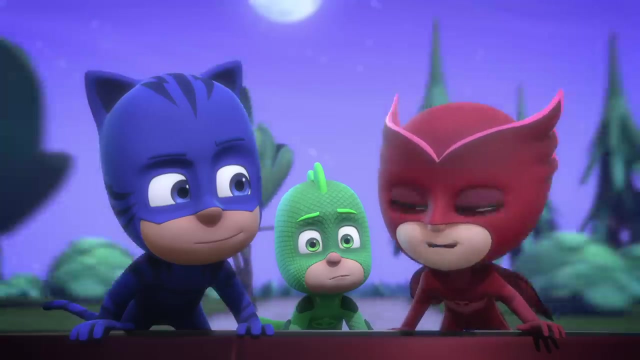 Those PJ Masks were never gonna catch me in that super-slow cat car. Come on, PJ Masks, Let's stop. Romeo. Super Owl Wings Owlette. Whoa, I was almost bird feed. Thanks, Catboy, No rush Owlette. 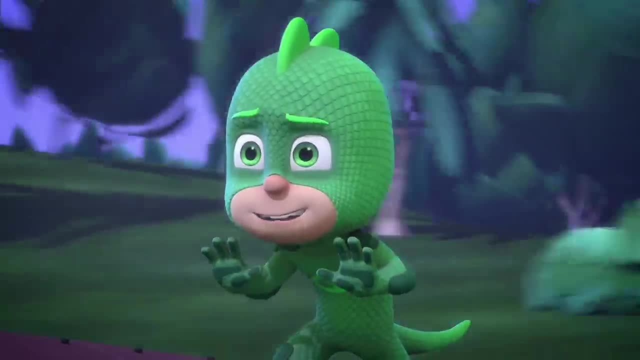 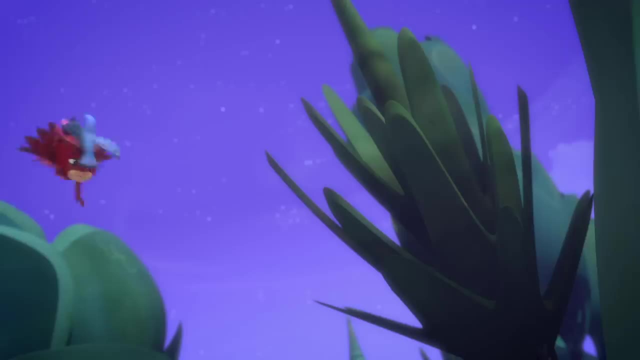 We'll get there. Hey, Let's sneak up on him really, really slowly. Why be slow? Let's just go. Whoa Ha-ha, Whoa, Owlette, Owlette, Owlette, Owlette, I'm okay. 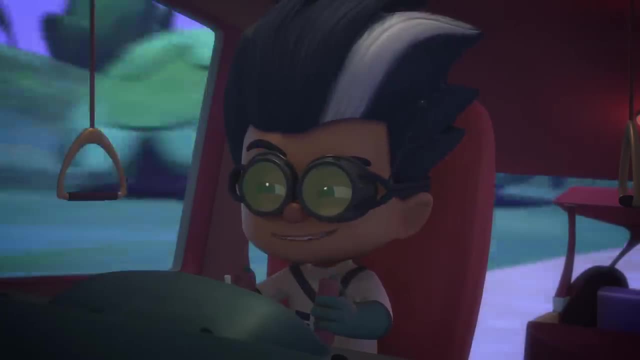 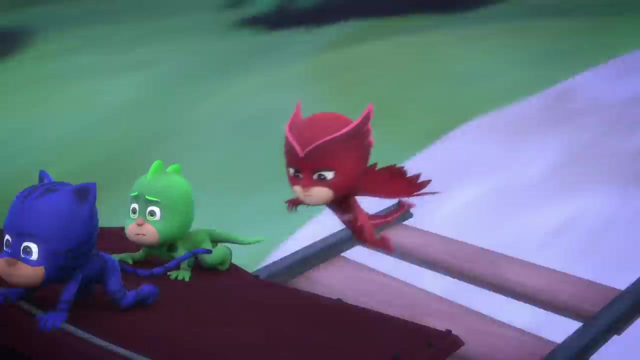 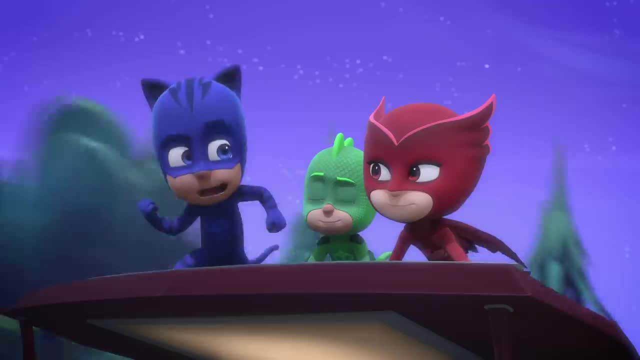 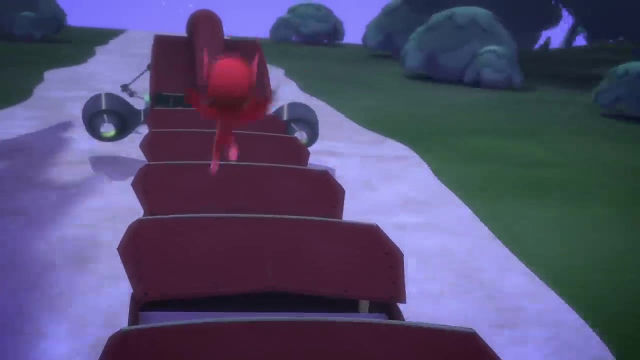 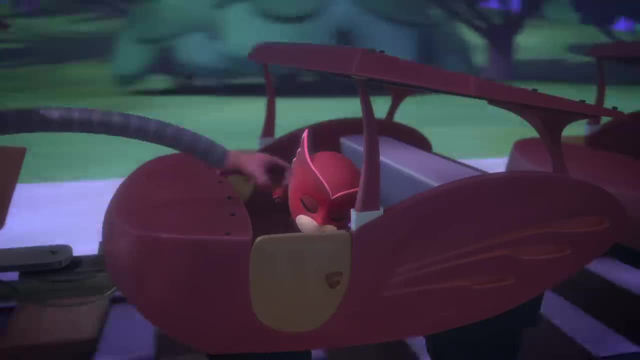 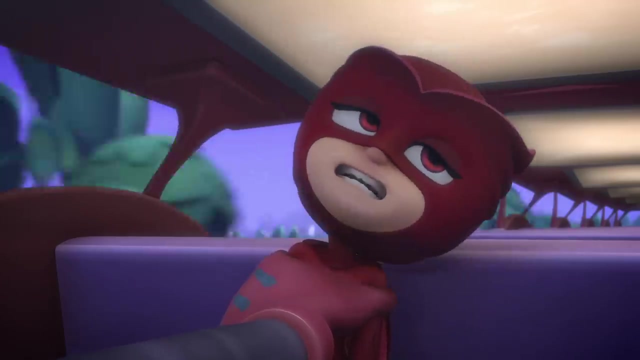 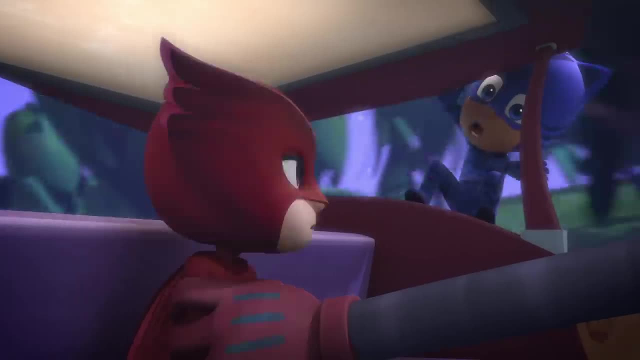 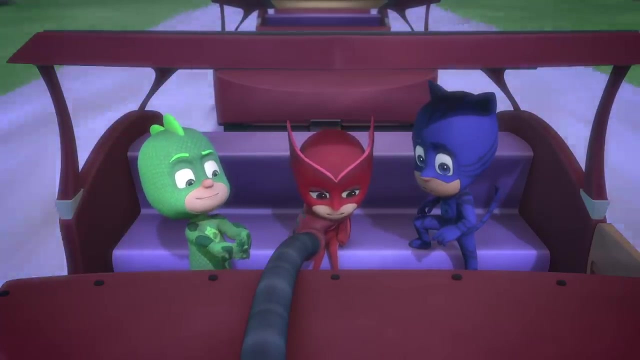 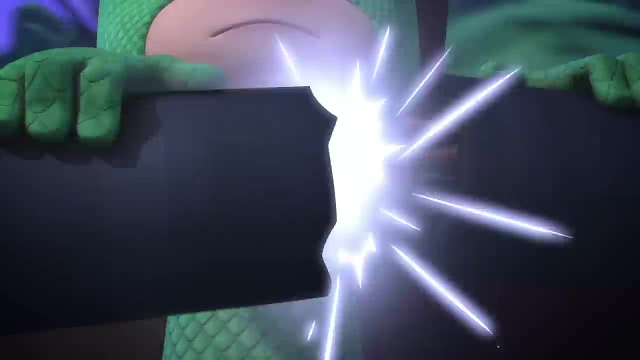 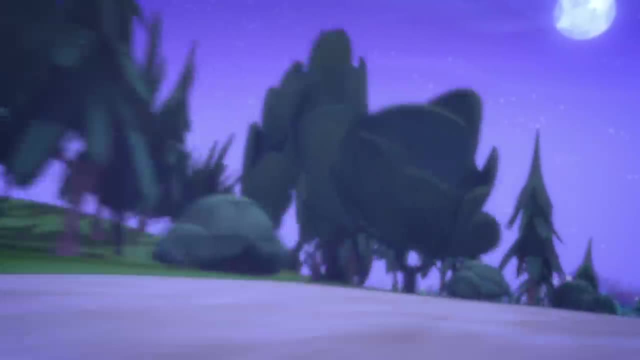 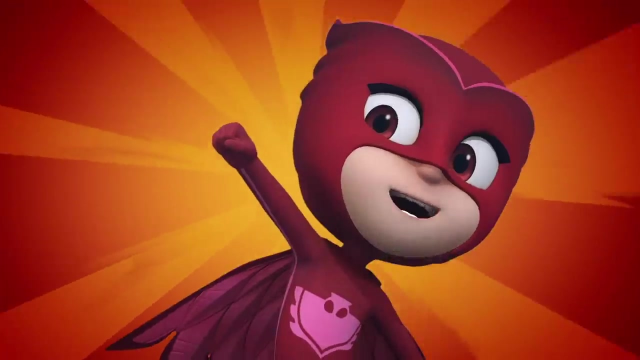 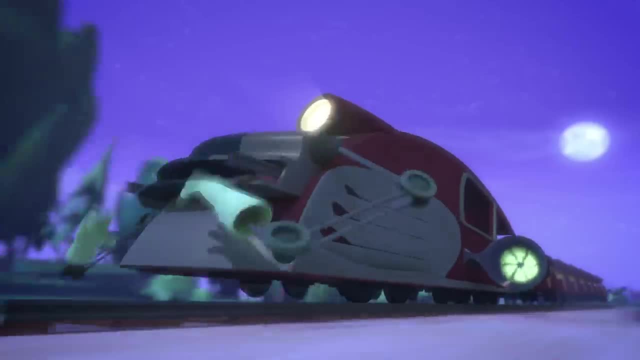 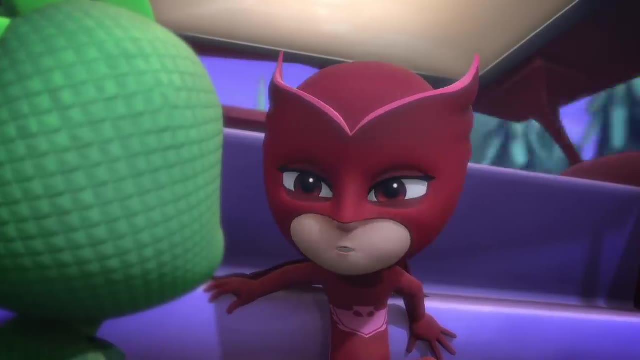 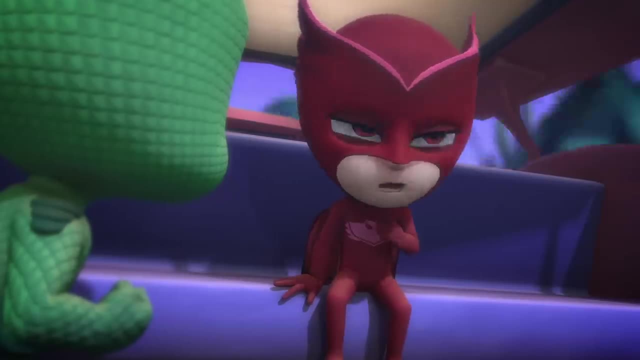 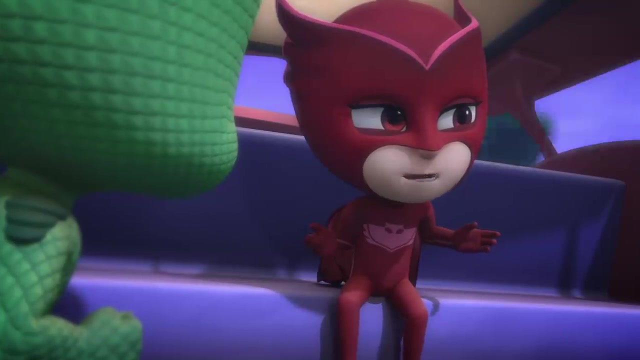 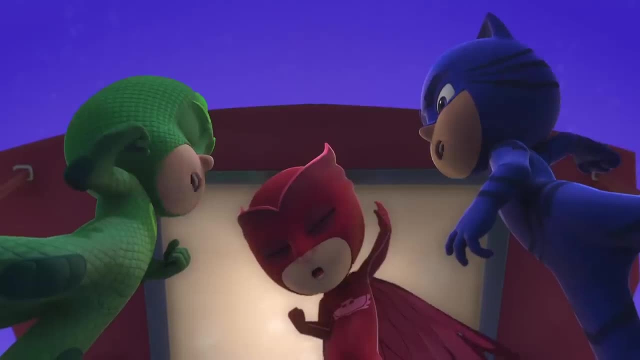 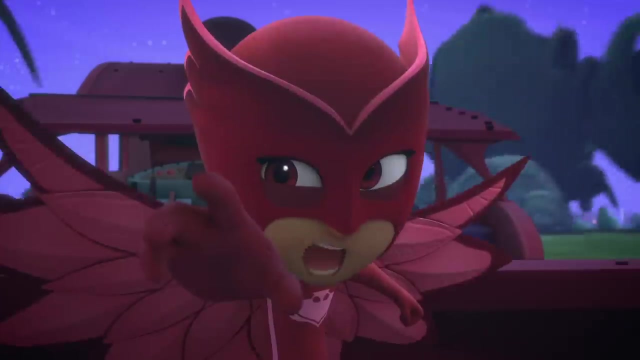 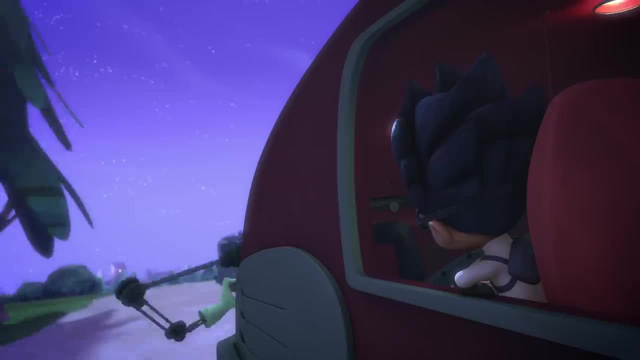 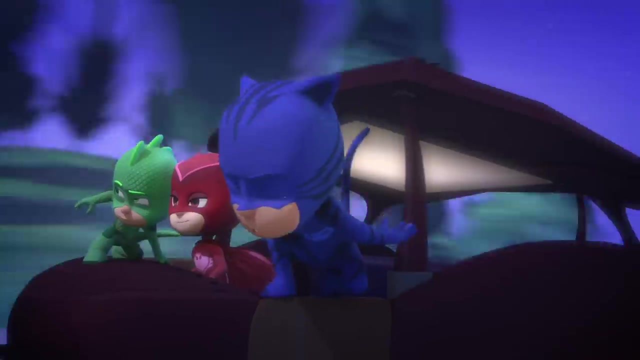 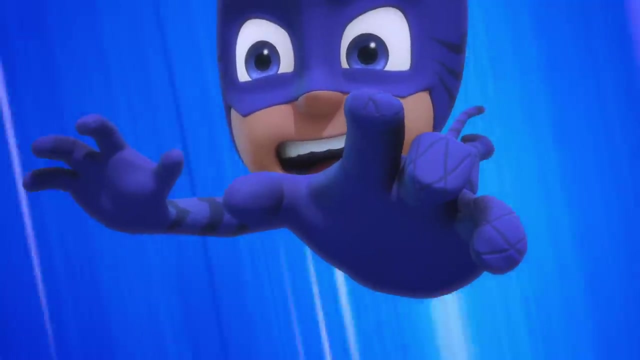 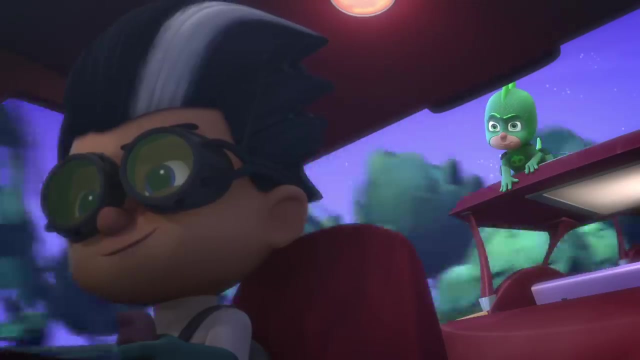 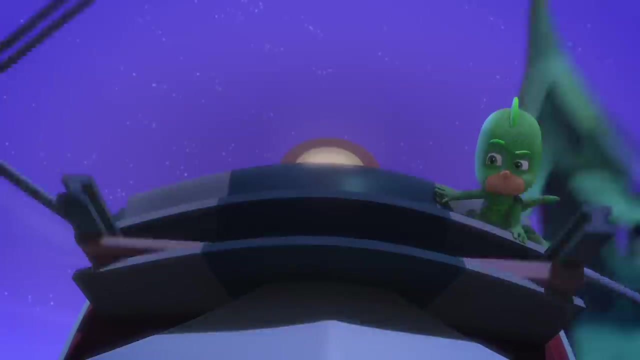 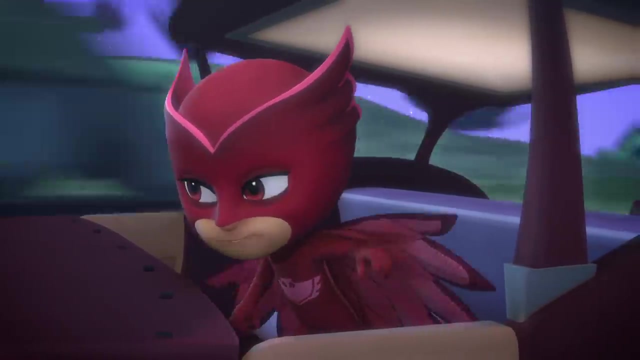 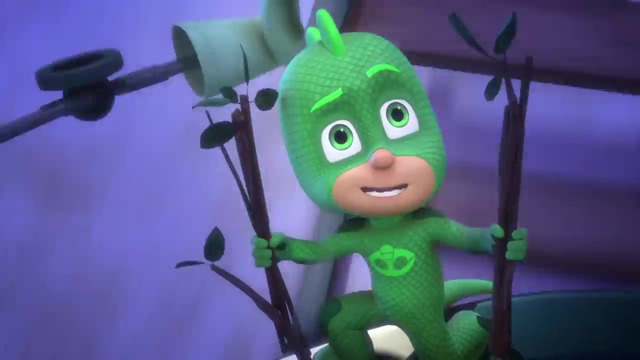 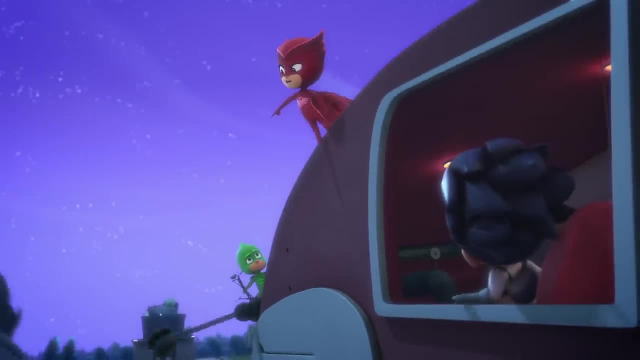 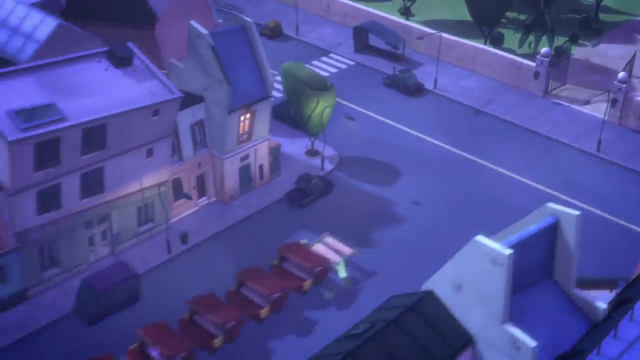 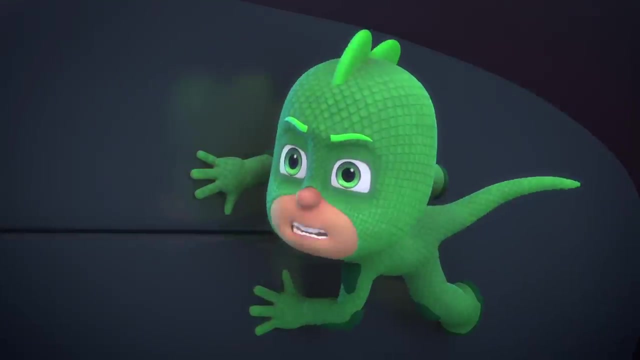 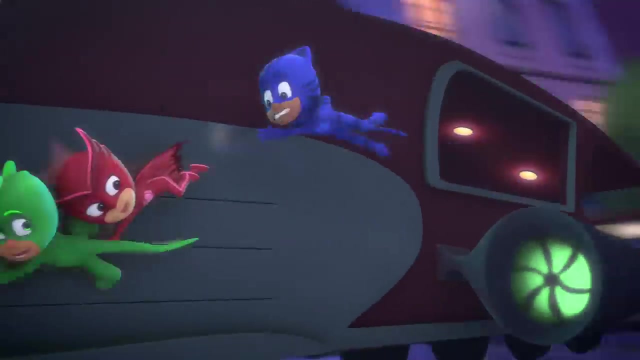 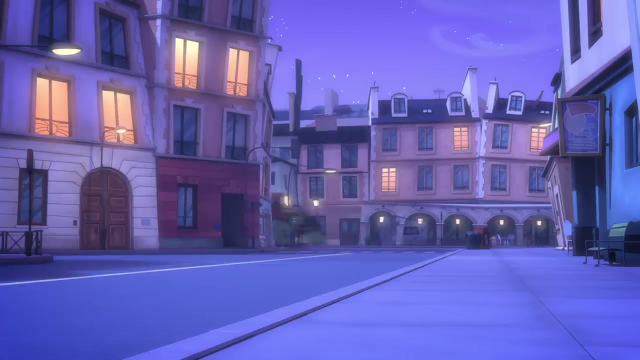 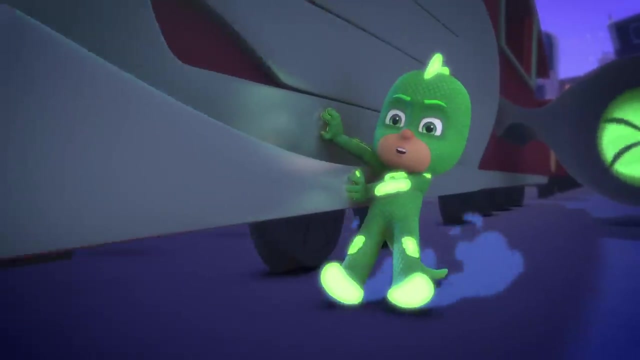 Too late, Romeo, Get go, Jam that tracker-whacker. No, Whoa, Super Lizard Grip. Hang on to me everyone. I've got this. Super Lizard Grip, Super Lizard Grip, Gekko Muscle. 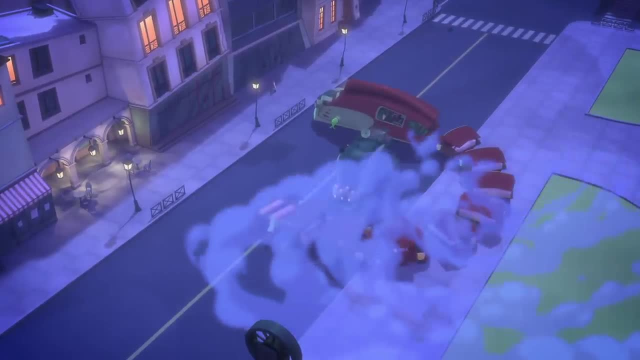 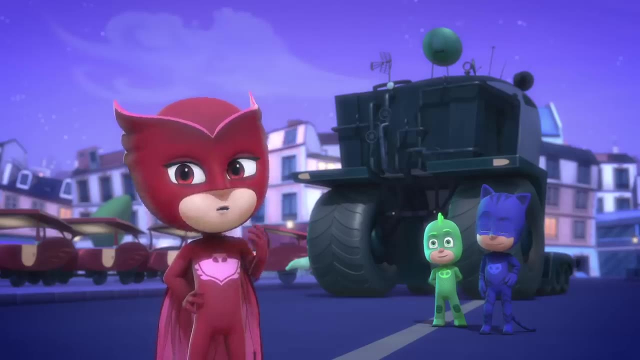 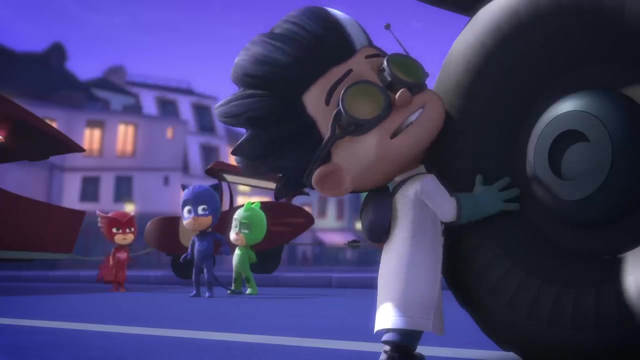 Ah, Aw, Huh. See, Romeo, I told you we could catch your lab, My lovely lab. Yes, yes, yes, I might have lost my train, but I'll always have you, my lovely lab. Now, let's get this train back home. 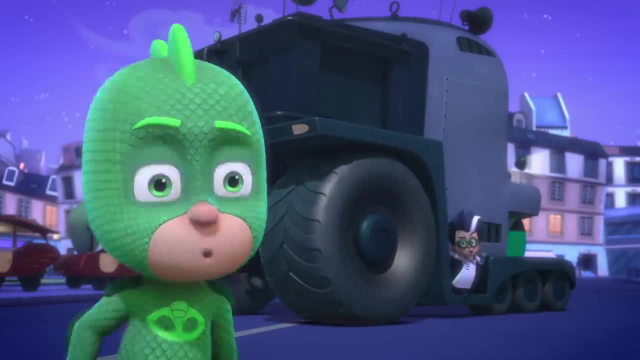 Everyone at the fair will be so happy. I'll see you next time, PJ Masks. Huh, He didn't even say thanks for helping. Don't worry, Gekko, We saved the Fairground Flyer train. PJ Masks, I'll shout hooray. 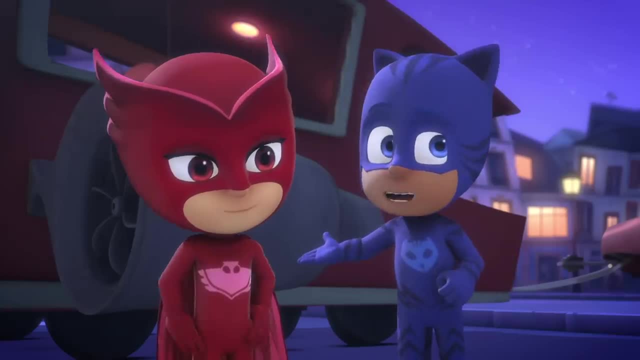 Because in the night we save the day. Yay, Come on, It's almost time. I've been on this train once, but I can't wait to ride it again. Woo-hoo, Yeah, Hey, you guys go ahead. 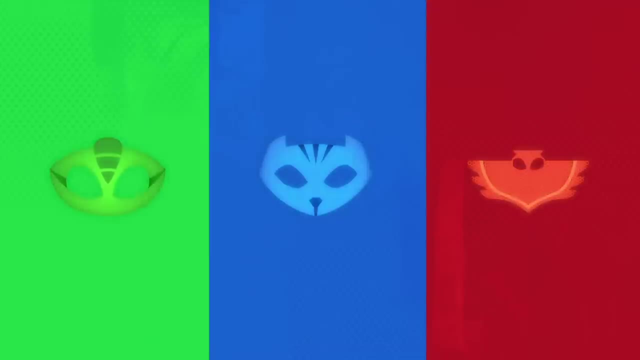 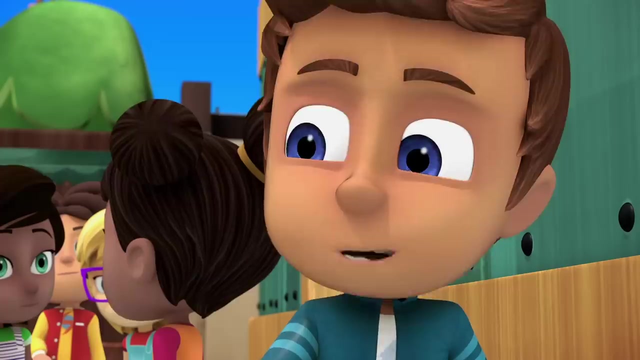 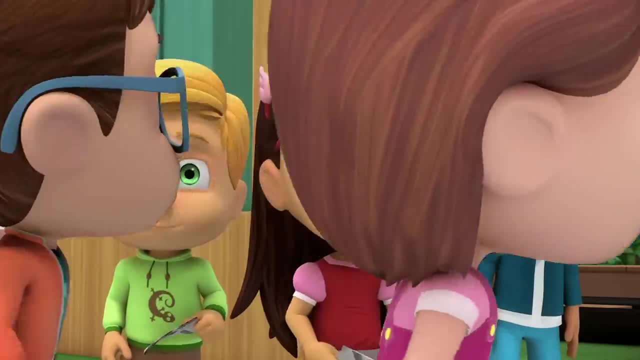 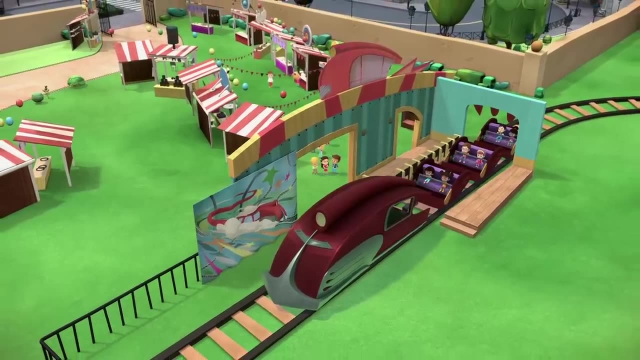 Yay, Yay, Yay, Yay, Yay, Yay Yay. Thanks Amaya, I'm happy to wait. Enjoy the ride. It goes pretty fast, Gekko's Nice Ice Plan Huh. 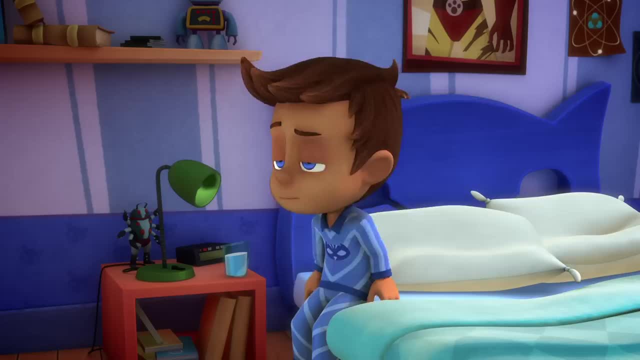 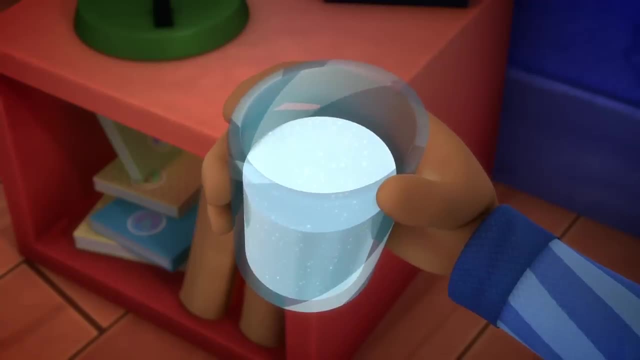 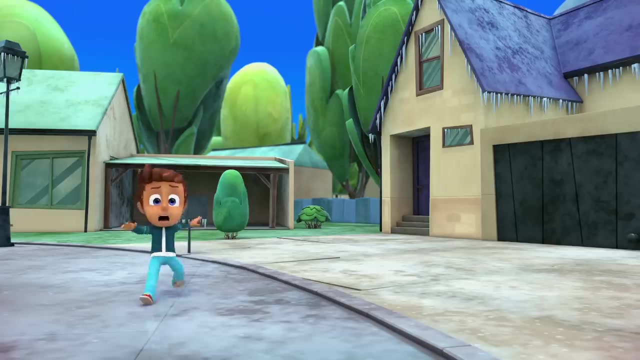 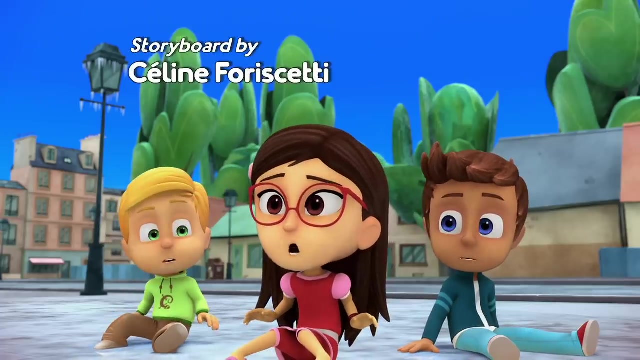 What's this Ice? But it's the middle of summer, Icicles, Whoa, Whoa-heh. Ah, Yo, Wooo, Wow, Woo-hoo, Whoa, Whoa. That was awesome. There's ice all over the place. 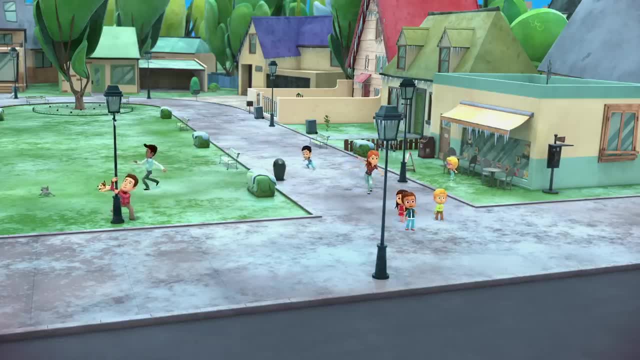 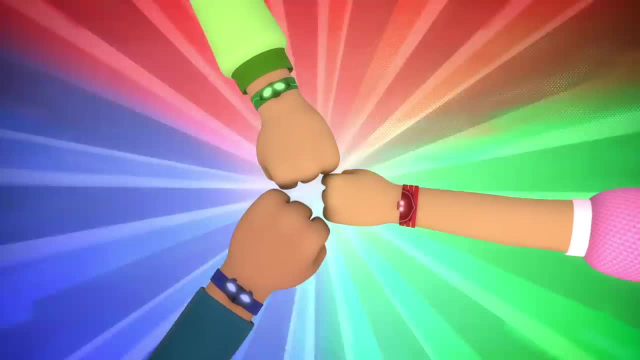 Everyone's slipping and sliding, But only to the end of the street. Then it just stops. What's going on? We'll find out tonight. PJ Masks, we're on our way Into the night to save the day: Night in the city. 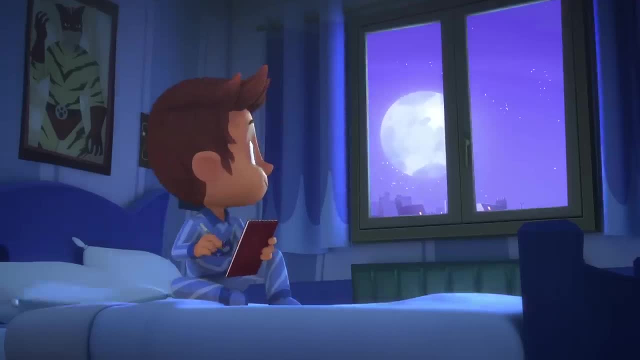 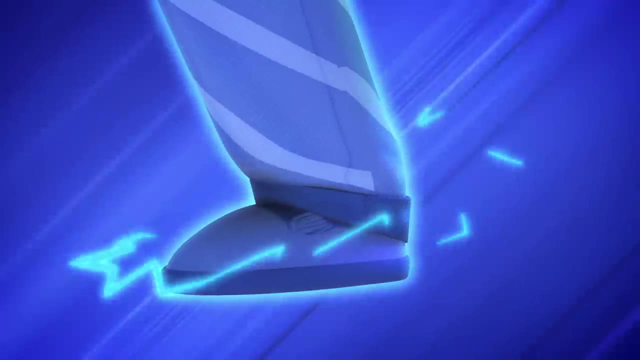 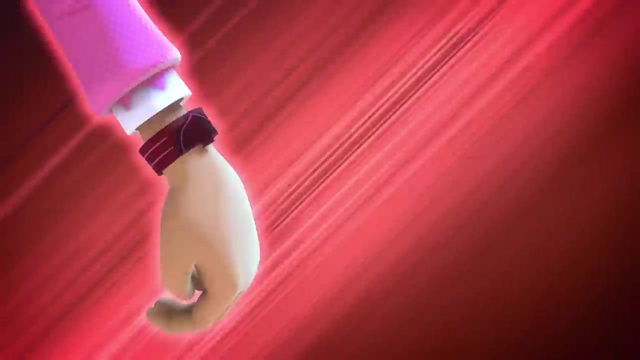 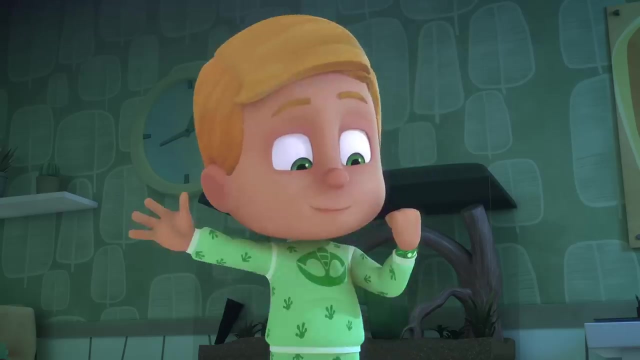 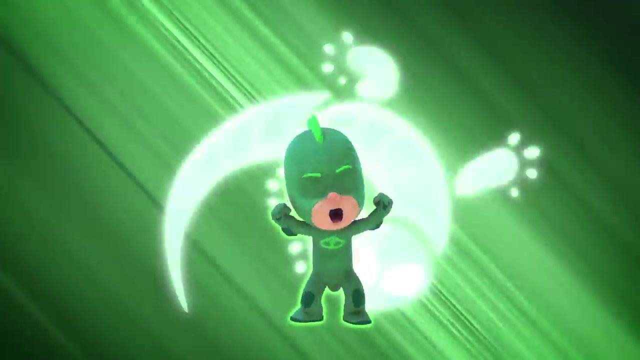 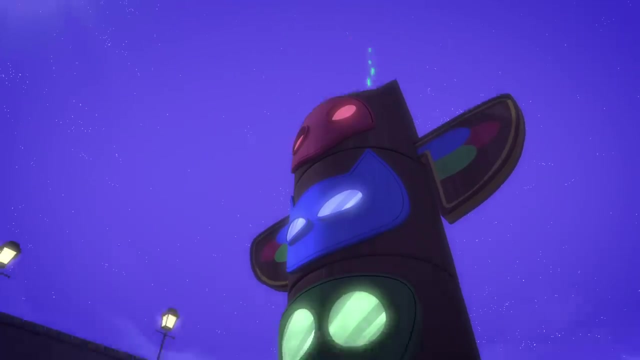 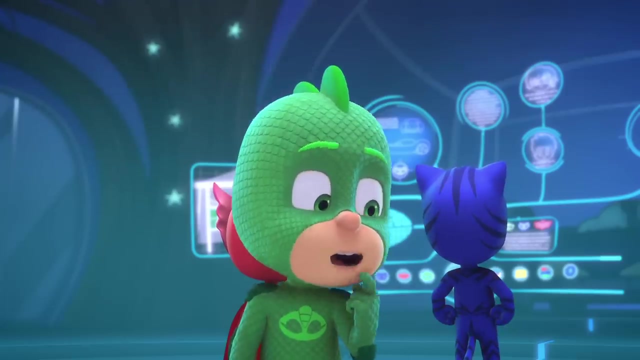 And a brave band of heroes is ready to face fiendish villains to stop them messing with your day. Connor becomes Catboy, Amaya becomes Owlette- Yeah, Greg becomes Gekko. The PJ Masks, The Gekkomobile can stick to anything. 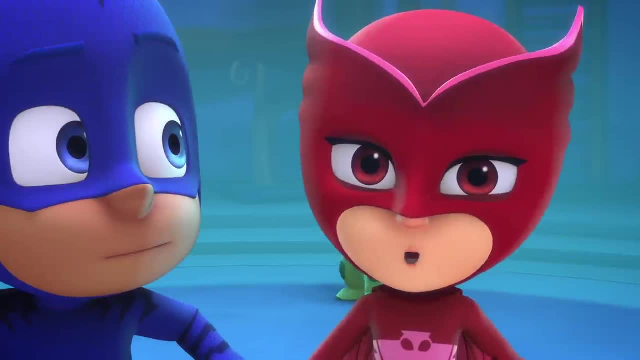 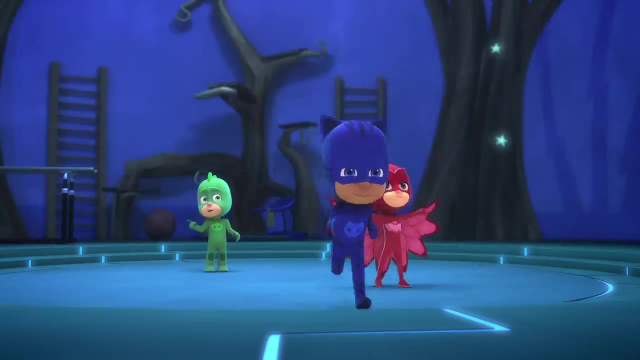 It'd be perfect for the ice. What about the Gek? Let's take the Owl Glider. We can check everything out from above. Good thinking, Owlette, But I thought the Gekkomobile could. No, They're probably. 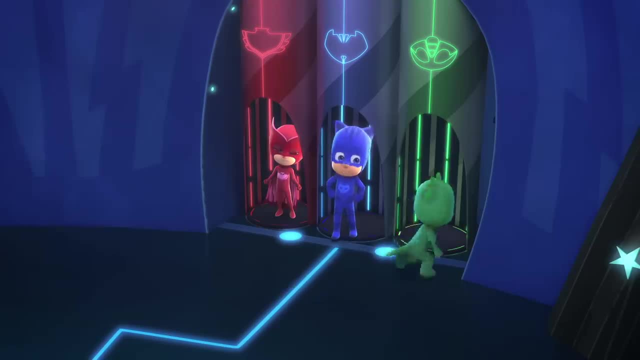 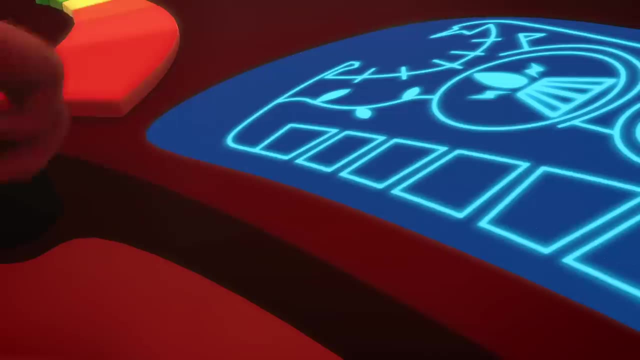 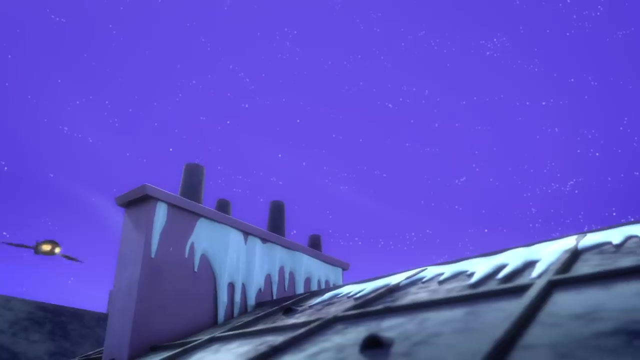 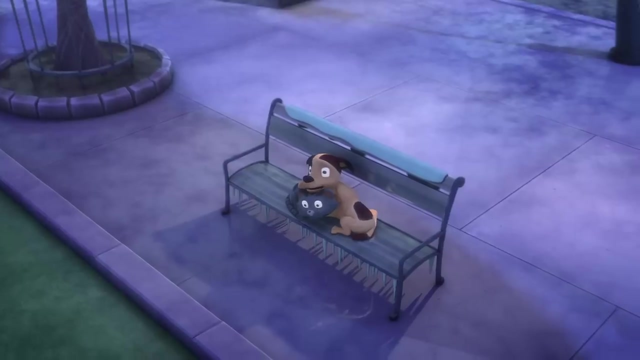 They're probably right. Shh, Come on, Gekko, Let's go save the day. It's even worse now. Almost half the city's frozen. Even the cats and dogs have made friends to stay warm. Whoa Wow. 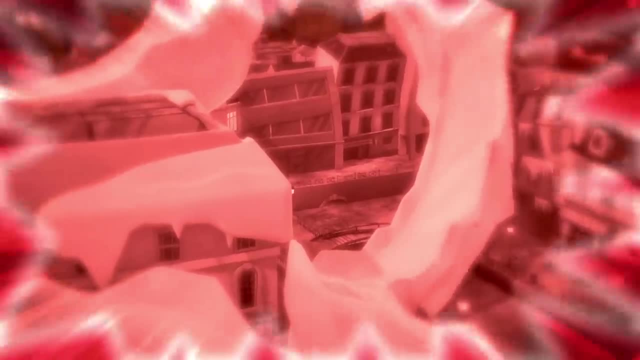 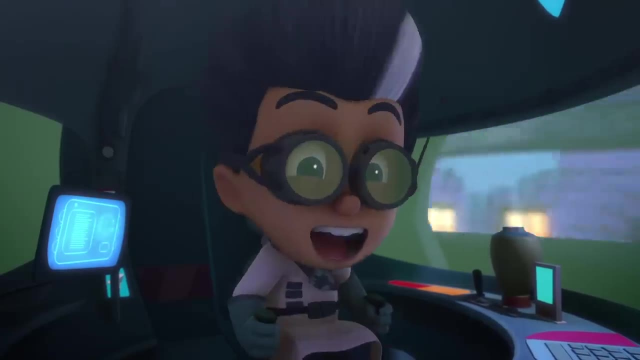 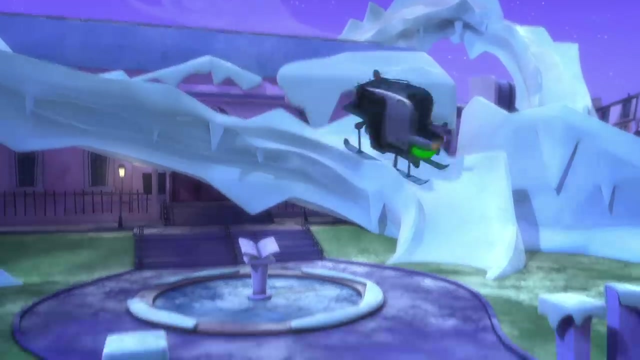 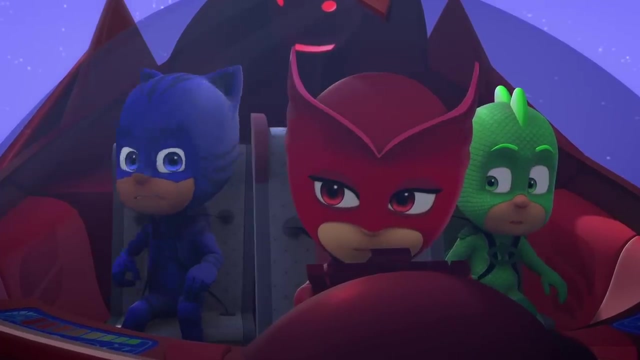 What's that? Owl eyes? Hmm, Look over there, Romeo's lab. Whee, This is so much fun. I knew Romeo was behind this. What's that on the front That looks like an ice machine. Go after him, Owlette. 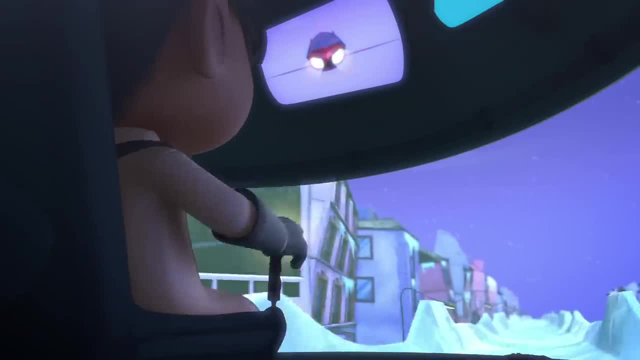 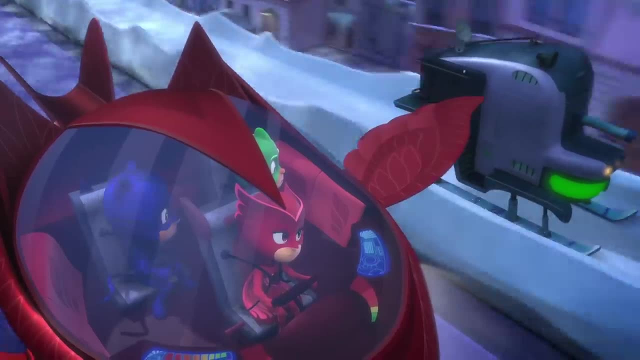 Aha, I wondered how long it would be before you PJ do-gooders showed up. Where are you up to, Romeo, Isn't it obvious? I'm making the city into an icy rollercoaster for my new lab, toboggan. 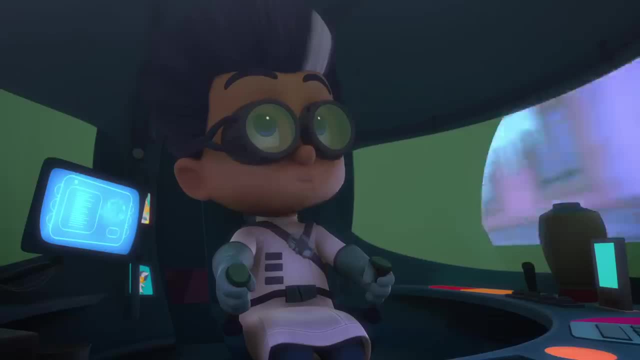 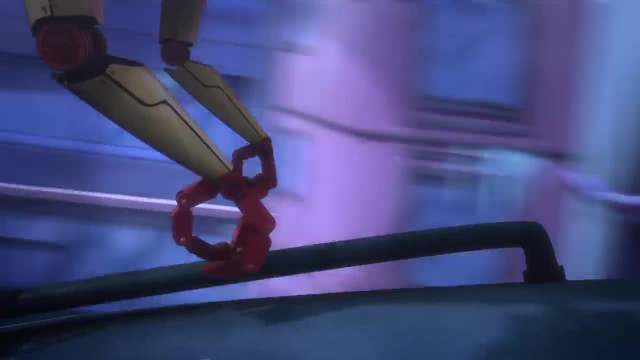 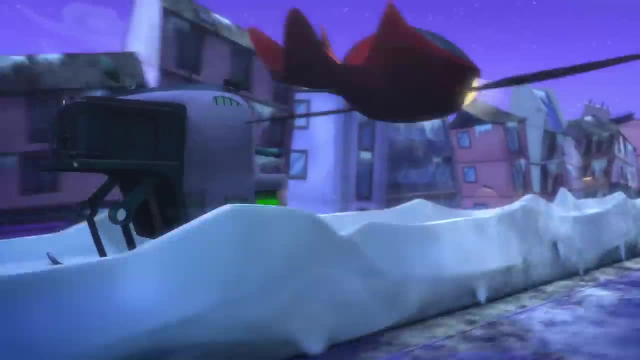 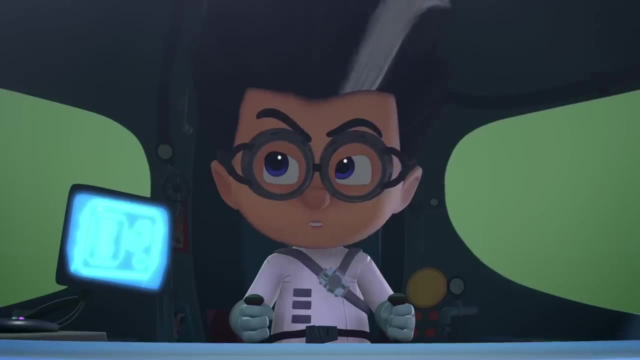 I made it. I made it Woo-hoo. If you just want an amazing ride, Romeo, I could use my super gecko muscles to push your lab around on its wheels. It's not just about having fun, even though it is fun. 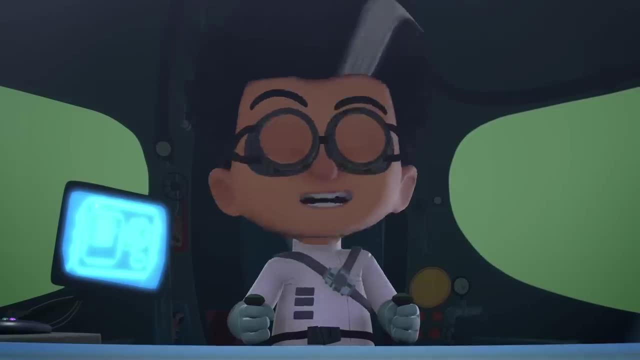 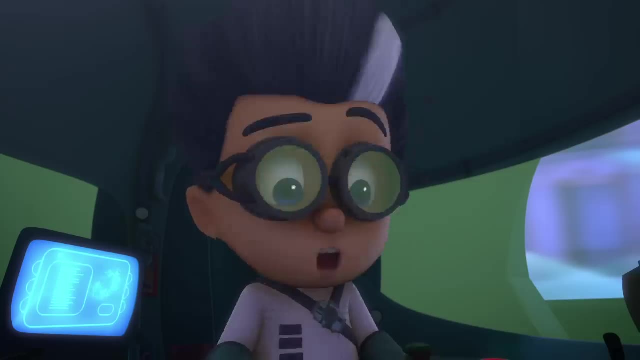 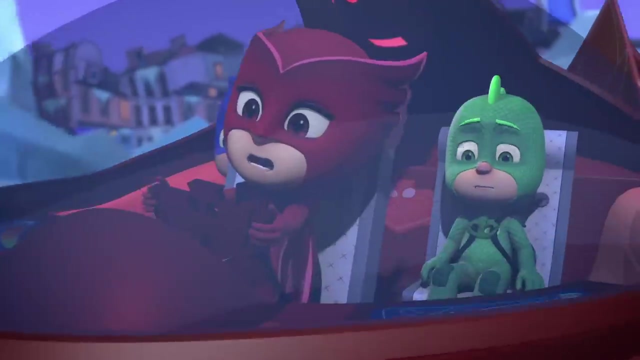 While you daytime dodos are all slip sliding around, I'll be taking over the whole world. Romeo's taking over the whole world. Ugh, that's steep. Whoa, Whoa, Whoa, Whoa Luttering feathers. 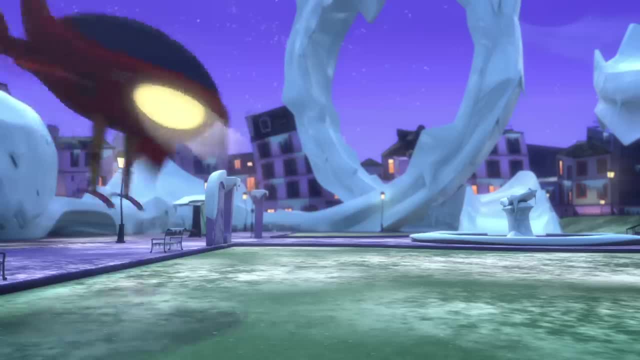 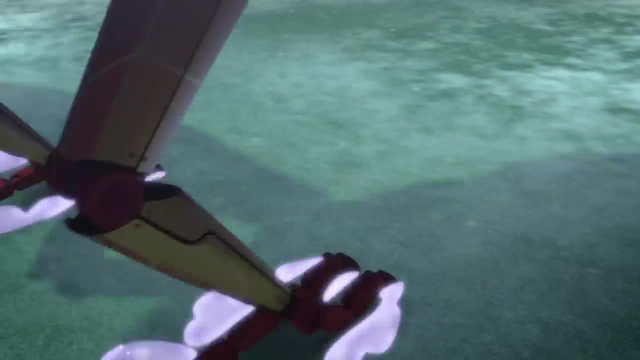 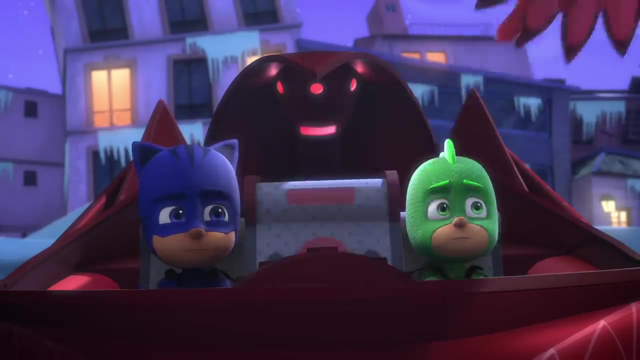 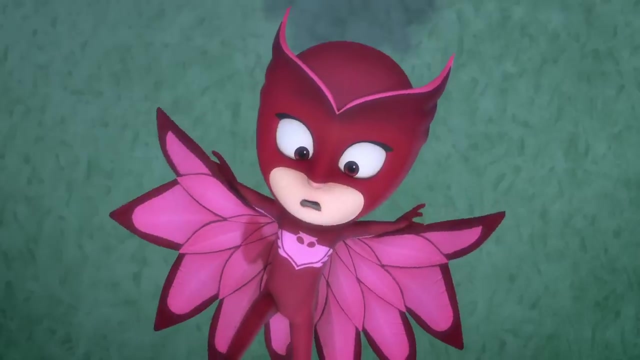 I can't fit through. We'll have to land Whoa, Whoa, whoa, whoa, Whoa. We've got to stop him before he ices anything else up. Whoa, It's really slippery. Whoa. 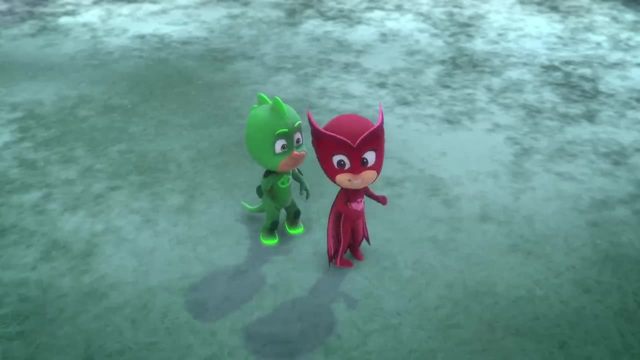 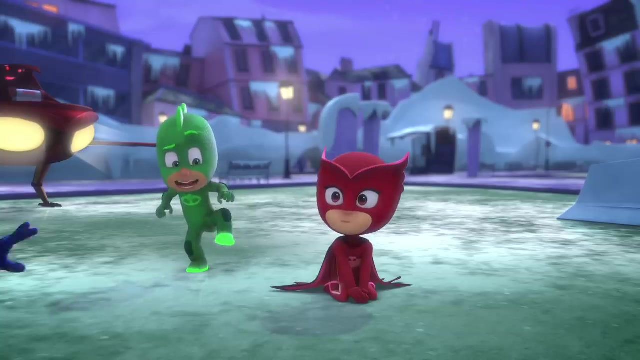 Whoa, Phew. Thanks, Gekko. Whoa. Hey, maybe I could chase Romeo. My feet are really sticky. Hang on, Gekko. Whoa, I've got a plan that'll definitely work, But with my sticky plan we could. 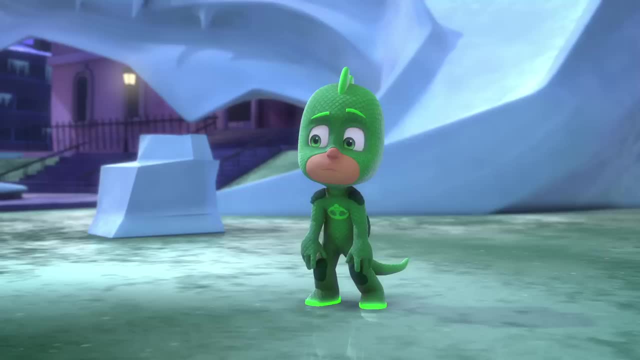 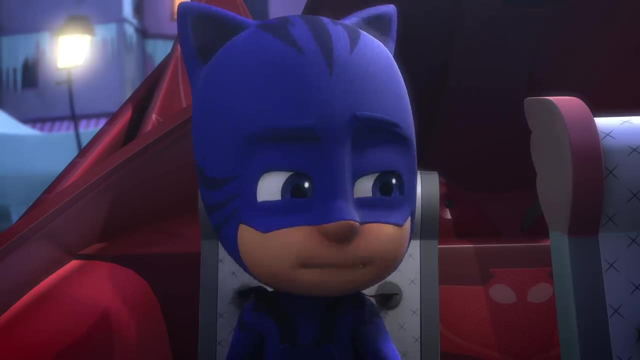 But I'll need some help. Back to the Owl Glider. Oh Well, I suppose it could wait. Owlette, we need your Owl Eyes to find Romeo, Then your flying skills to make sure he doesn't see me, and get to the top. 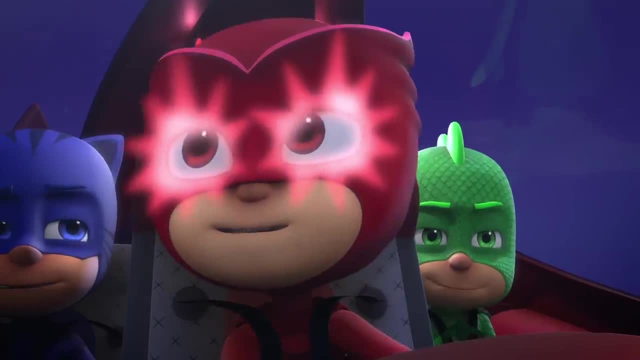 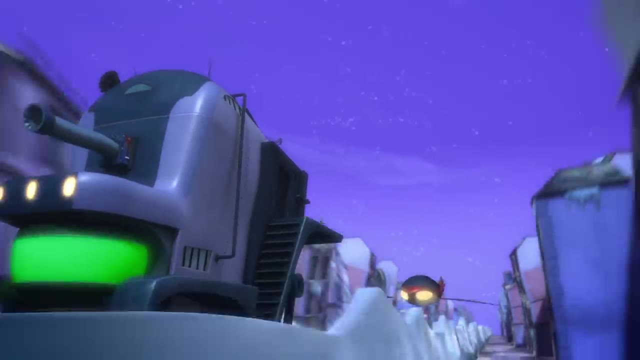 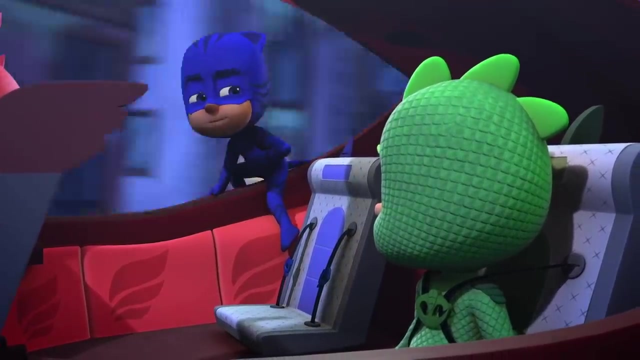 Let's go, Gekko Owl Eyes. There he is, Wahoo. Okay, Gekko, I'm going to sneak onto the lab from below, You sneak on from above, and then we'll take control of the lab. before Romeo ever knows we're there. 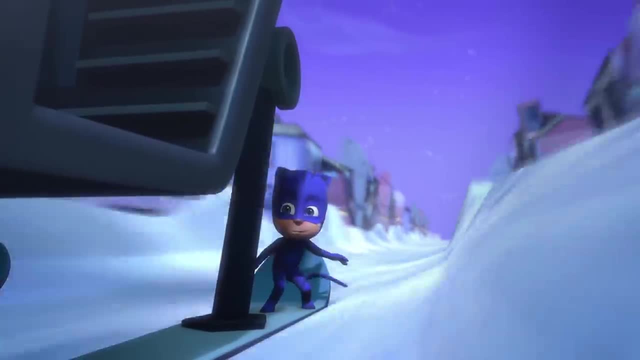 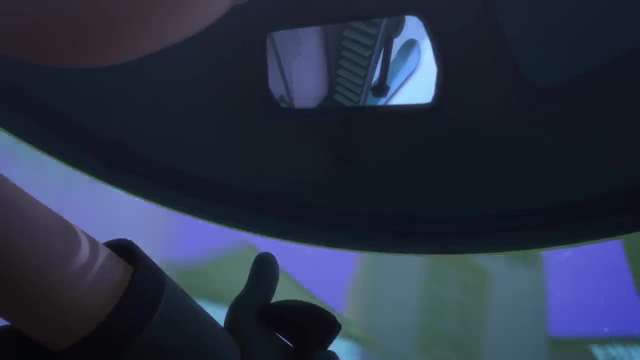 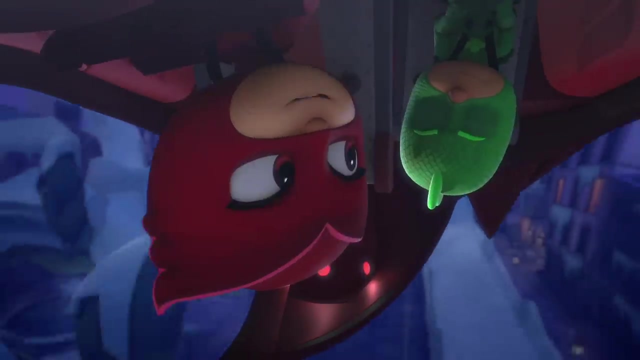 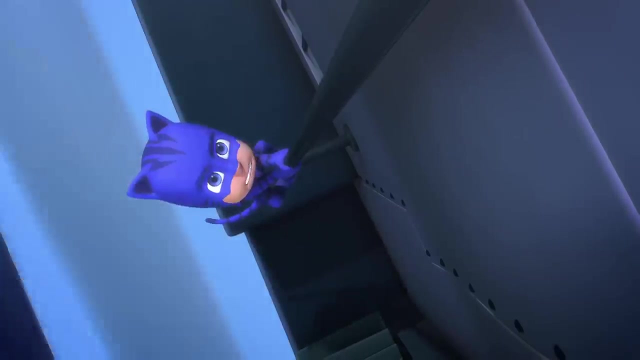 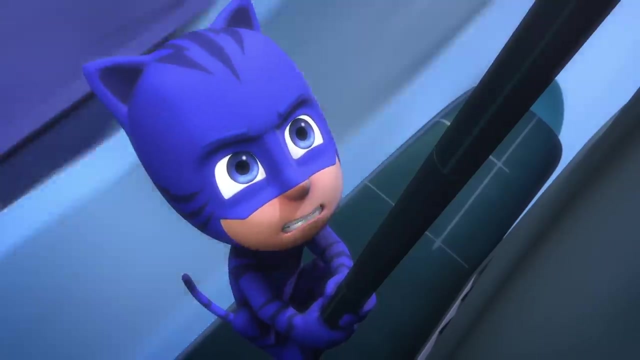 Super Cat Jumps Whoa. Hmm, Must have been the wind- Huh. Catboy leaps like a panther onto the icy pipe and climbs up with his super Whoa, With his super Wah. Nothing beats Catboy. 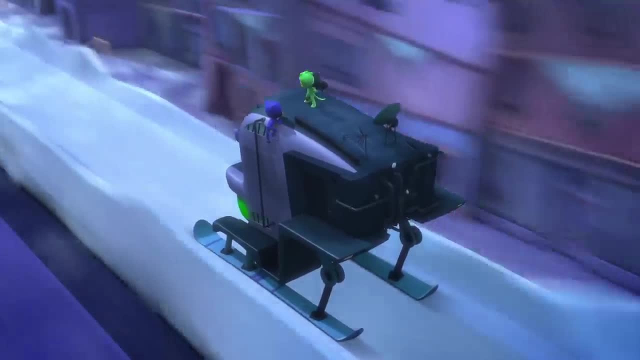 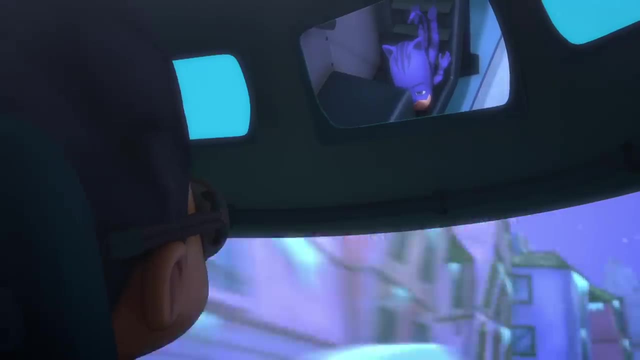 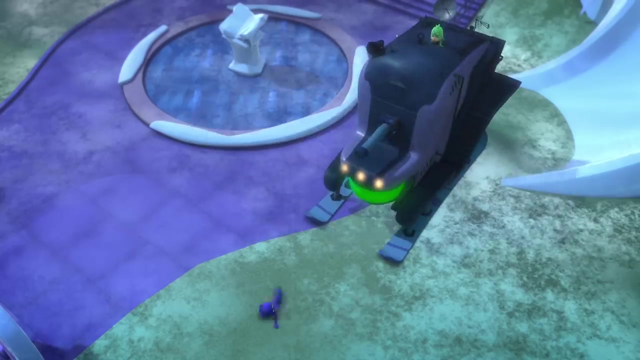 What took you so long? Ooh, Ooh, Ooh, Ooh, Eee-yow, Poor Pussycat. Now get away from my laboggin' Phew. Whoa Catboy, watch out, Uh-oh. 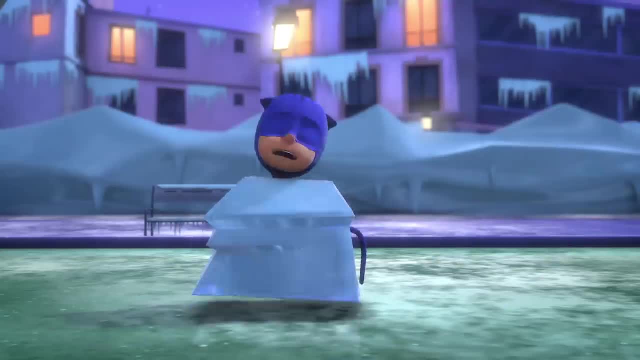 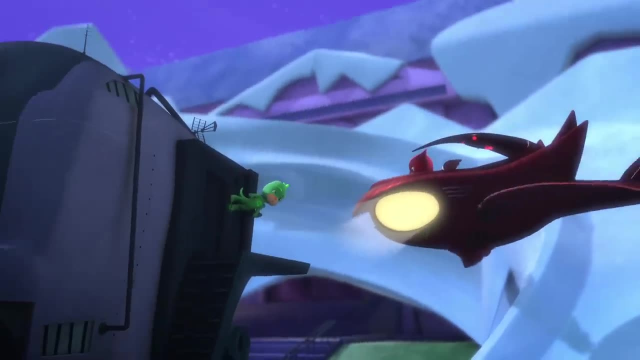 It's c-c-gold. I c-c-can't move. L-Let me out of here, Ro-Romeo Owlette. I think I might be able to stop, Romeo. Look, Not now. Gekko, Come back here. 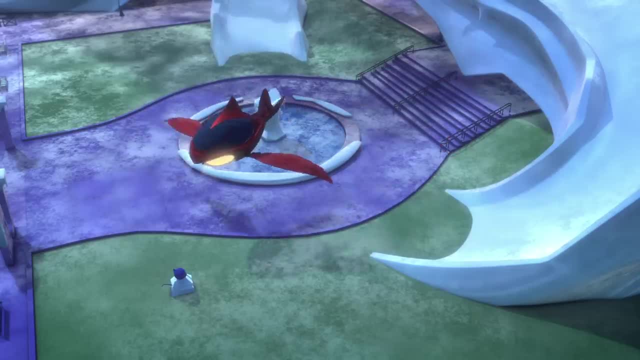 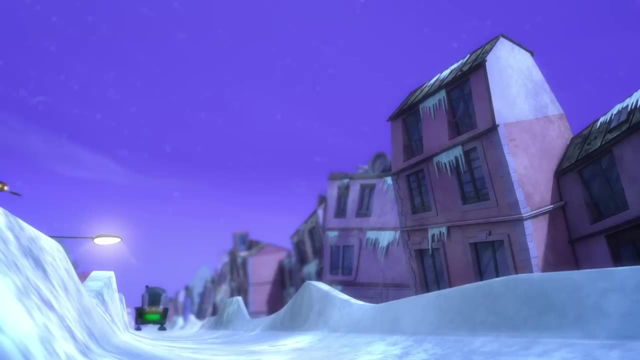 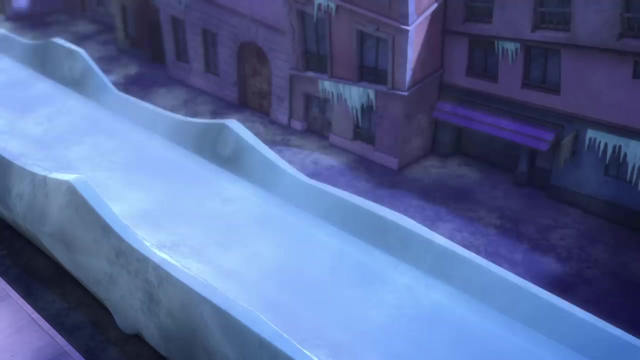 Mwah, Mwah-ha-ha-ha, Catboy. what can we do? Don't worry about me. Romeo's getting away Quick. stop him, Can't keep up with the pace. A-P-J masks. 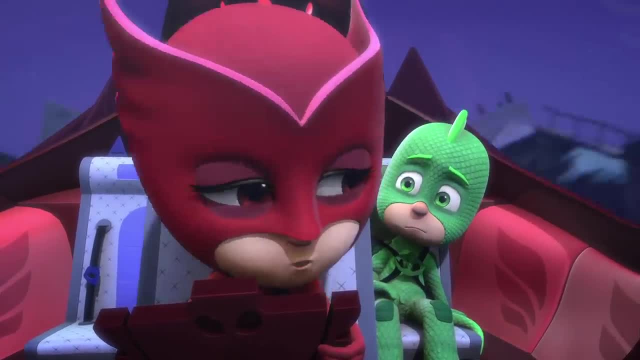 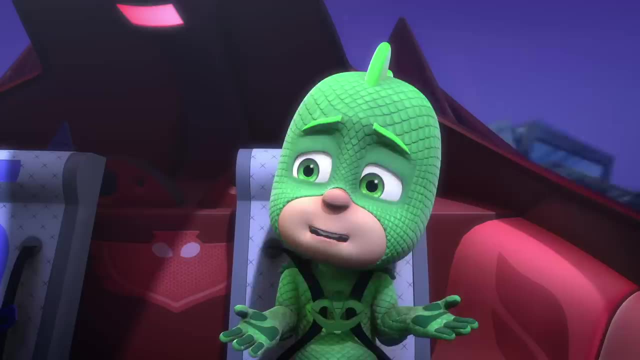 Ooh, we may be superheroes, but right now, Catboy's a super ice block, Ugh Ugh. So the two of us need a plan, Gekko, and fast. That's what I was trying to tell you. 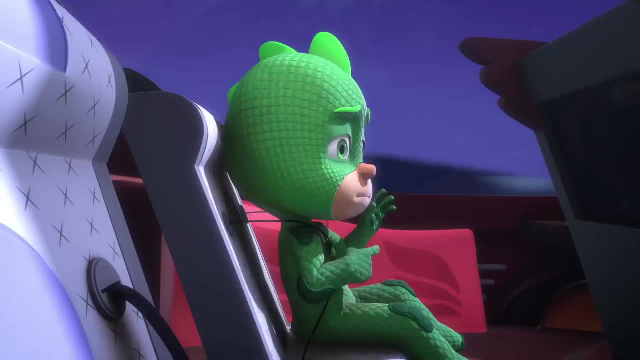 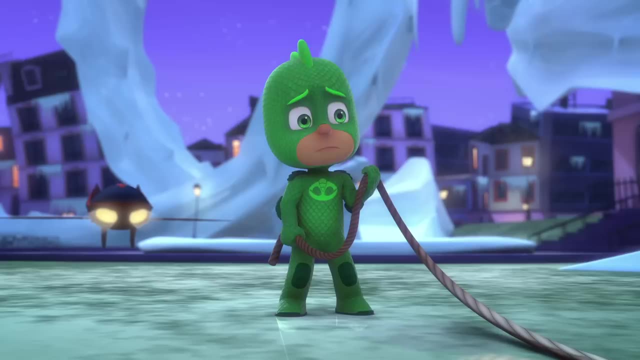 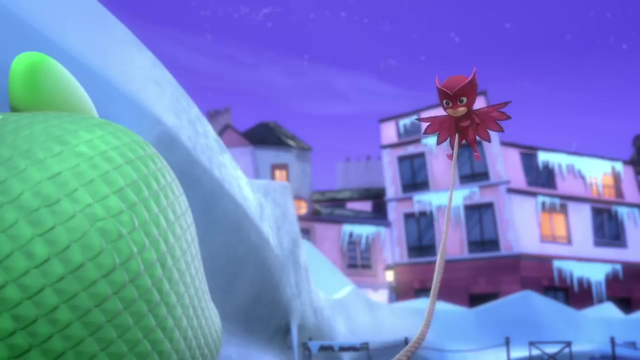 I Hey, I know what we could do, but I'll need your help. But with my plan I could. Okay, what do I do? Ah, Whoa, owl wings. Ah, that's better. Okay, I'll tie this to the lab. 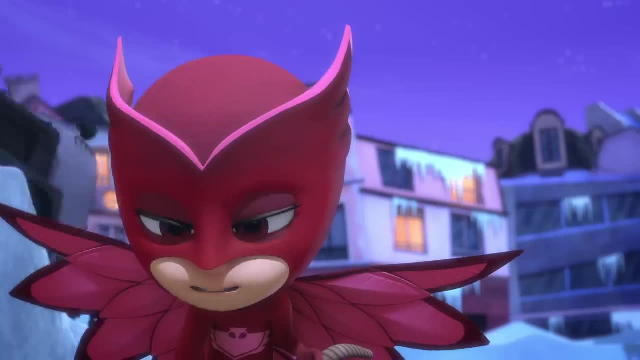 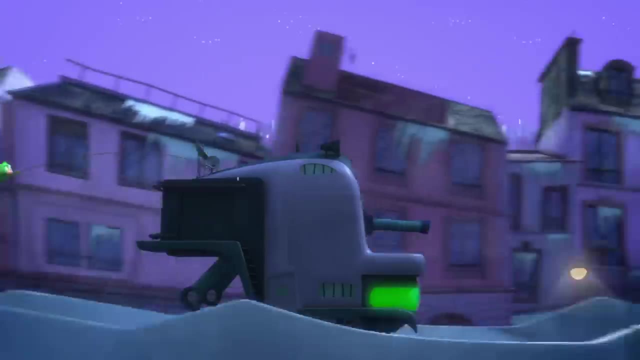 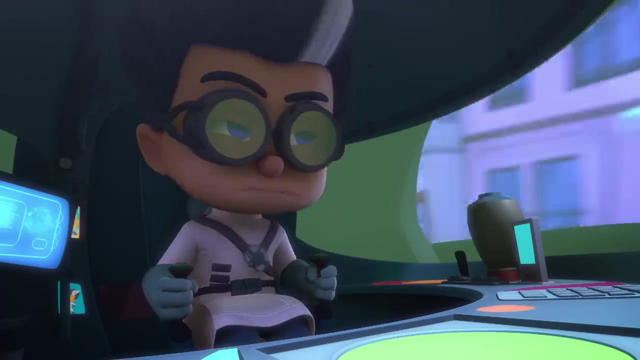 then you use your super strength to stop it moving, Yeah, but Then we take control of the ice machine. Go, Gekko, Wait, Whoa, Whoa Ugh. You think you can outwit a genius like me, Birdbrain. 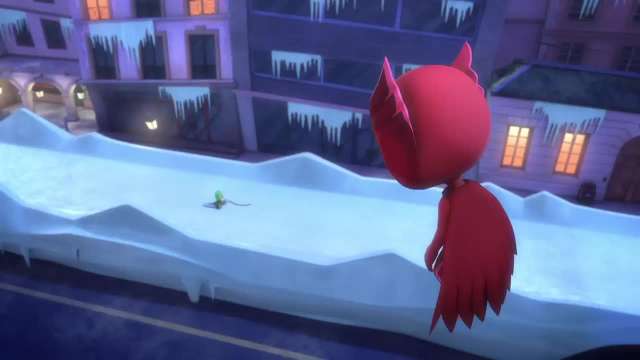 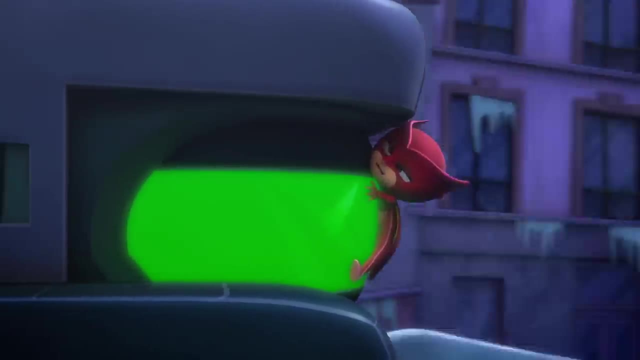 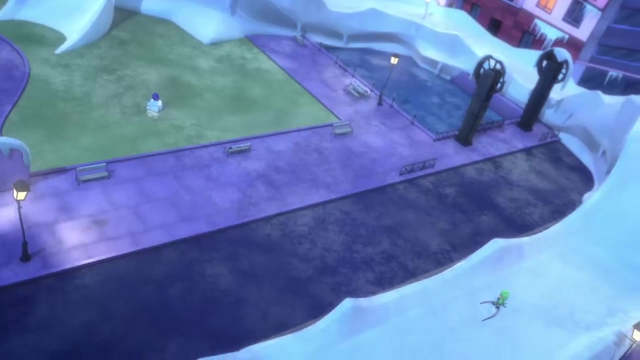 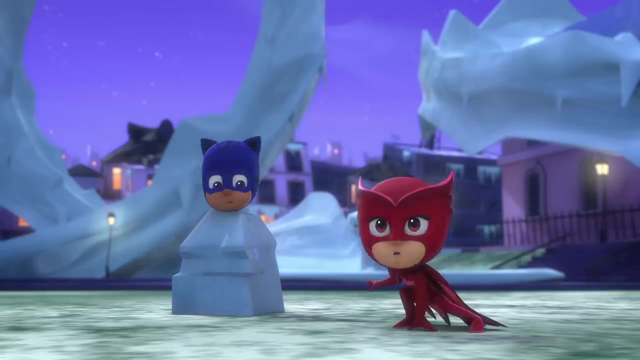 Huh, Ah, Super Owlette muscles. Wait, I don't have super strength. Whoa, Gekko, where are you? Owlette's in trouble, Owlette's in trouble, Oof Ah, Whoa, Uh-oh. 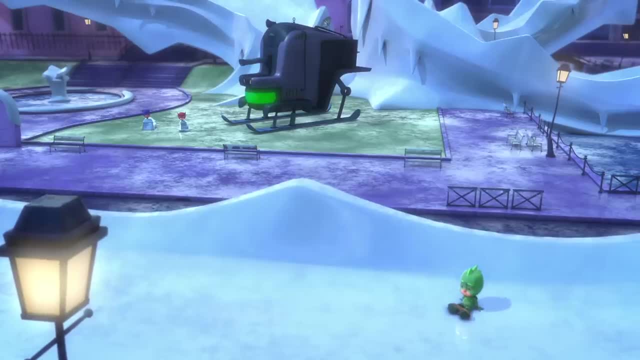 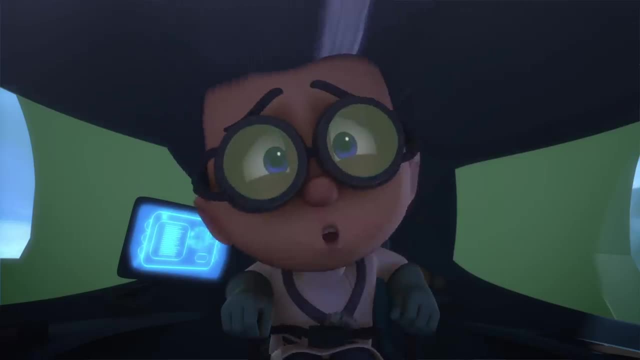 F-f-fluttering, frozen f-f-feathers, Ha-ha-ha-ha-ha. Two little ice blocks lying on the road. Two little ice blocks. oh so very cold. Ha-ha-ha-ha-ha-ha. 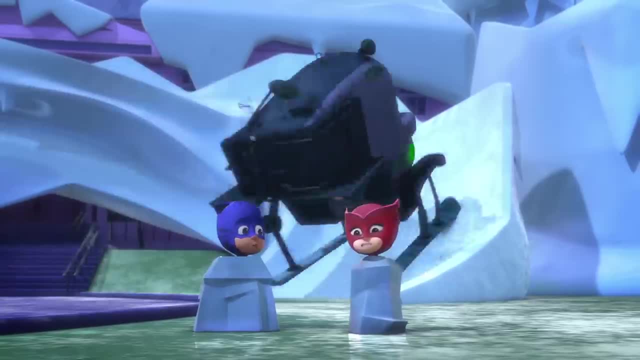 G-g-g-Gekko, I've got a plan, Whee-hee. Wait, I've got a p-p-p-better plan. Slithering serpents, Slithering serpents. Finally. I had stuck up for my own plan. 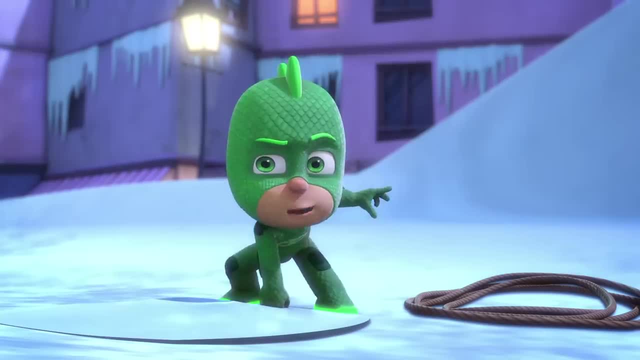 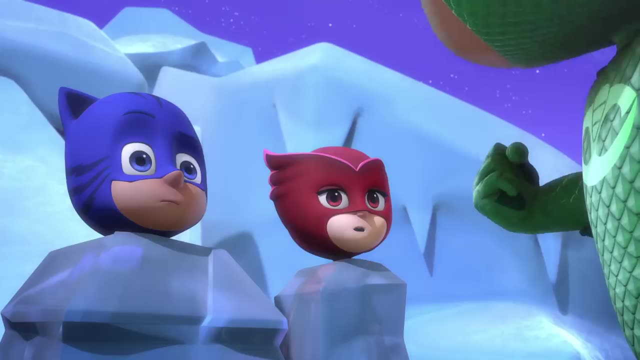 and used my own super power. It's time to be a hero. Super Lizard Grip, It's time for my plan. You can help by smashing as much of Romeo's icy ride as you can, Ready for some ice pinball? Huh. 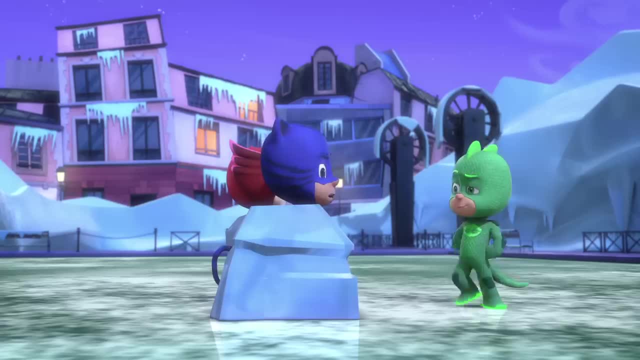 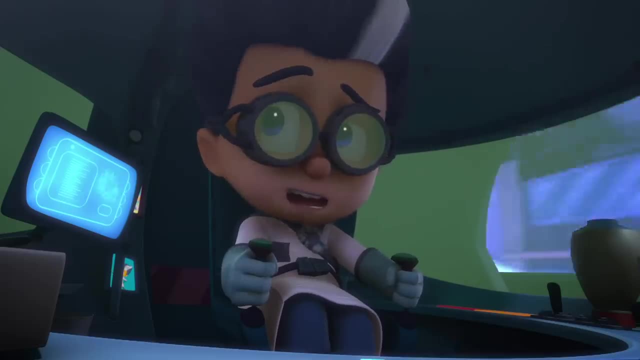 Hey, maybe Gekko's plan could work. Come on, let's smash some ice. Whee-hoo-hoo, Ha-ha-ha-ha-ha, Huh, Those icicle heads are smashing up my beautiful ride. 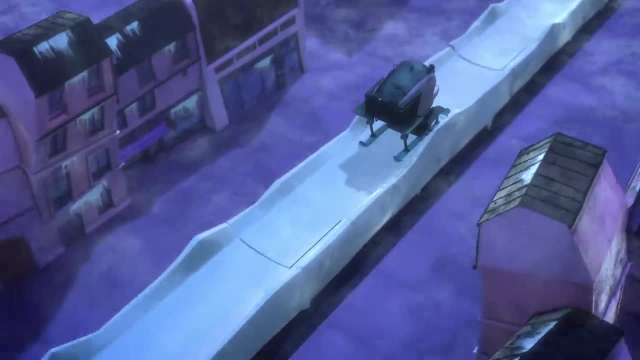 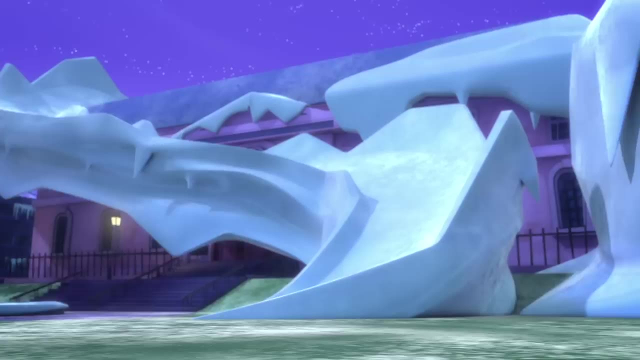 Ha-ha-ha-ha-ha-ha. Now I only have one way to go. Now I'm going to show Romeo how to move on the ice: Super Lizard Grip: Ha, Ha-ha-ha-ha-ha. 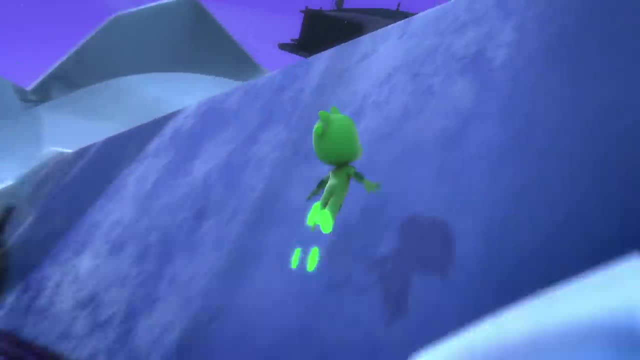 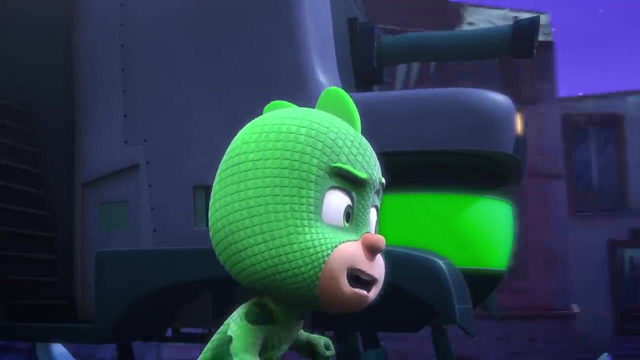 Ha-ha-ha-ha-ha, Ha-ha-ha-ha-ha. Hello Romeo, With my Super Lizard Grip, I'm better on the ice than you. Nonsense, My loboggan was made by a genius, me. 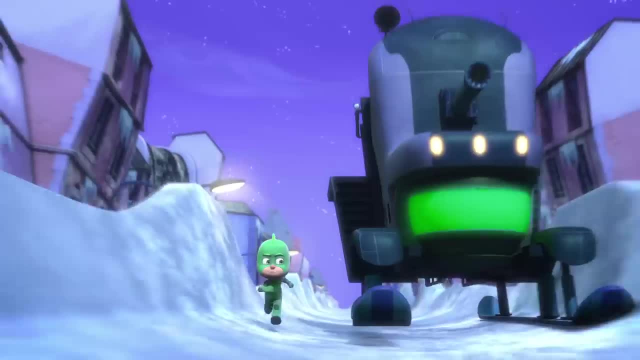 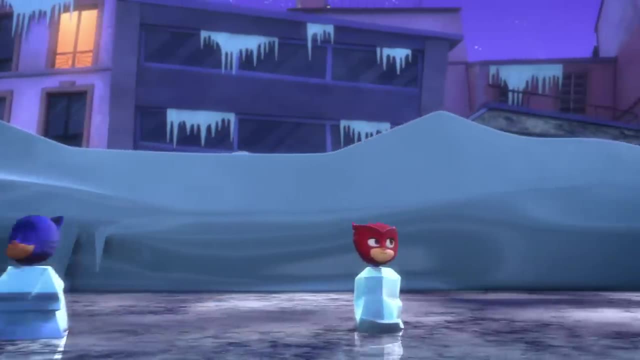 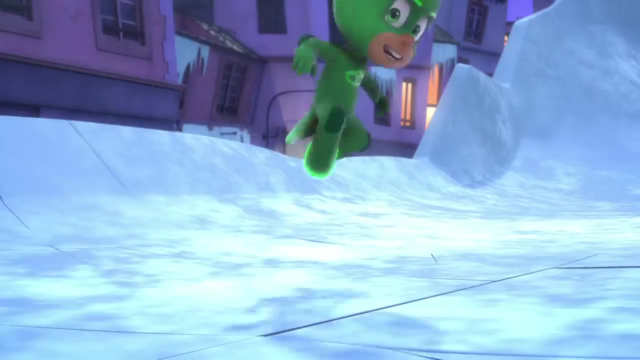 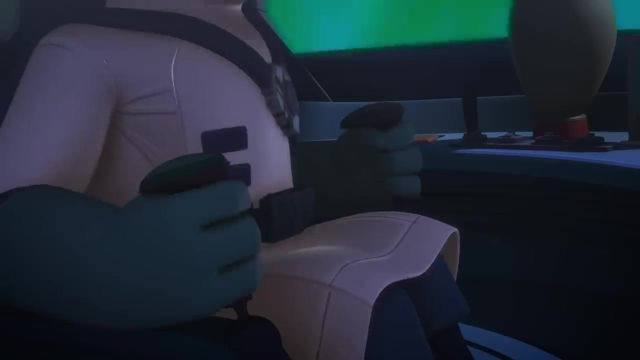 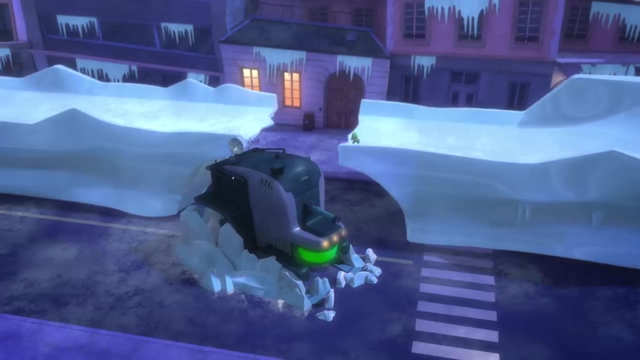 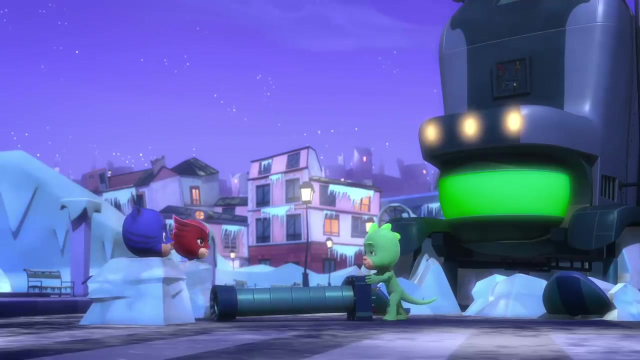 So there's no way one of you mini-minded muttonheads could beat it. Let's see, Go Gekko, Can't catch me. Super Gekko Muscle. Ah, No, Gotcha Romeo. Yeah, Time to get you de-iced PJ Masks. 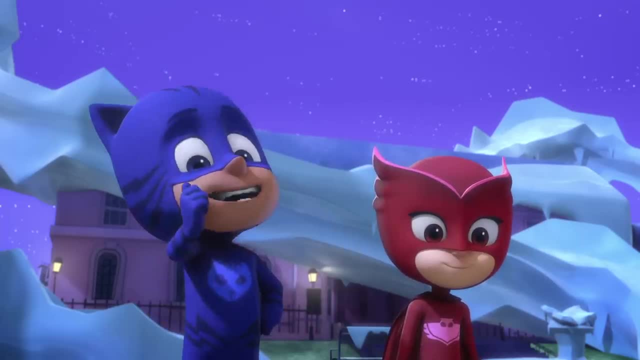 Oh yeah, Nice work, Gekko. That plan was the cat's whiskers. Yeah, we're really sorry we didn't listen to you. No, it's my fault. When I have a good idea, I need to stick up for it. 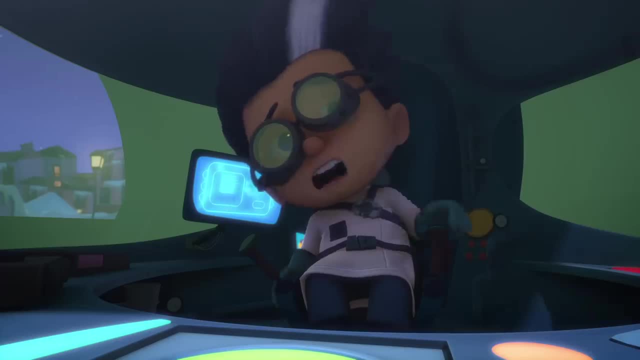 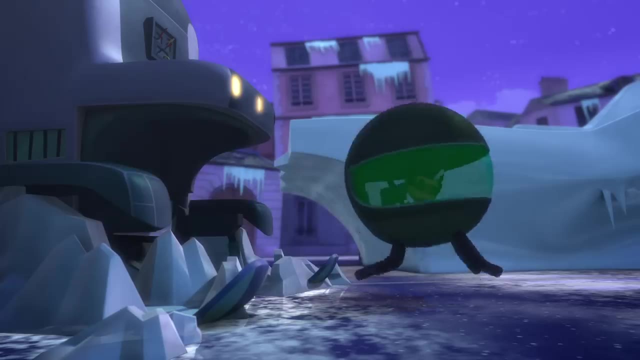 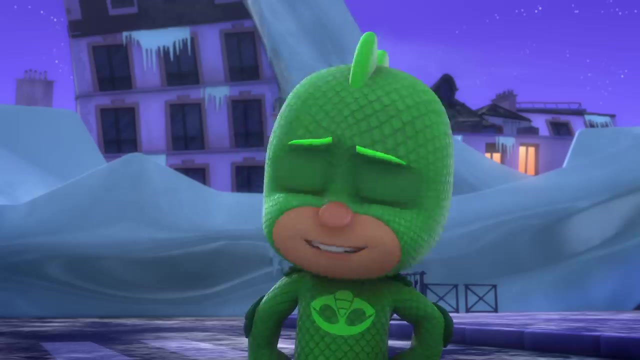 Where are you? Looks like Romeo's really frozen on the spot. You pesky PJ Masks. You always have to spoil my fun. I'll beat you next time, PJ Masks. Well, there's still a lot of ice, But if anyone can multiply morning, we can.